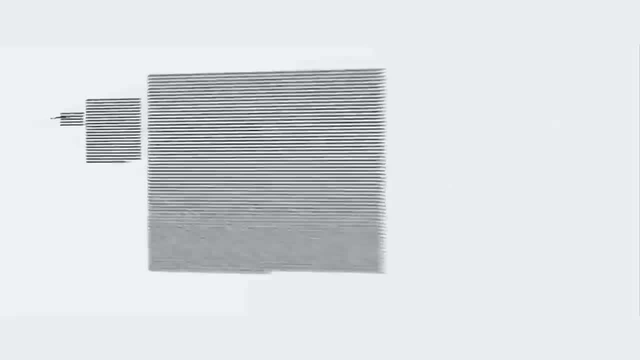 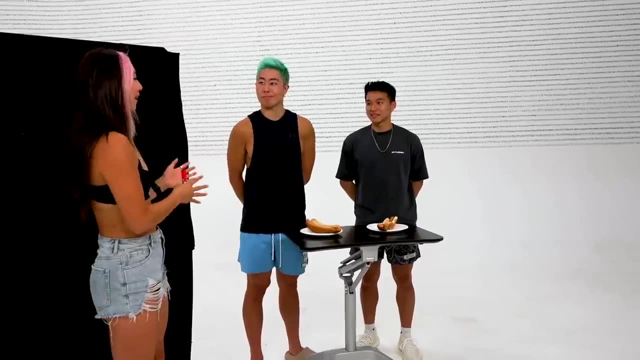 the 100,000 digit math problem. But before I solve that, let's see how I do for the 100 digit math problem. This one is going to be interesting. Behind me is a 100 digit division problem, And if Zach and Ben can finish their hot dogs before I finish my math problem, I have to eat a hot dog. 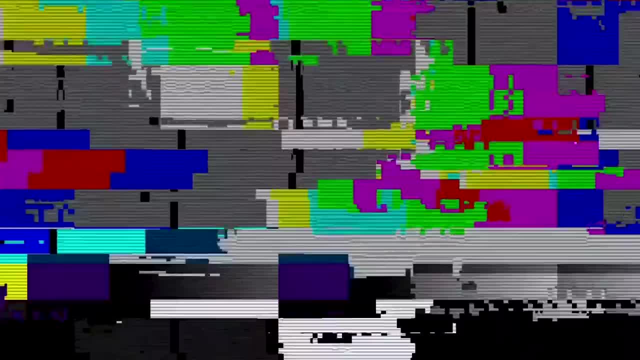 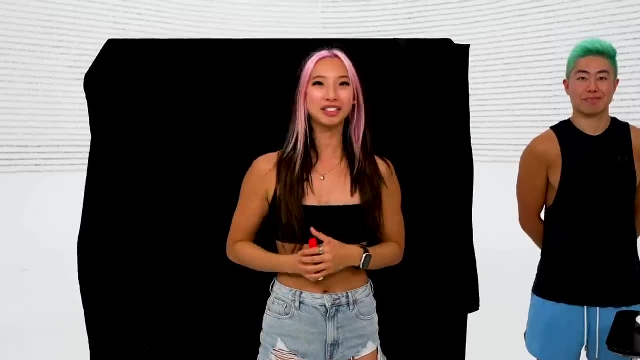 I didn't mean to say hot dog. Let's try the intro again. Behind me is a 100 digit division problem, And if Zach and Ben can finish their hot dogs before I finish my math problem, I have to eat a tarantula. You ready? 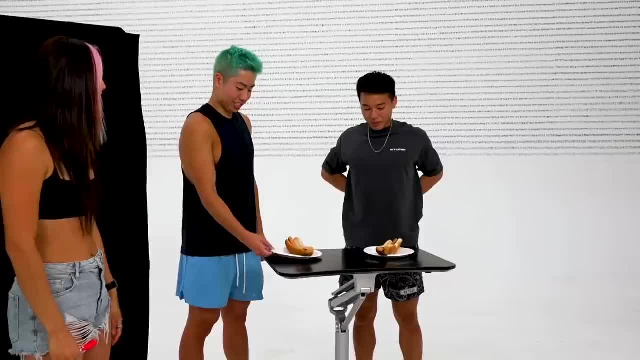 Uh no, I just had lunch. Are you sure you can't finish a hot dog, Bro? this is a lot, Wait. so what happens if we win? You get to see me eat a tarantula. I want more than that. 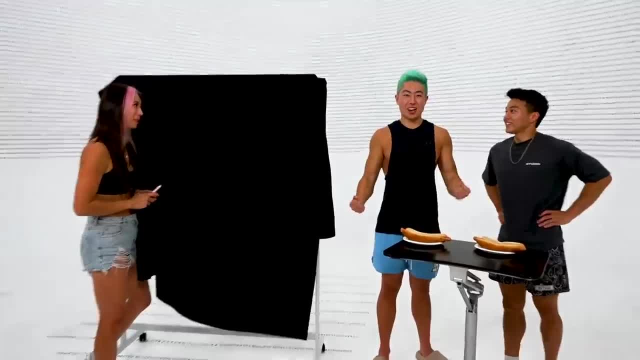 All right, If they win, they also get $500 to split. Let's go. Oh my goodness, Wait. I'm kind of hungry now. I'm hungry now. Wait, Ben, we should touch tips before we start. Three, two, one. 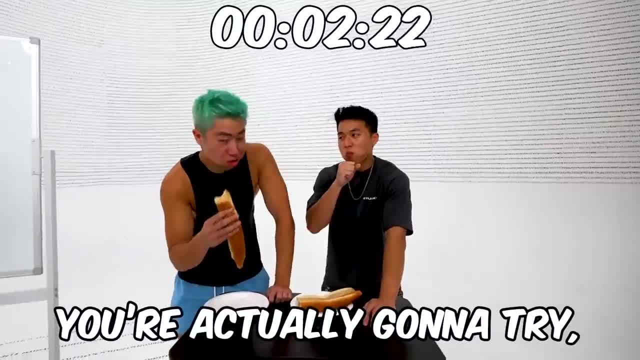 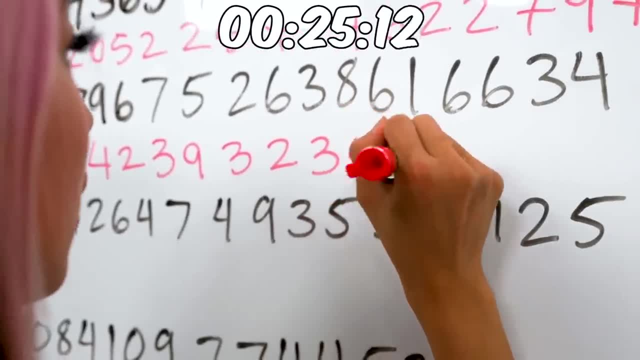 Cheers Go. You're actually going to try right. All right, Nine, seven, eight. Did you guys get water? Did you get a trash can? I'm pretty focused right now, but it seems like Zach and Ben were struggling to eat their hot dogs. 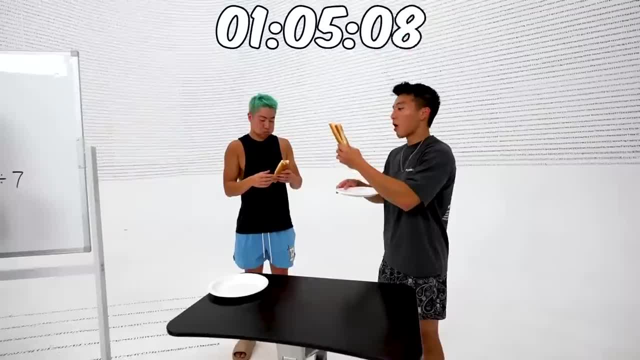 You got it. Come on, You got it. I'm already three rows in and I don't even know if the boys are even halfway done. I'm glad they had lunch before this. We're going to tag team this. Ben, you bite mine, I'll bite yours. 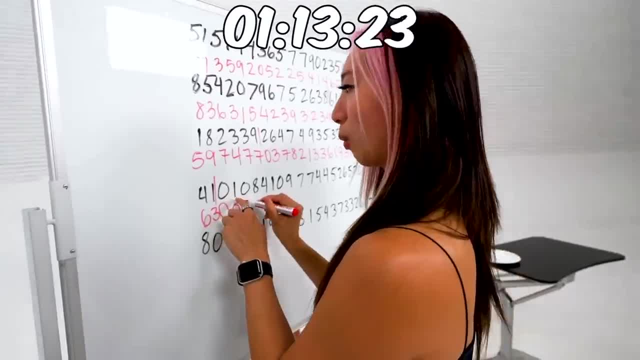 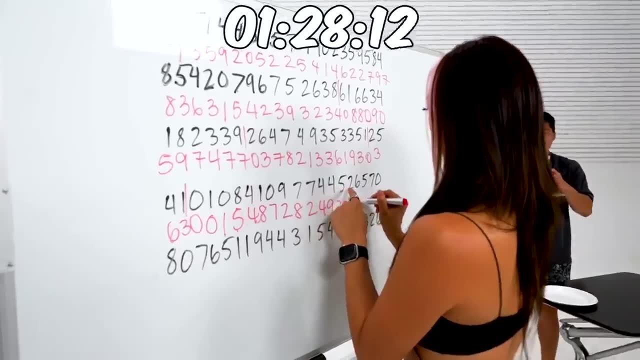 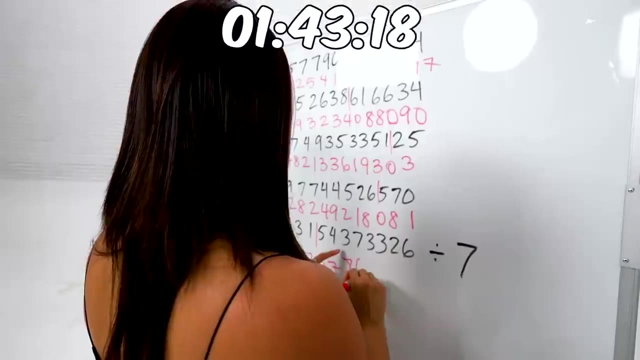 Five, four, three, two, one. You know we're done. Five, four, eight. Wait, just shove it in. Just shove it in Two, one, eight, Zero. one, One, two, three, three, six, seven, six, one, eight. 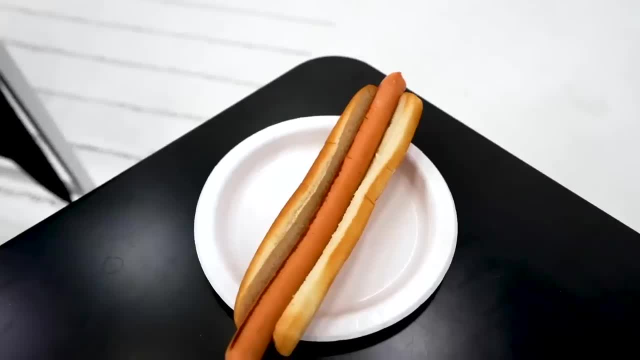 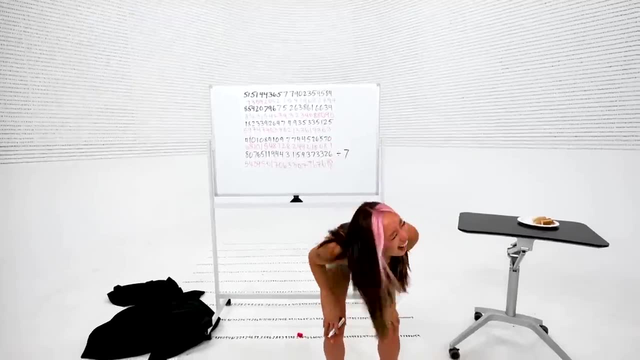 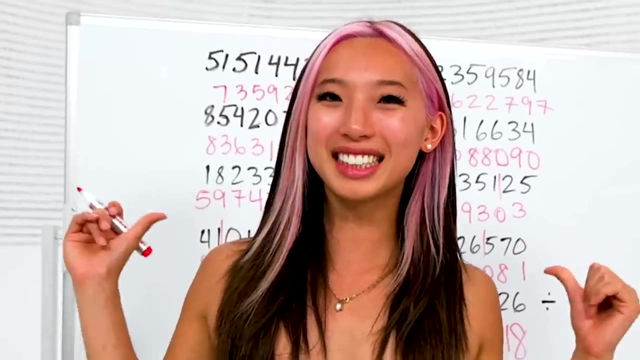 Bro, you just left me hanging. No way You didn't finish a hot dog, Bro, I just spat out the entire freaking hot dog. I think I did it faster than I did last time. I finished this in one minute and 46 seconds. 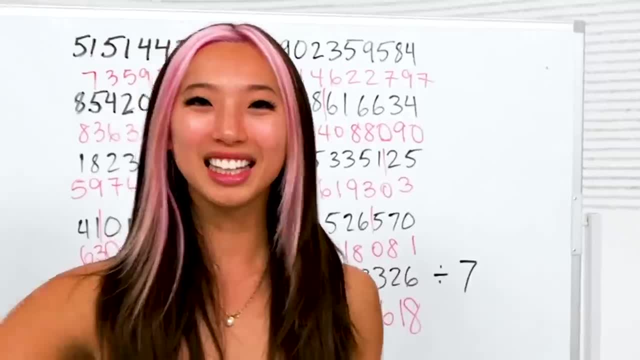 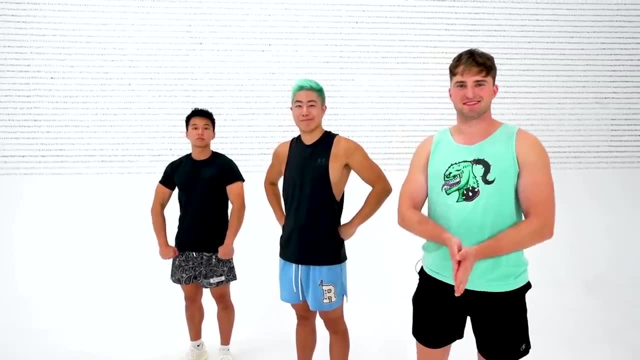 I didn't know I could fit that much of a sausage in my mouth. Well, that was fun. Let's move on to the next one. This is a 1,000-digit math problem. That's a lot of digits If the boys can finish 1,000 push-ups before I finish my math problem. 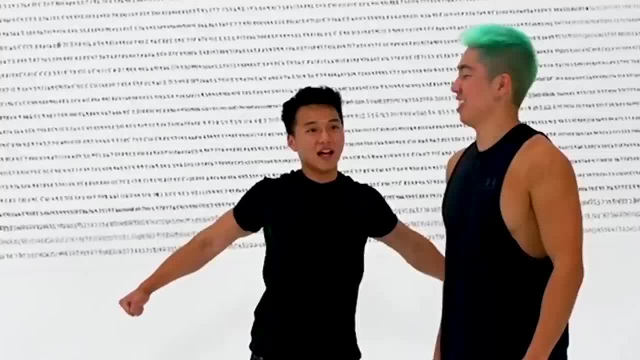 I'll give them $1,000.. Let's go. That's a lot of guap, That's a lot of push-ups, So I really hope I do not lose. All right, we've been doing a lot of chest days recently. 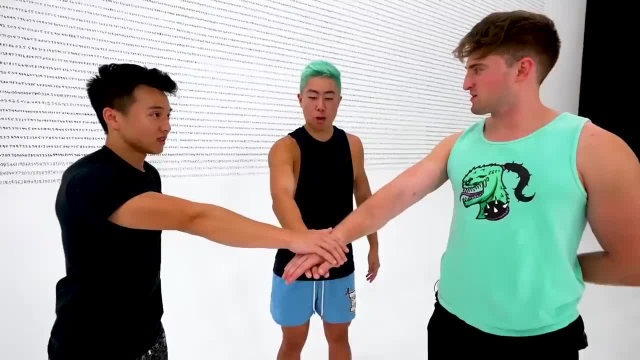 Today's going to be the day we do the most push-ups we've ever done. Come on, bring it in. One, two, three push-ups, All right. Michelle, you've been doing a lot of math problems recently. You got this. 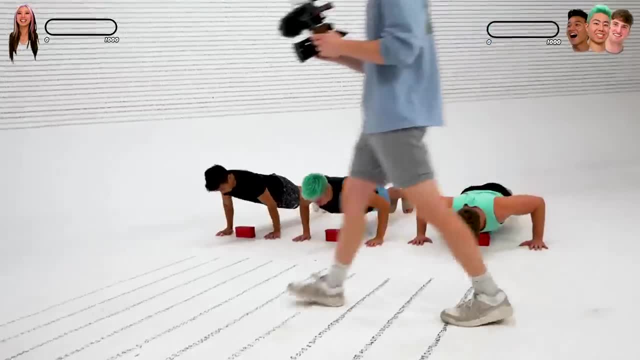 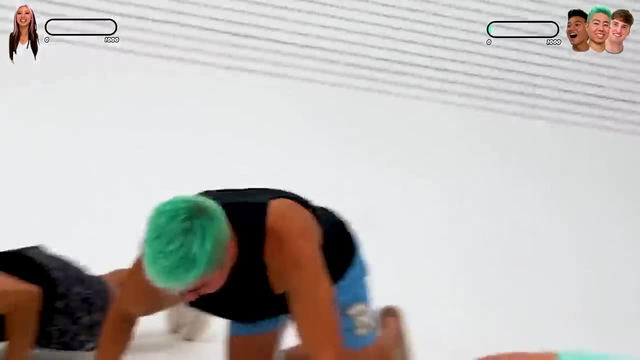 Ready, Yeah, Yeah And go. I'm a little nervous for this challenge, but Because the boys work out every day: Zero, nine, five, four, Oh, it was still. Keep three. divide by seven. One, eight, eight, three. 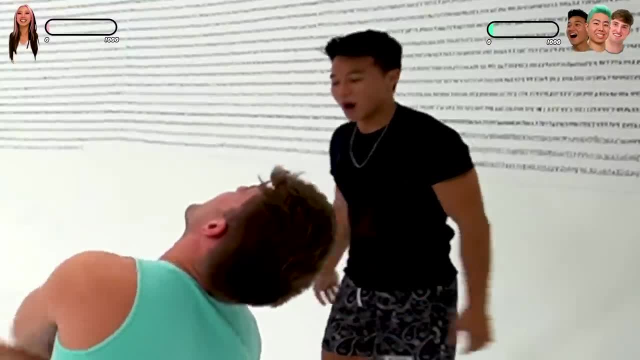 Zero nine: What are you guys at 50.. My chest is too big and my arms are too short. My shoulders are hurting. All right, right, now we're all at 50.. 50?? We've already done 150. 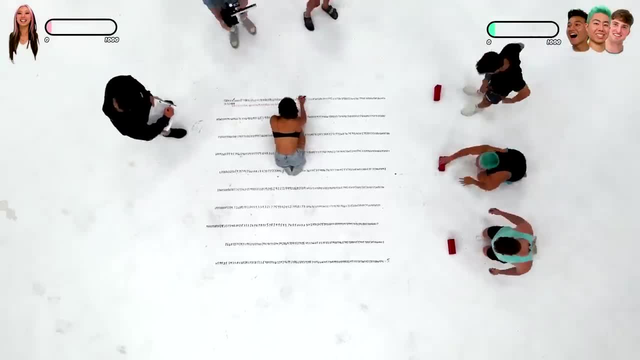 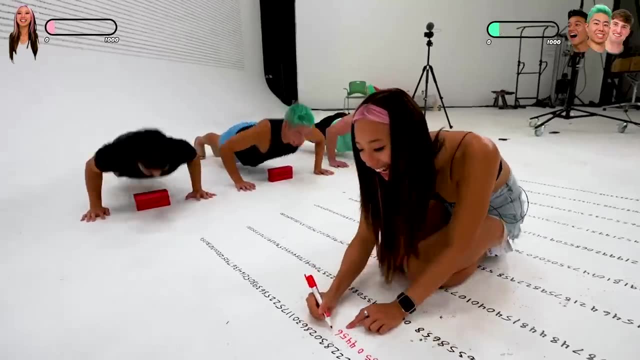 How Knees puppy. And if solving a 1,000-digit problem wasn't hard enough, the boys tried to distract me. You guys are so loud. Three, four, three, four, Stop, Eight, Nine, Okay. 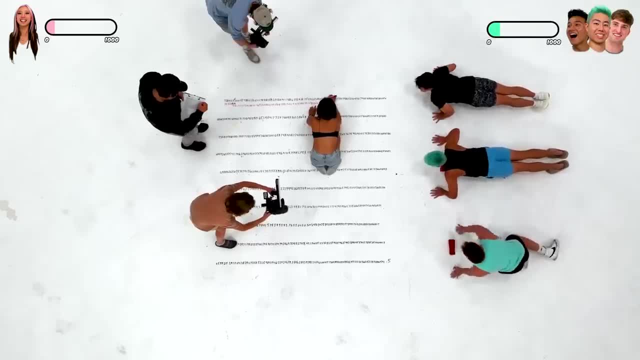 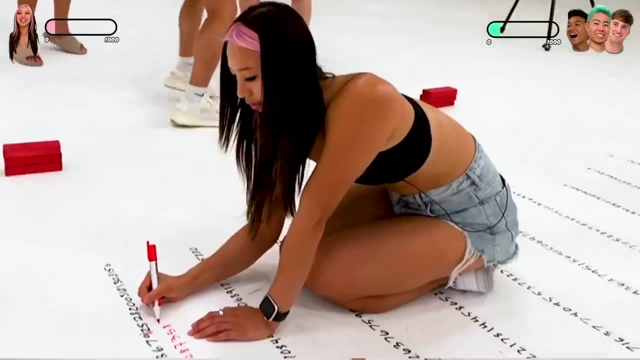 Nine. If anything, they're really just making themselves more tired by yelling 18,. my arms hurt. I'm trying to focus, but the boys look like they're just having fun. Their confidence is definitely making me feel nervous. I don't think I can get the full range of motion with this. 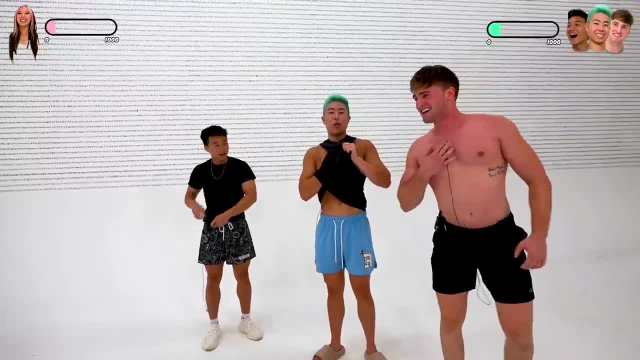 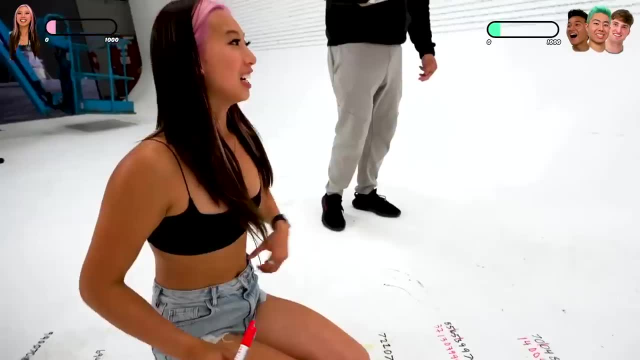 Let me help you. This one's for the boys, For the girls, This one's for the girls. You guys are so weird. Wait, maybe we need to take our pants off. I'm just kidding. I just finished 100.. 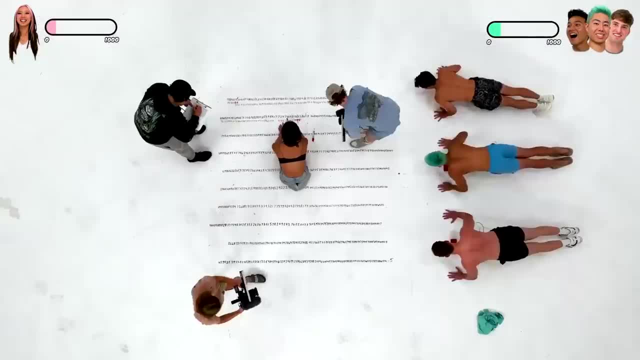 All right, boys ready to knock out 20 together? No, No, All right, let's do 10.. One, Two, Oh crap. I keep making silly mistakes I don't usually make. This challenge is pretty close so far. 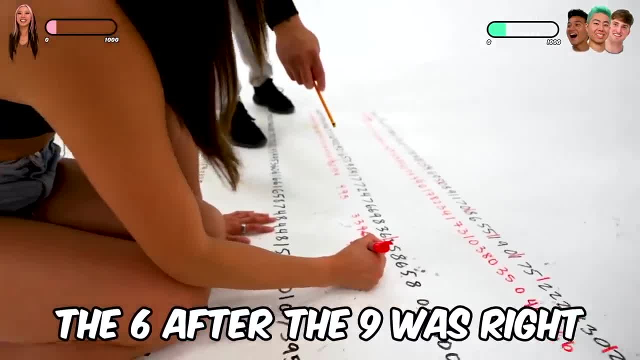 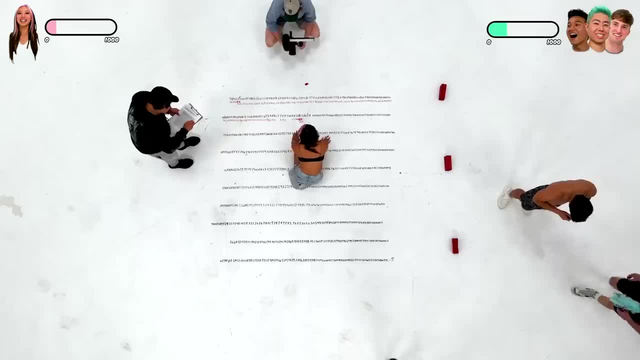 and I'm not doing as well as I thought I would be. I'm not getting six anymore. This is too hard. My chest hurts. She's only one and a half rows down and she's making mistakes right now. My accuracy really needs to be on point if I want to win. 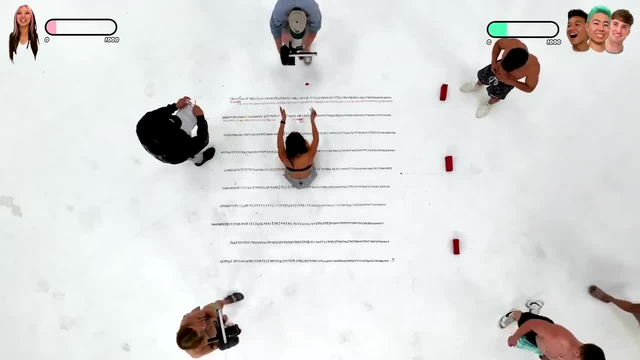 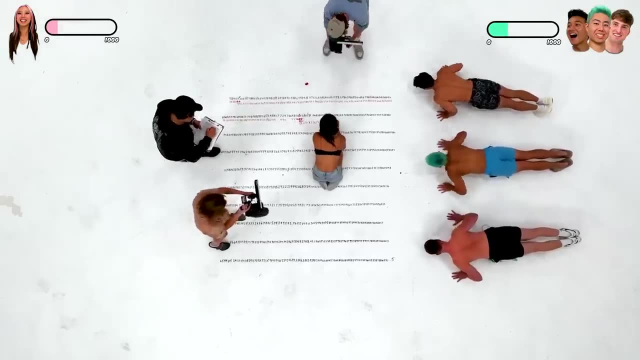 This should be a. Oh, I did divide by six, That's why I'm doing it wrong. Six, seven, two, seven. All right, come on, guys, We need a thousand dollars. For some reason, I kept dividing the problem by the wrong number. 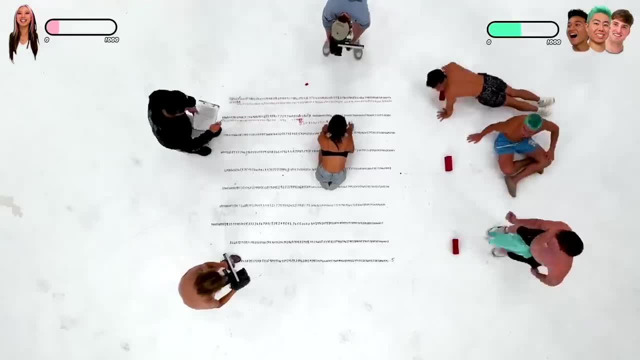 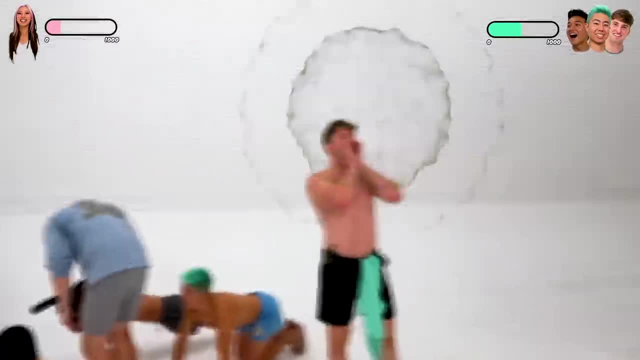 I did divide by six again, Which leads me to keep making mistakes and giving the boys more time to get ahead. We're coming for that 1,000.. Seven, seven, three. Divide by five. Divide by five. Wait, how many are you guys at? 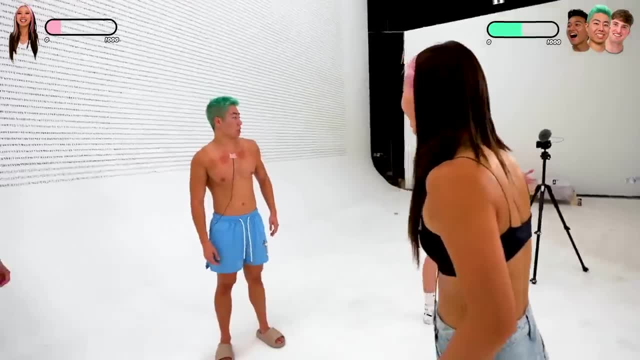 150.. 150. 130.. Wait, you guys are already halfway there. I'm not even halfway done. We're done with 430.. I need to go faster. That means I can take a break. Hey guys, I have an idea to distract Michelle. 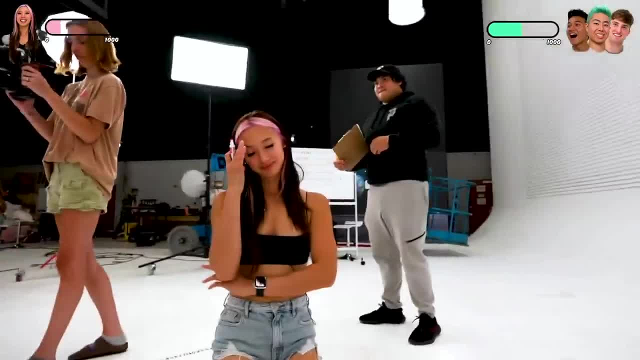 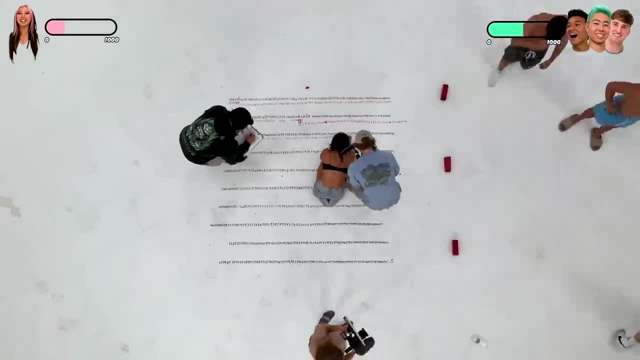 Oh, Michelle, I dropped a block. Zachary, Divide by five. Divide by five, Michelle. I'm not even halfway done yet and the boys are just breezing through the cushions. I refuse to lose the $1,000. 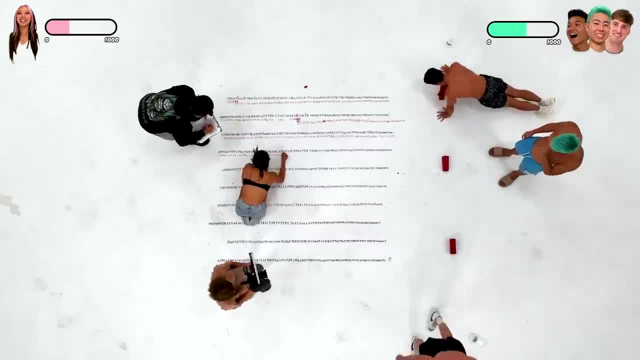 I gotta go faster, Bro. I feel like Ben can do so many because his arms are so short. All right, well, I'm at 200.. I hope they tire out really, really soon. I don't want to give away $1,000. 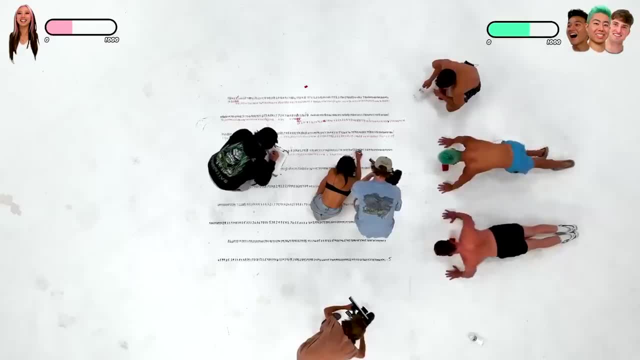 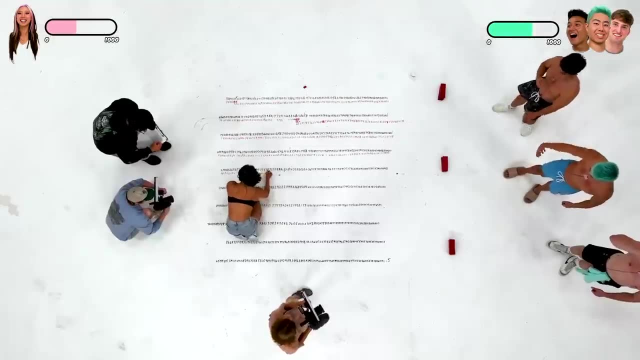 190.. I think that's supposed to be a four right there. No, stop talking, Ben. I think you missed a number. I'm not talking to you. I don't think we need to panic yet. Michelle's not even halfway through. 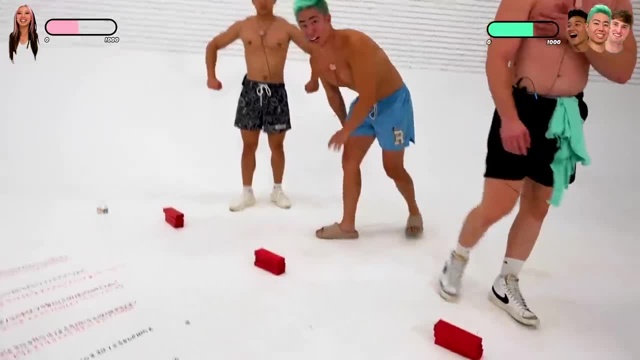 One, three, five, seven, six, seven, three, One, three, five, seven, three. All right, We're all at 200.. 400 left. No, Let's go. Wait, Michelle, how many more do you have? 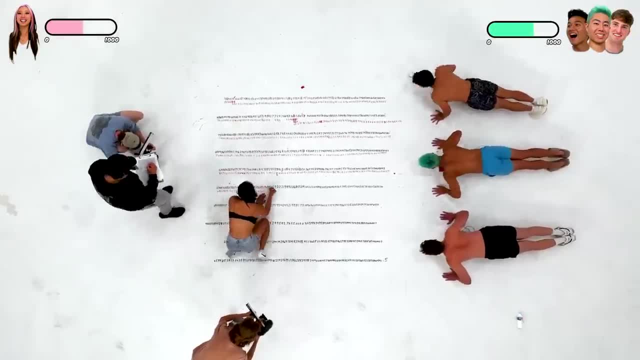 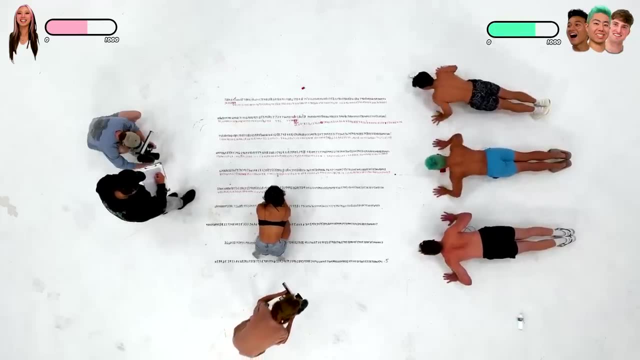 Five more rows, Let's knock out 20.. One, two, three, six, seven, eight. Oh, I'm tired, Dude, come on, I'm holding it. 11,, 12,, 13,, 17,, 18,, 19,, 20.. 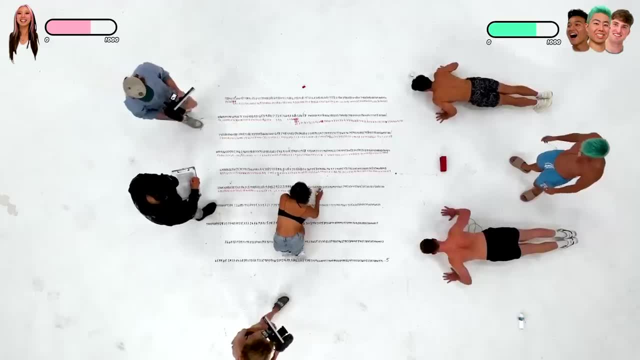 All right, 20 more. No, no, no, no, no, no, no, I got 10 more. I think One, two, Even though the boys were ahead, they started to slow down a bit because they started to take breaks. 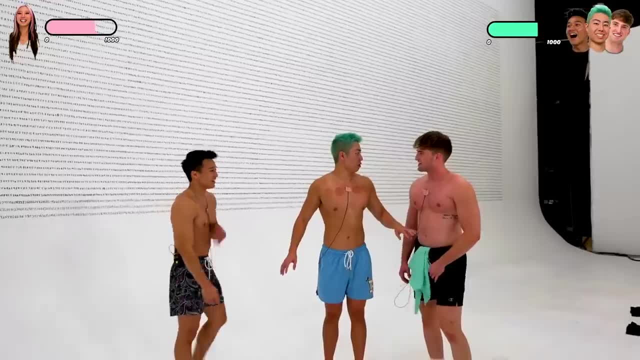 One, seven, three, three, three, four, four, five, zero, zero, seven, eight, Jake, stop Nine, nine, Let her cook. No, we can't. Oh my gosh, My time to catch up. 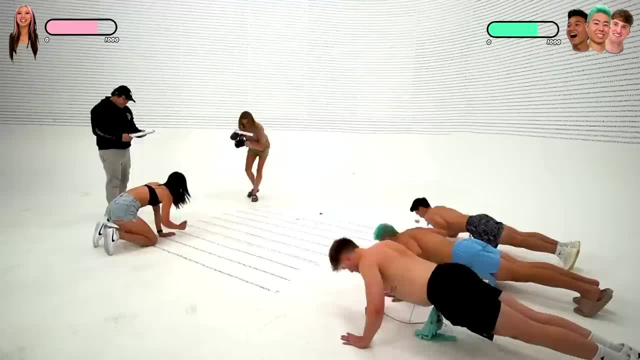 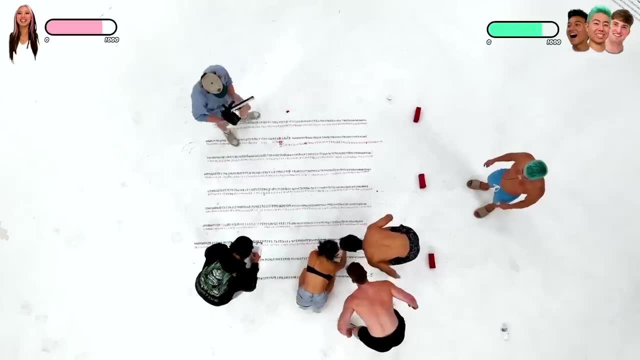 Michelle, what are you at? We're at 690.. I'm 300 left. Wait, she's ahead of us. One, two, six, seven, eight, nine, ten. I need a short break, All right? Hey, no, Matt, no. 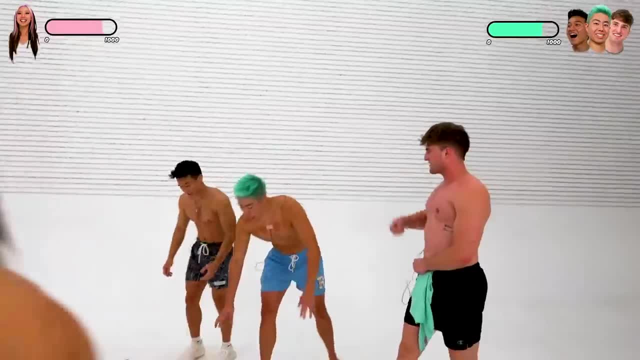 Wait, what are we at 750?? What are you at, Michelle? I'm at 800.. Guys, we need to pump it out. One, two, three, four, five, six, seven, eight, nine, ten. 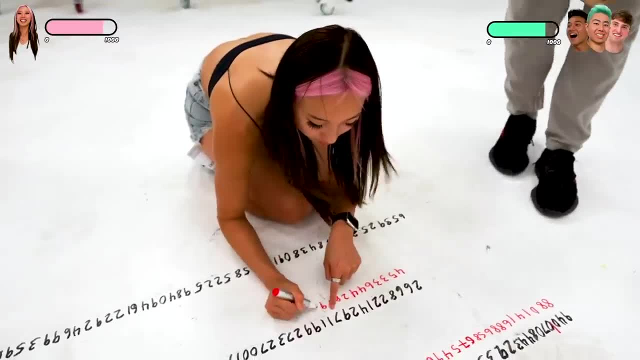 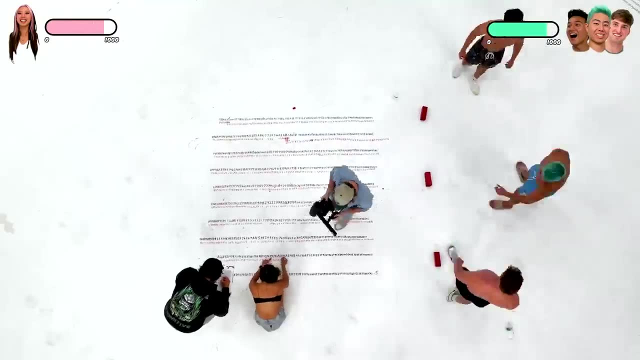 I can't get my money away. 30,, 40,, 40,, 80,, 30.. Oh, I'm about to pass out, Zach. she has one more line, Ben, we have to carry. I'm feeling pretty good. 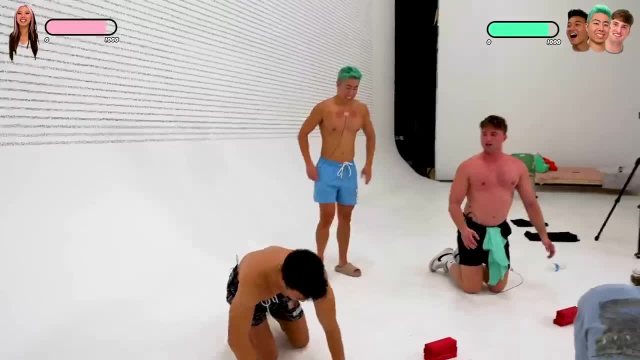 Our boys are getting tired. I'm not making that many mistakes- 300.. You guys got to wait for me to catch up. We have no time, Do 10.. I'll do 10.. OK, Hold me up, Jake. 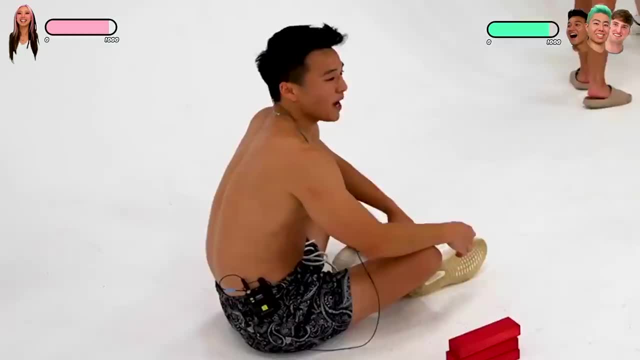 All right, Zach's at 300.. Oh, last row, last row, last row. Wait guys, When she gets in the middle. we just got to crank it out, Michelle, we're at 300 each. I think I have 50 left. 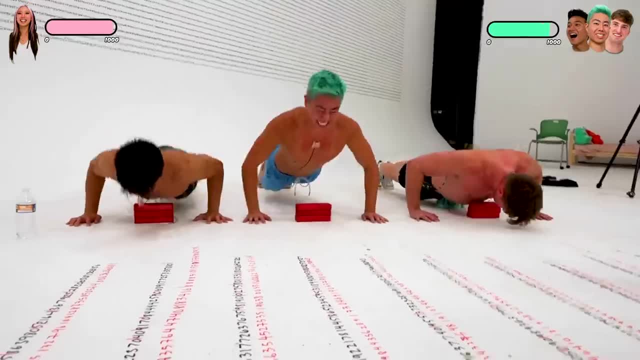 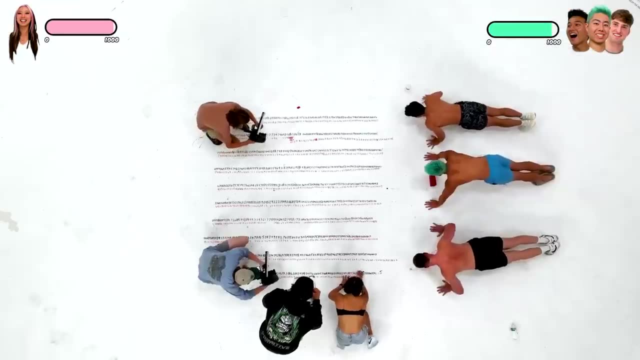 Last 100.. Oh, It's really coming down to the wire, and making one small mistake might be the difference between winning and losing 20.. No, Come on, come on, come on, Ah, 16.. 16.. 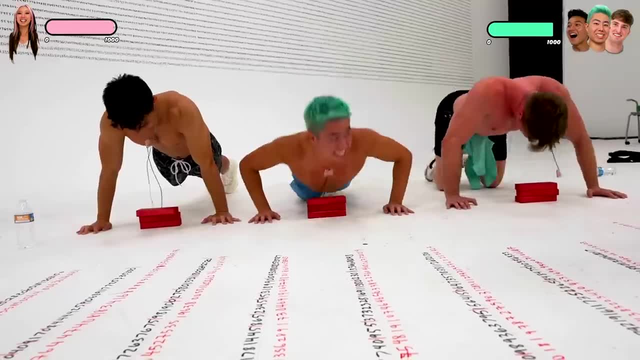 17. No, No, No, No, 33. No, No, No, No, No, 33. 33. No, No, No. Oh wait, She's not finished. I didn't hear you. 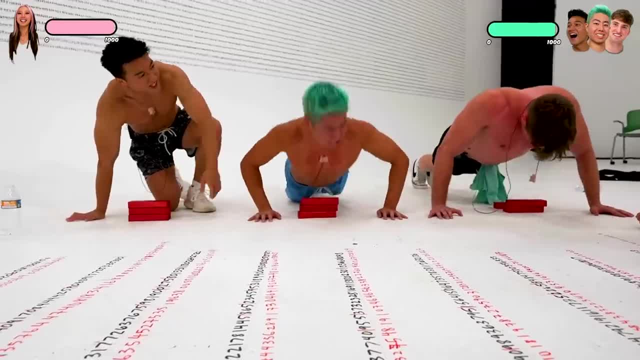 30. 30., 29. 30. 30. 30. Come on Zach. 30. 30. 10. 30. 30. 30. 30. No, No, No, No. 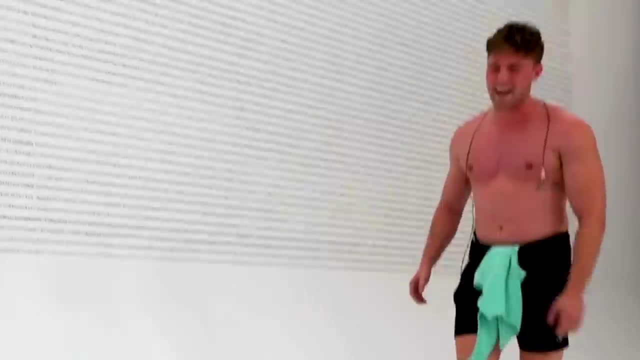 Zach, Wait, how many did you do? 33.. 333.. I did 33.. You were supposed to do an extra. What I thought you were supposed to do it. I thought you were going to do the extra. I finished it for you. 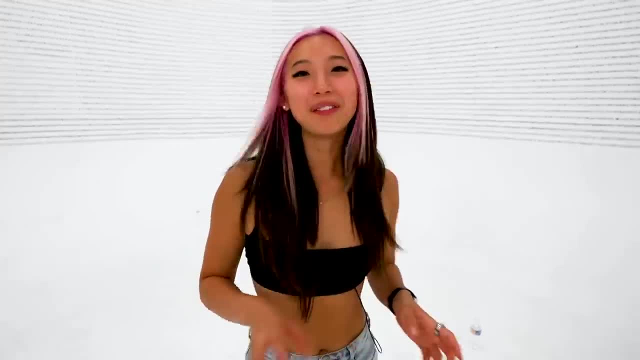 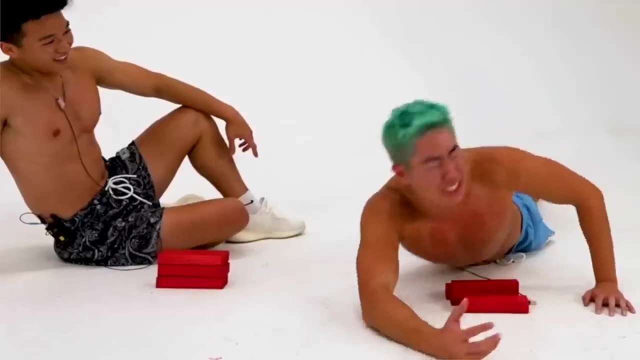 No way. They only did 999.. I can't believe the boys missed out on $1,000 because of lack of communication. They each said that they had to do 333 push-ups and one person had to do 334, but nobody did it at the end. 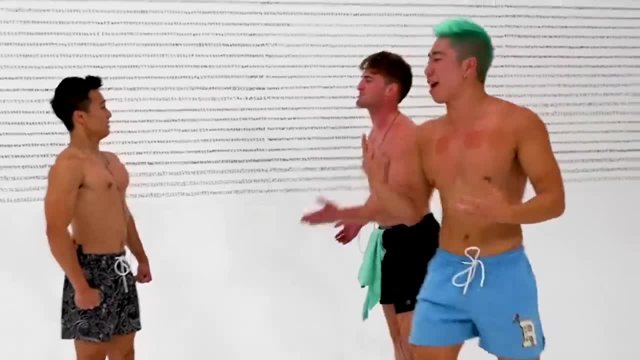 Ben, we can establish this. You said you have the shortest arm, You'll do the extra. I don't think the boys can do math. At least I won Ben. why would I be doing the 334? Because you said you were him. 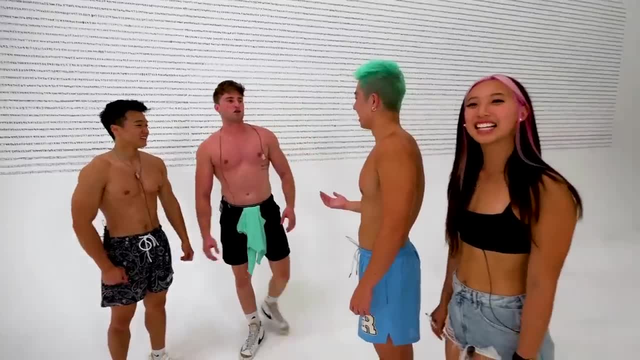 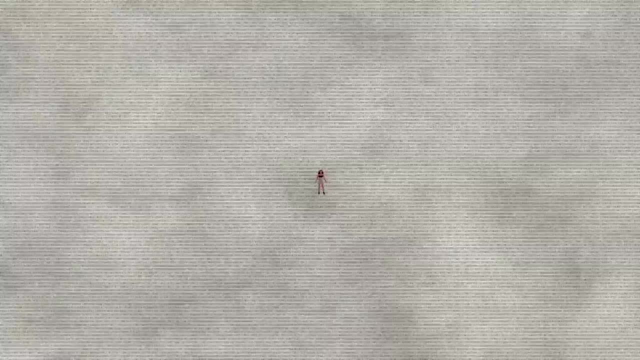 Wait a second. we said you were him. I never said that You guys did 999 push-ups for nothing. No, we did it for a sick pump. And now the moment you've all been waiting for, the 100,000 digit math problem. 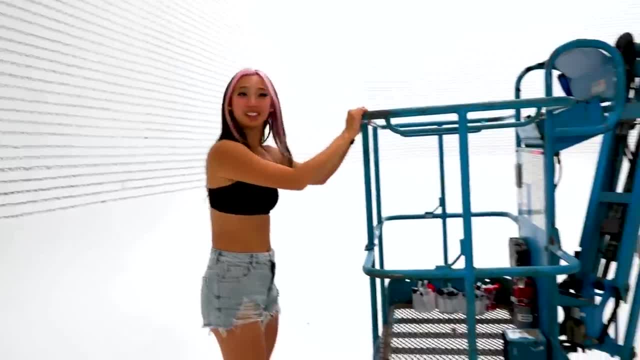 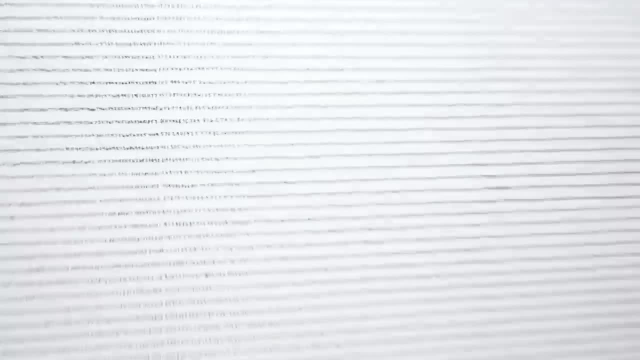 This problem is literally so big I have to use this lift to start the problem. Come, come, come. All right, let's go up. My phone number is hidden in this math problem. Let me know if you can find it. 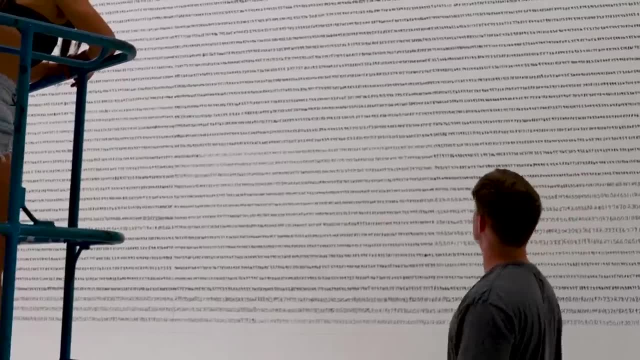 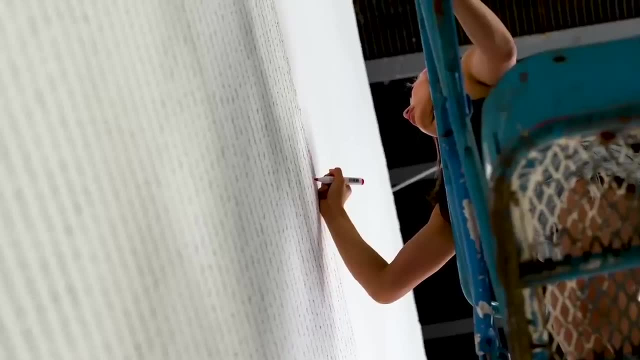 This is going to take me forever. Holy crap, Michelle. how long did this even take to write Over 100 hours? Oh my God, On top of solving the 100,000 digit math problem, if I don't finish, for whatever reason, in 10 days, 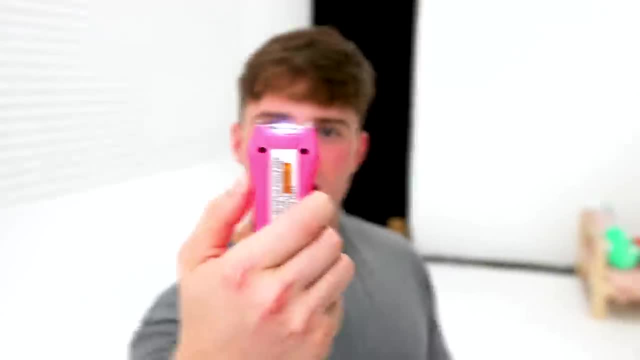 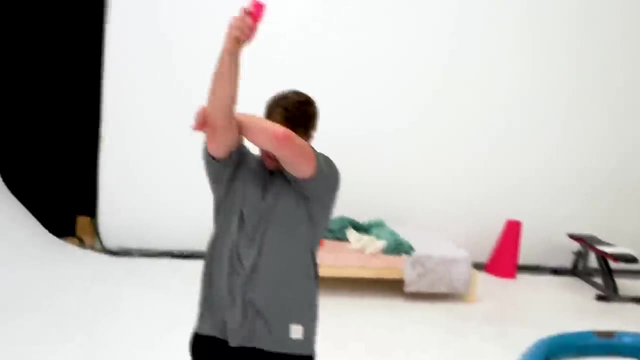 I have to get tasered. Look how insane this is. Oh my God, That's so scary. No way I have to finish. Oh my God, Put that away. Put that away. Wait. look, It says 420.. 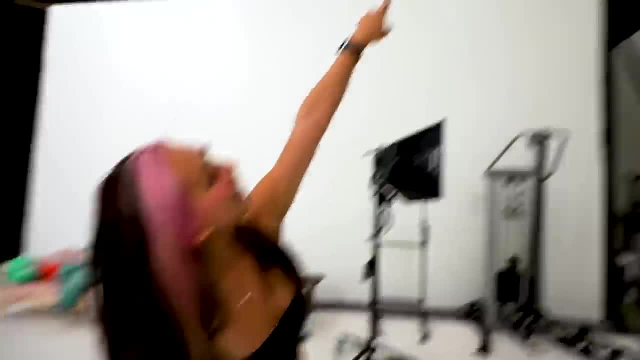 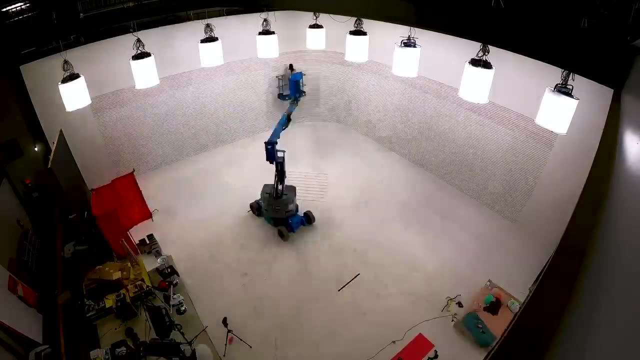 Do you see it? And I have a GoPro up there that's running time to prove that I will be working nonstop on this problem for 10 days. And since I'm going to be here for 10 days, I have a bed and a gym and these cute ZC plushies. 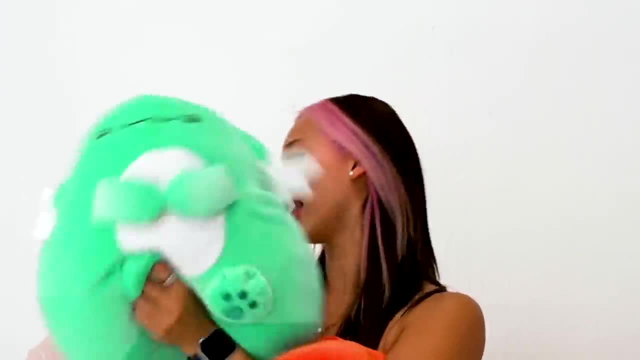 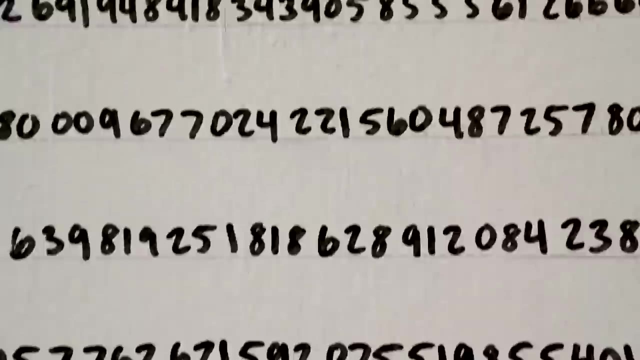 which you can get at zcstorecom. Yay, math. So excited I feel like I'm going to have a mental breakdown, maybe three times in this video. All right, Jake, you can decide what number this 100,000 digit math problem will be divided by. 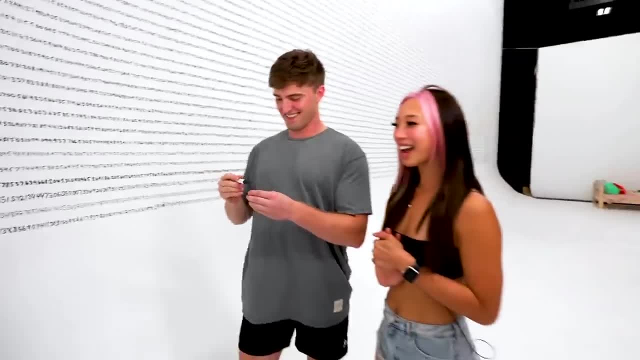 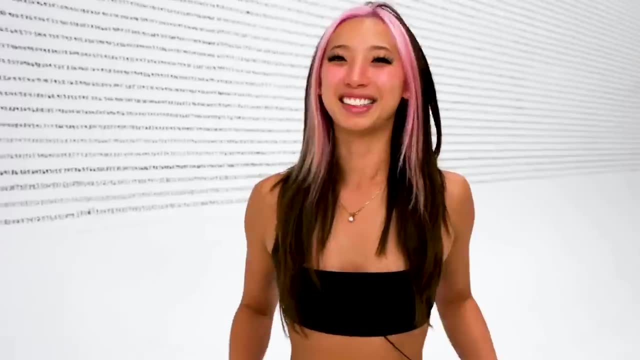 Why don't we do eight? OK, I'm so excited. This is going to be so hard. Honestly, if I was her, I wouldn't be quite as excited, But she loves math. I do love math. Last time I solved a 10,000 digit math problem. 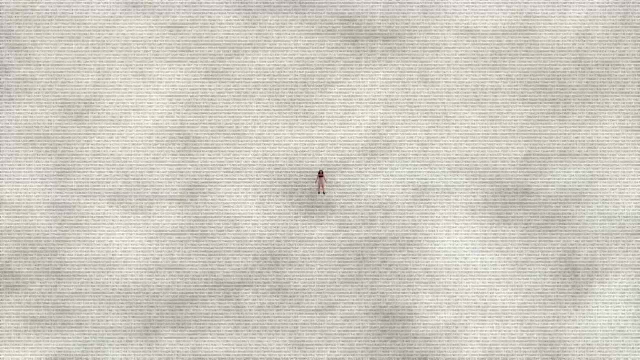 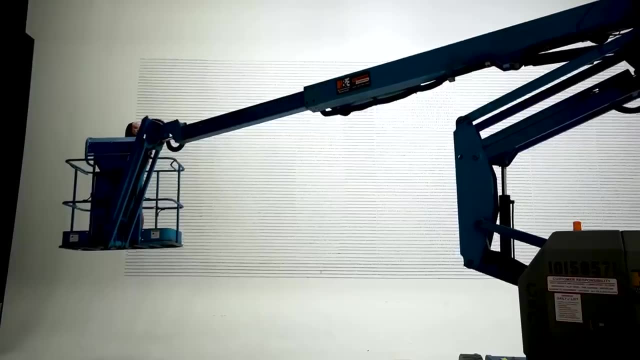 and it took me 8 and 1 half hours. So while I do the 100,000 digit math problem, I'm also going to see how fast I can solve the first 10,000 digits. Let's get started And we're going up. Time to officially start with the first digit: 2, 3,, 4,, 5,, 9,, 10.. 10 digits done: 0,, 2,, 1., 0., 4. 4.. 50 digits done. 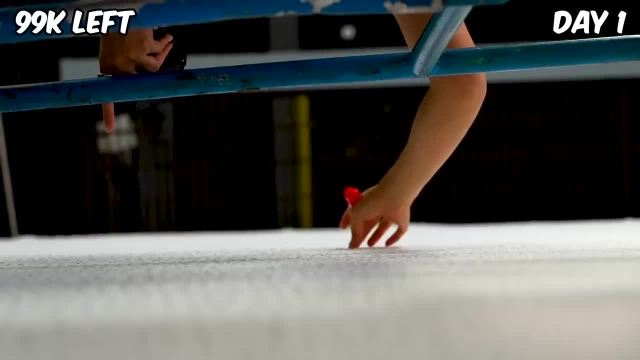 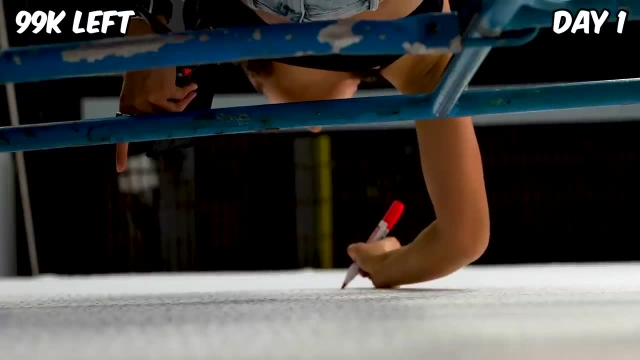 Only 99,950 more to go. Even though this problem is so long, I want to try to make as few mistakes as possible, But I already know I'm due to make some 0, 6.. And, sure enough, 6, 5.. 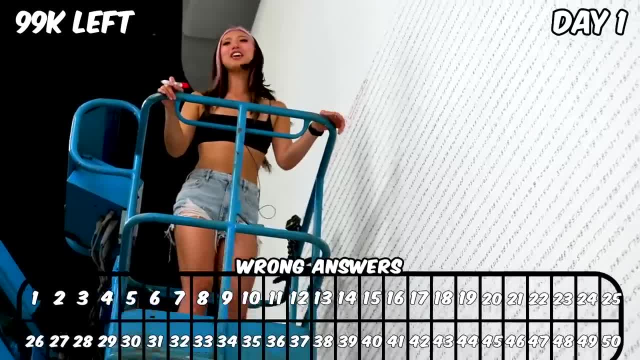 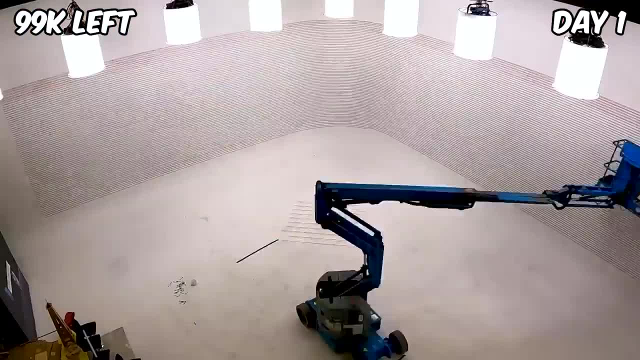 Michelle, stop, I'm pretty sure you got a digit wrong. No, I wrote a 5 instead of a 3.. If getting tasered for not finishing wasn't enough, if I get 50 digits incorrect, I have to restart the entire problem. 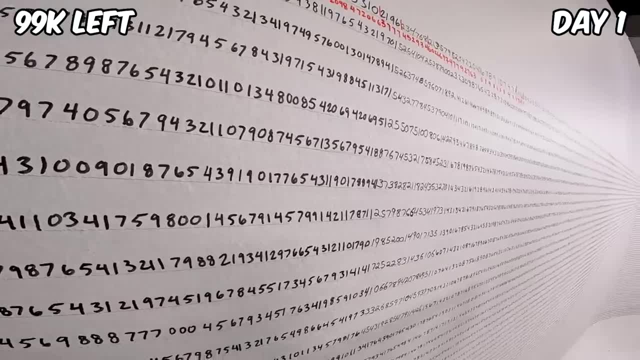 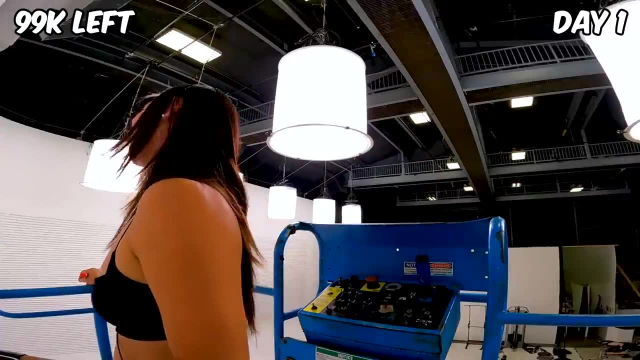 All right Time to move it over. I'm so scared. This is not easy to control. 1,, 2, 8.. Oh man, I got another digit wrong And I'm at 300 digits. This is not looking so good for me. 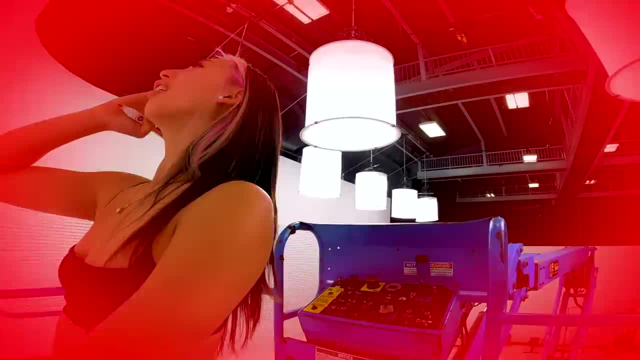 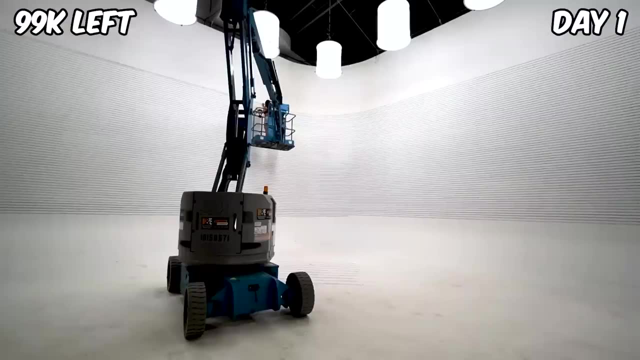 0, 8,, 3, 2.. Oh, 4, 3, 2.. 4, 3, 2.. It hasn't even been 500 digits and I've already made three mistakes. Hopefully I don't make any more anytime soon. 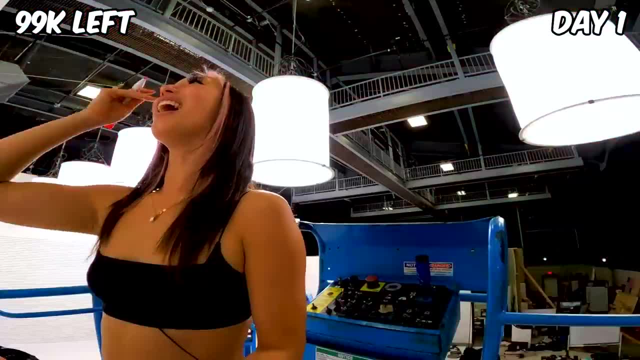 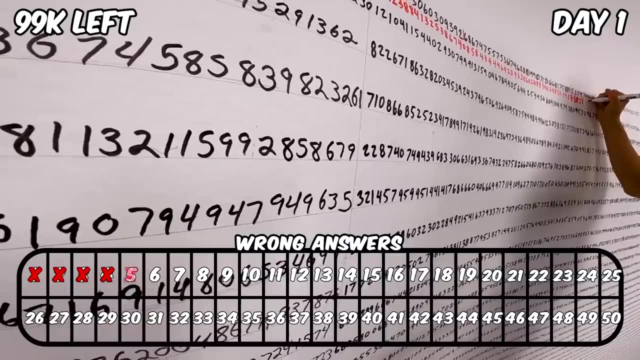 I spoke too soon. It's not a 6.. Remember, every small mistake I make is one step closer to restarting the entire problem. 5, 5, 2.. What? 5, 5, 2, 8, 2, 4, 998,, 999,, 1,000.. 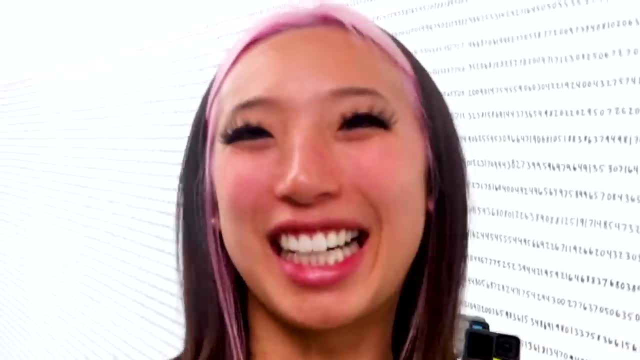 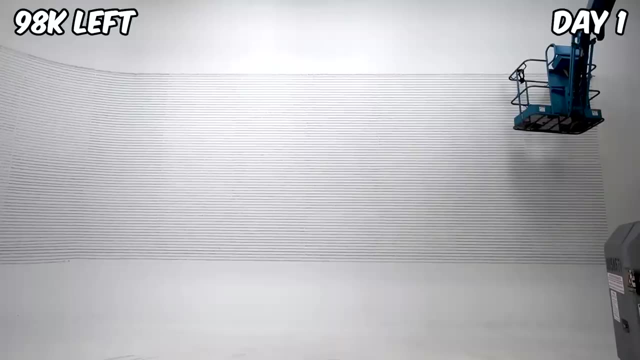 Woo, Even though I'm only 1% of the way done, I'm feeling very good. I think I can keep going. Hello, 0, 9,, 4,, 7.. Ah, I can barely make it 1, 5,, 2,, 4,, 9.. 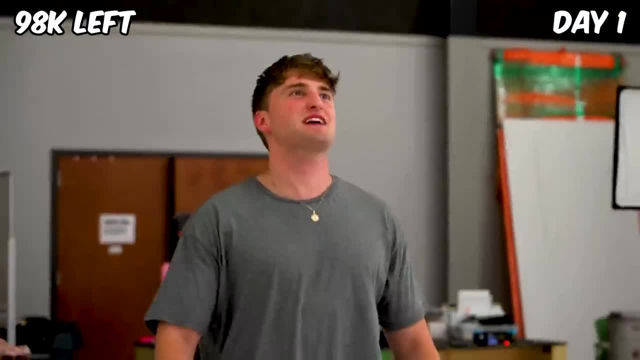 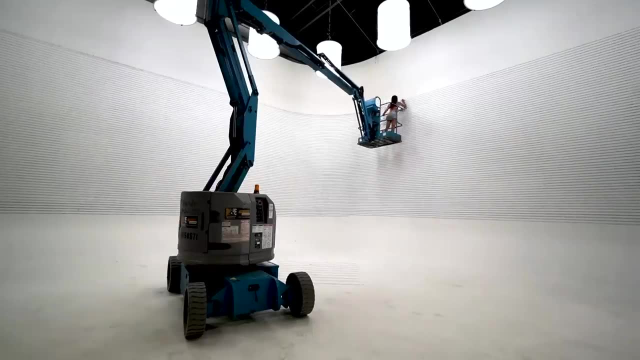 I just finished my first row. Congratulations. How many more? 68 more to go. Huh, Michelle has finished around like 1,600 digits, but that's literally only 1.6% of the entire problem. All right, I'm starting row two. 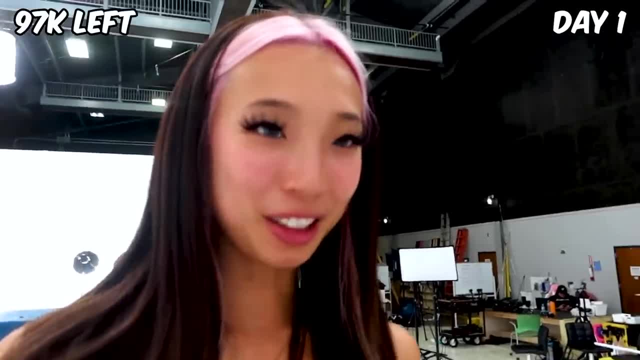 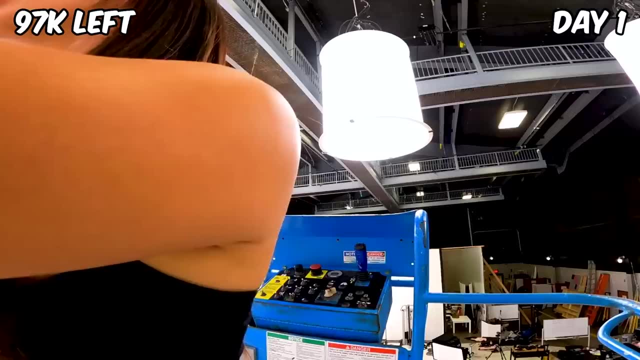 I think I need to pick up the pace a little bit more. I just realized that this GoPro probably catches my armpit. like 90% of the time Did I shoot 2,, 2,, 2. 2.. 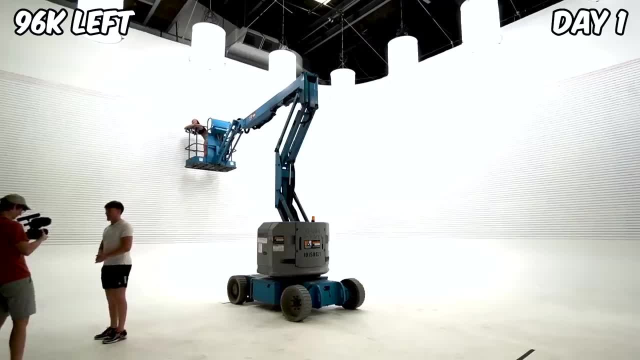 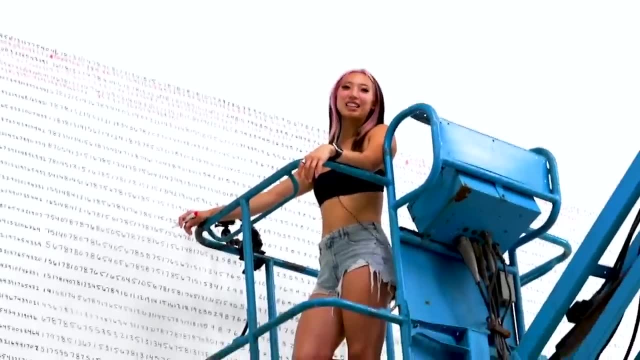 Michelle started 3 1⁄2 hours ago and, as you can see, she's barely made it there. Guess how many digits I've done: 3,500. Actually, yeah, I'm pretty good at math: 3 1⁄2 hours, 3,500, what does that mean? 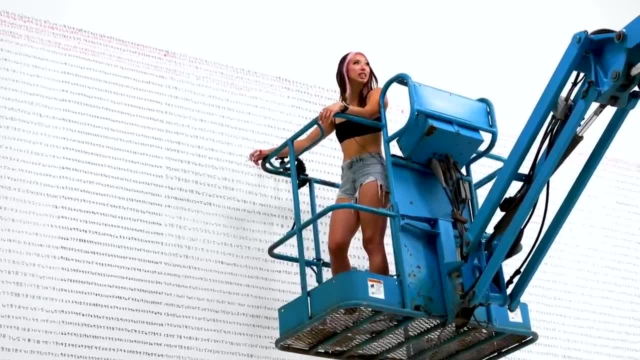 I don't know how to do math. That means I won't do 10,000 digits until like 10 hours in. What do I do? I don't know By now. in the 10,000-digit problem I'm like in the middle. 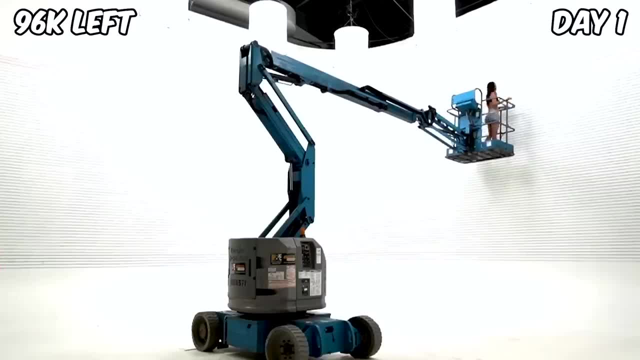 but over here I'm still at the top 4%. If I keep going at this pace, I'll finish in 75 hours. If I work around 7 1⁄2 hours a day, I can get it done. That's not too bad. 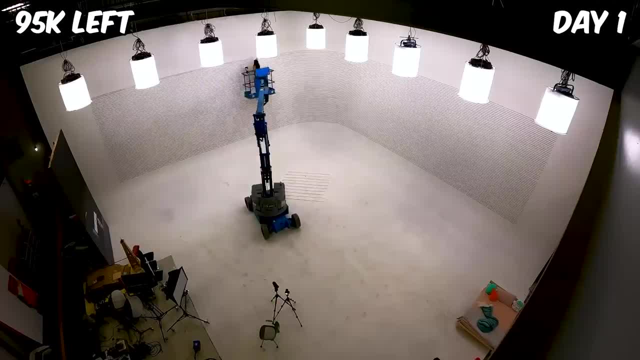 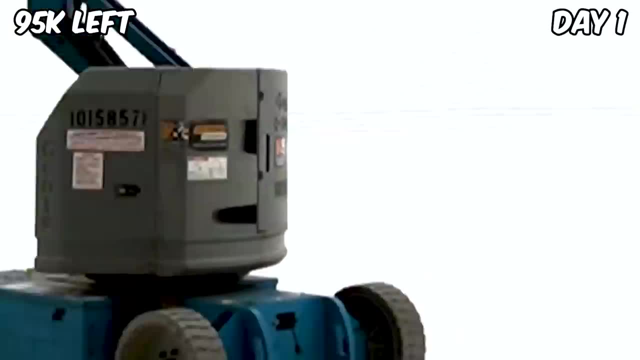 But imagine doing math for 7 1⁄2 hours every day. Oh no, I got this digit wrong. This is not an 8.. Oh wait, It's out of ink. That is not an 8. It is supposed to be a 6.. 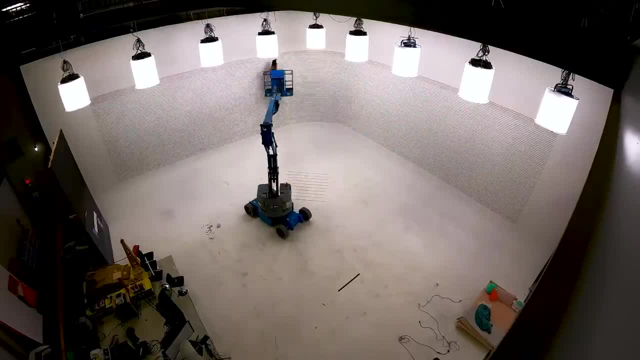 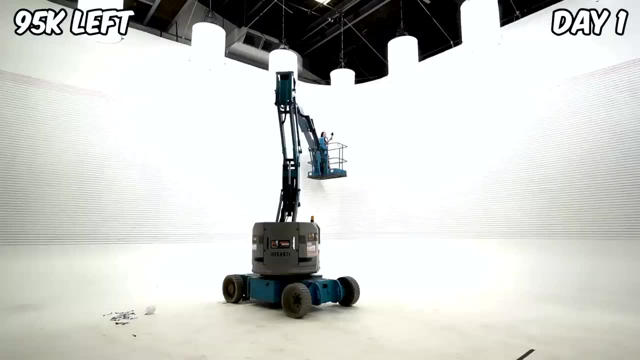 I'm officially 4 hours in and the good news is I have about 4,000 digits done. Bad news is I'm all by myself right now. My friends, my videographer, my manager, they all laugh. I got to keep going. 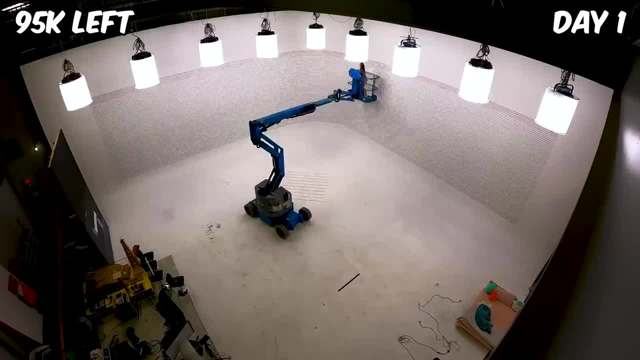 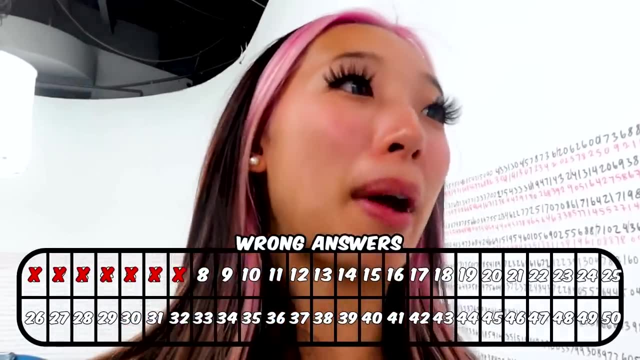 I want to finish 10,000 digits under 8 1⁄2 hours so I can beat my old time Around 5,000 digits in. and I got another problem wrong. I thought 14 divided by 8 is 3.. 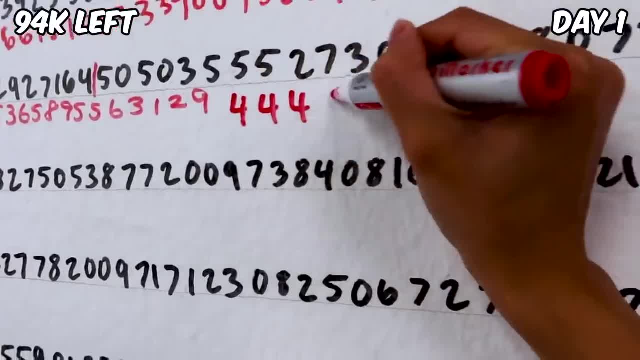 I'll show you guys my POV of the math problem. And just in case you're wondering how I don't get confused and lose track of the numbers, this is how I know to put a stop If I ever lose track of the numbers. 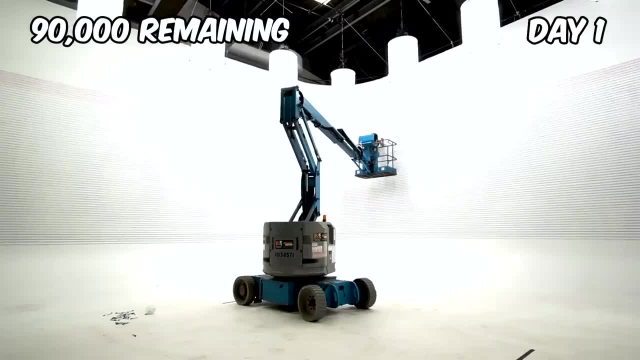 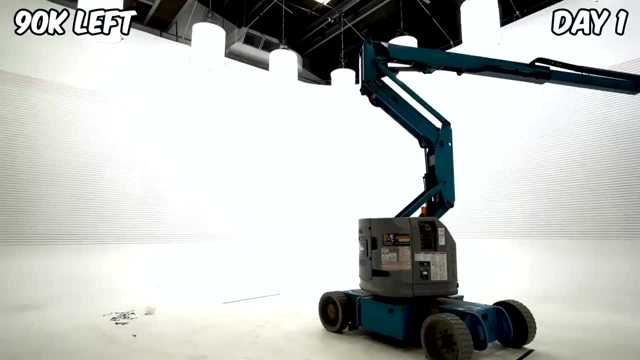 I can always go back to this checkpoint. So I finished 10,000 digits. It took me 6 hours and 57 minutes. I did not have a mental breakdown today. I am doing so well. I think I'm on track to hit 100,000 digits within the 10 days. 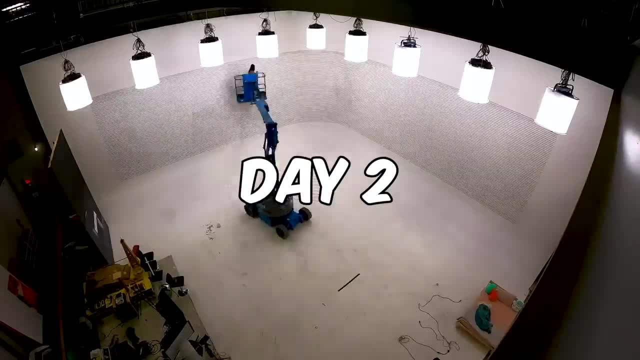 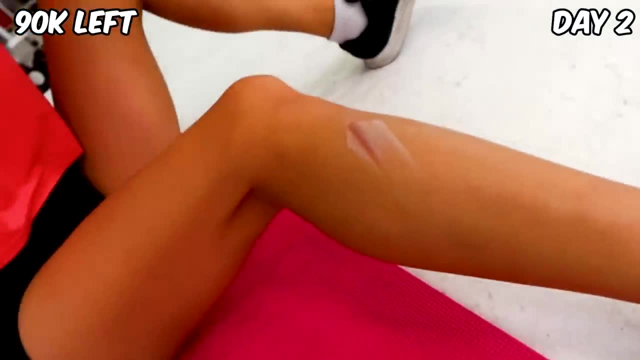 And on to day 2.. Good morning everyone. It is day 2.. Now I'm going to do a quick workout. I just hurt myself trying to turn on the light. Oh my god, It's only the second day. How did I hurt myself? 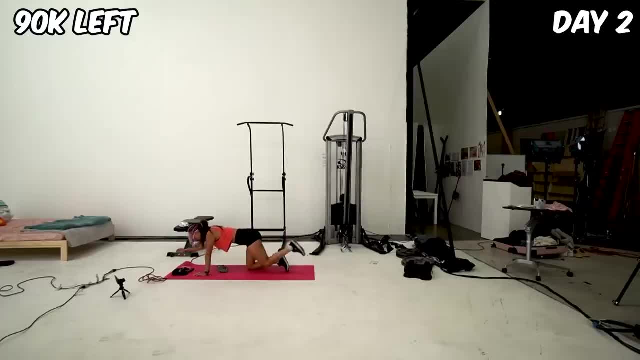 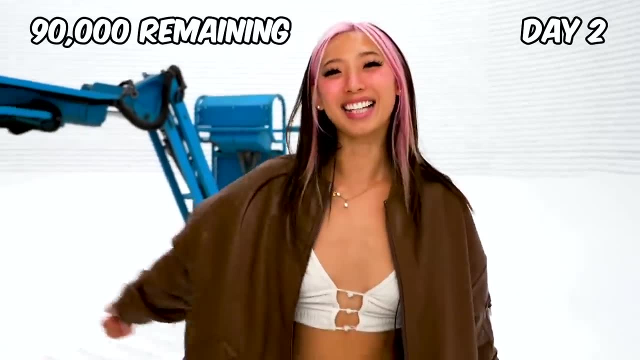 What do I do? Even though I want to finish this problem as fast as possible, I still want to try to keep my same daily routine. Well, at least for now. All right, let's do some math again. I felt like the speed I was going at. 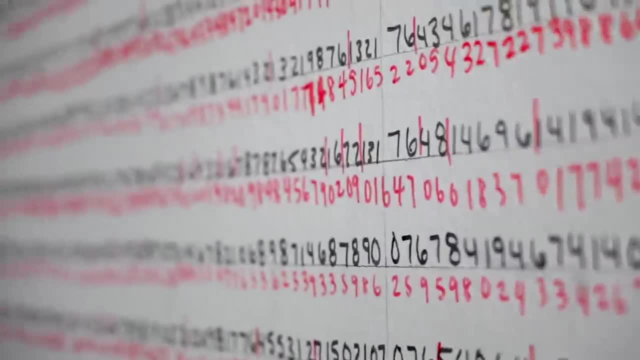 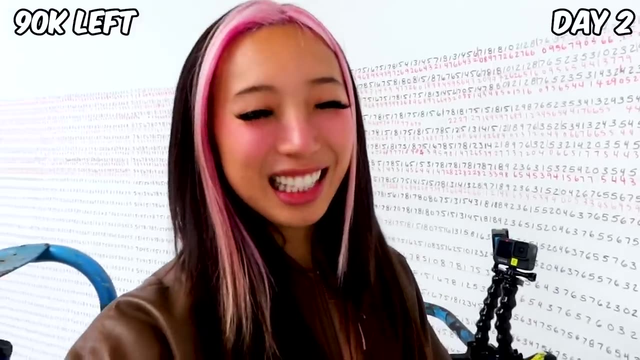 for the first day was okay, But today I want to try and pick up the pace while getting as few numbers wrong And I'm going up. So scary being up here. This is actually really cool, though. How many people can say that they've done? 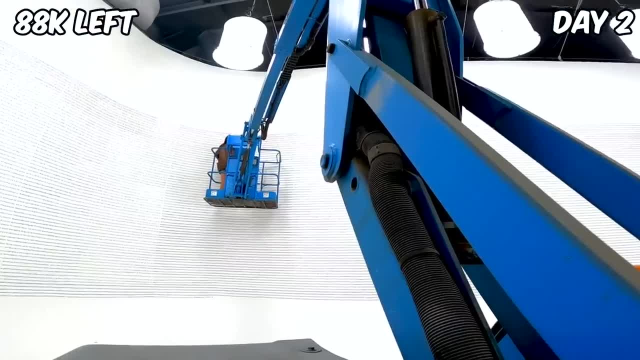 a 100,000 digit math problem? Not many people: 5,, 5,, 0,, 1.. I don't see it on here, Michelle. Something's wrong. Oh no, There was no zero. Let's go check it out, Michelle. 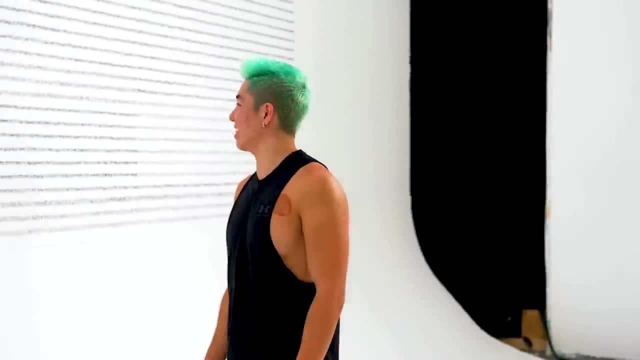 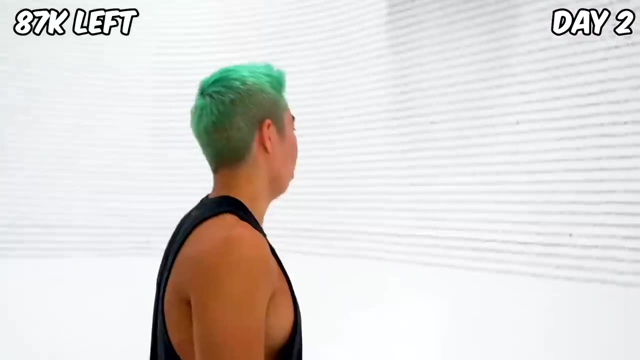 What are you on 12,273.. That's insane, But I've gotten 8 wrong so far. You can only get 50 wrong. right, I can only get 50 wrong, but I have to reset. Oh, I also broke the charger last night. 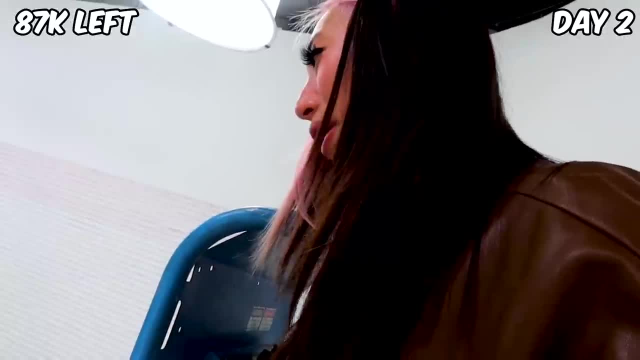 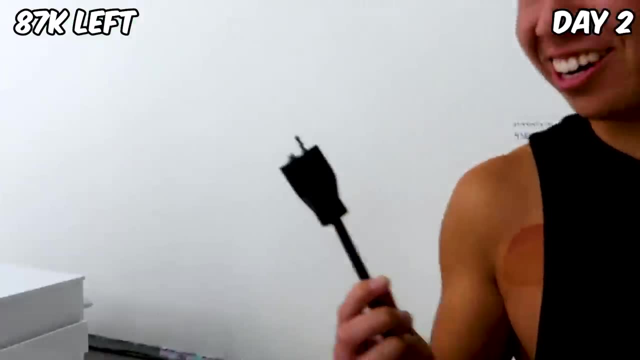 What charger? The charger to the lift? There's a charger for the lift. Yeah, I broke it. It only has one prong: It melted off. What do you mean? it melted off Where It like. melted into that. What on earth? 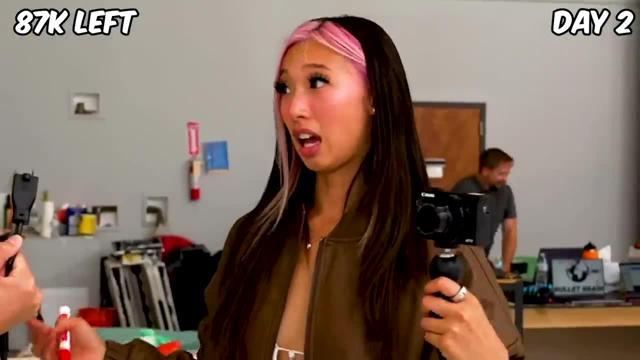 It wasn't my fault So you plugged it in. but it wasn't your fault. Yeah, And not having a charger for the lift could be a big problem down the road. Hopefully my lift doesn't stop working while I'm up there. 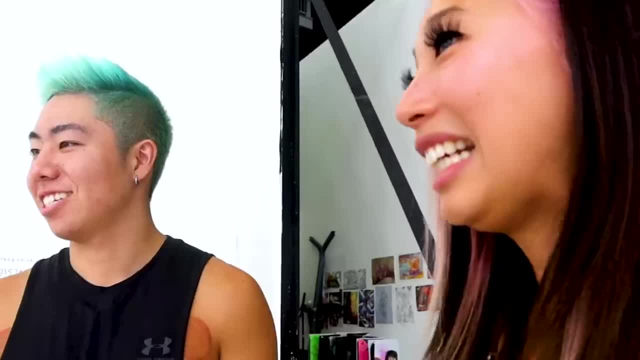 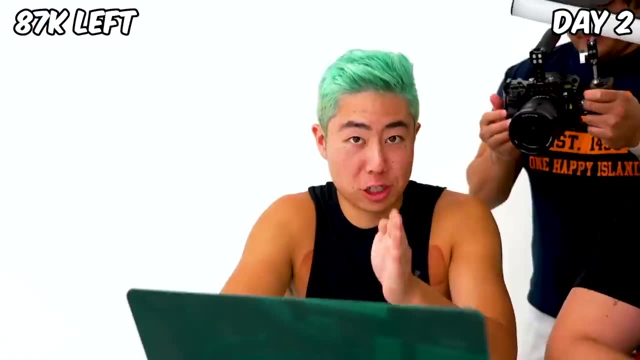 And I hurt myself trying to turn on the light this morning. I need adult supervision. We need to like Michelle-proof the entire set. I wanted to show you guys something real quick. This is Michelle's problem And just to prove to you guys. 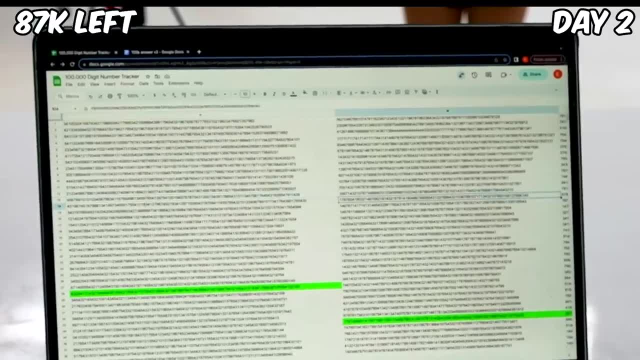 that there's literally 100,000 digits: column A, column B, and then it goes to column letter Q And if you go all the way down it shows the total over here: 100,000.. This is the answer key. 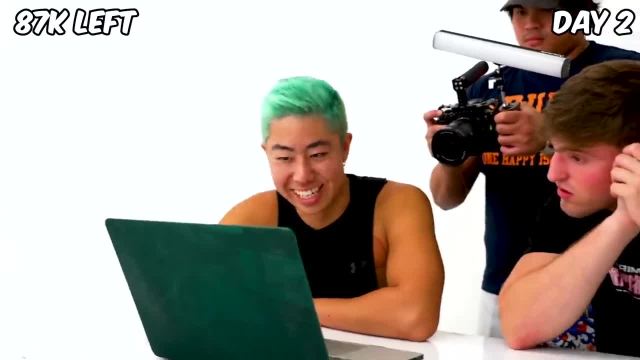 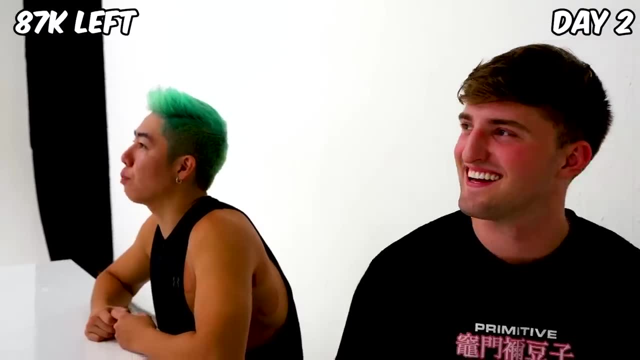 This is literally a 36-page document. That is insane. This is probably more math than what I would have done within the next 20 years. Just marry someone who can do this. Yeah, Jake, Huh, If you finish today, I'll propose. 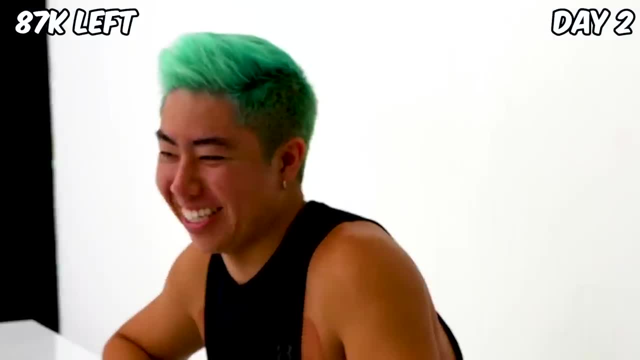 I'm working nonstop today. You have until the end of the workday. Let's end work early, 4 pm. You can do it. Is that too little time? Wait, should I make it shorter? You want to check my answer? 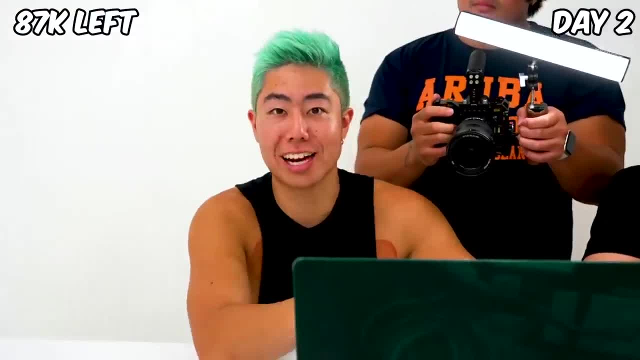 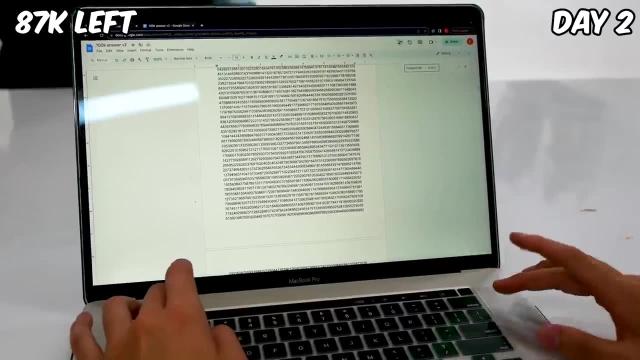 Right now Michelle's going to say the numbers, just to show you, guys, that she's not actually BSing this: 7-7-7-5-5-4-9-7-1-2-9.. Oh, wait, wait, wait. 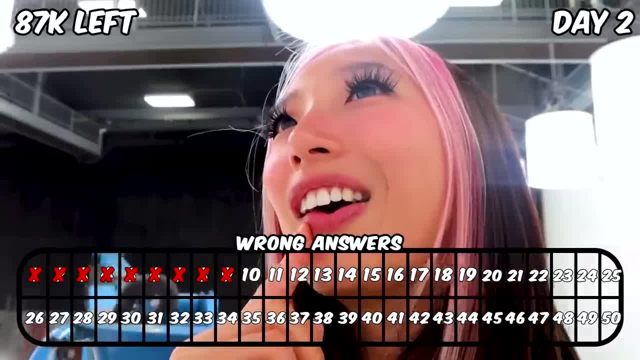 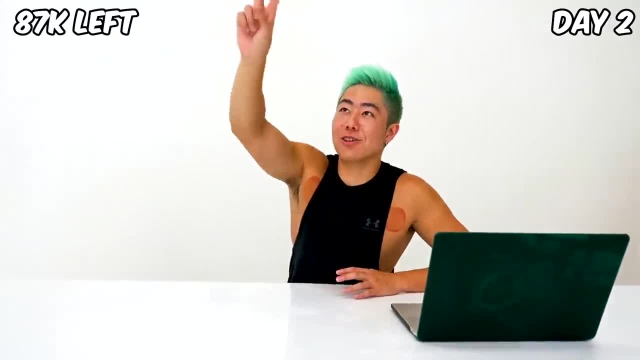 1-2-what? Um, Anne, You got it wrong. Uh-oh, Michelle, I think that was number 9.. 41 more to go. No Wait, Michelle, I have a challenge for you. Jake has to do your next 10 digits. 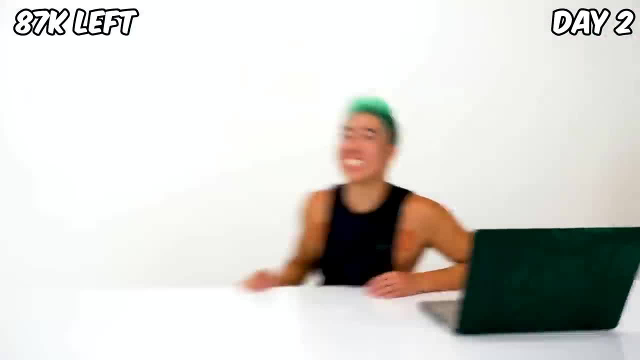 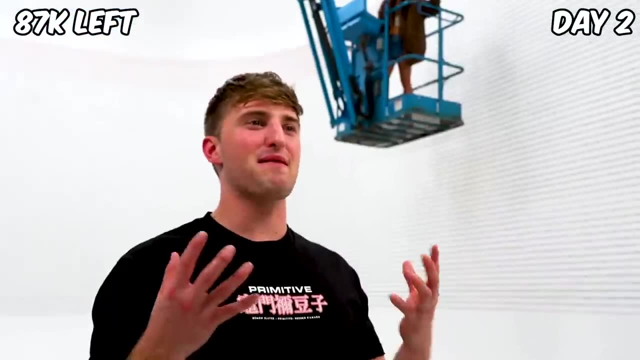 but if he gets any wrong, that goes towards your total. What Wait? I can't learn the abacus that fast. This might be the end for me. I have a 10% chance for each digit to get it right. Jake has never done math like this before. 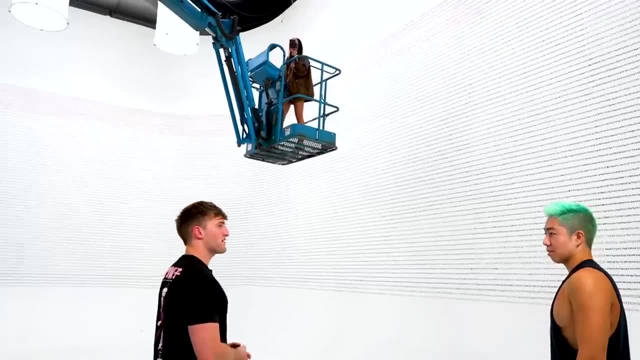 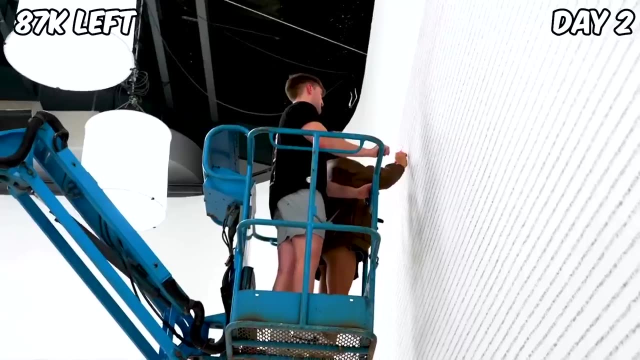 and, if I'm going to be honest, this makes me a little anxious. Oh my god, What if you have two human calculators? I reviewed some basic divisions with Jake and showed him how to organize his numbers in the same way I do. 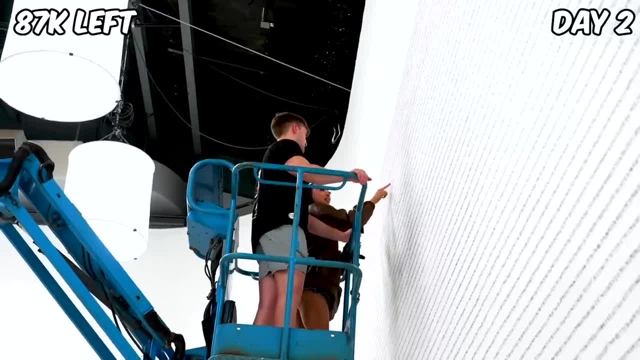 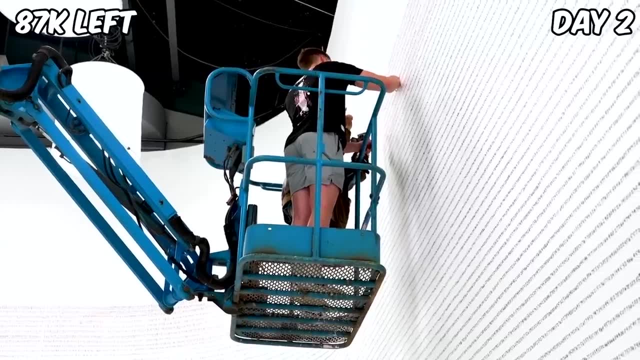 What goes into 25? 3. So this becomes a 1.. What goes into 12? 1. So that becomes a 4 and a 46.. Wait, what 25 minus 24 is 1.. And then 1 to 2?. 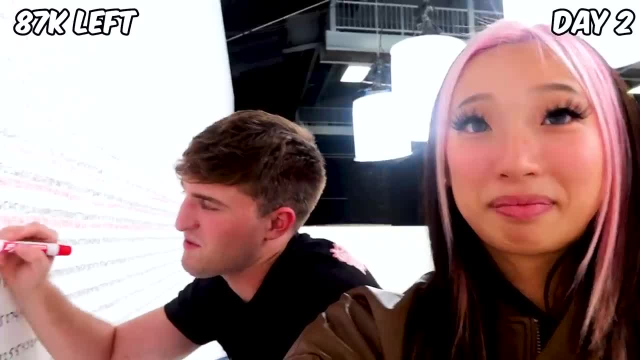 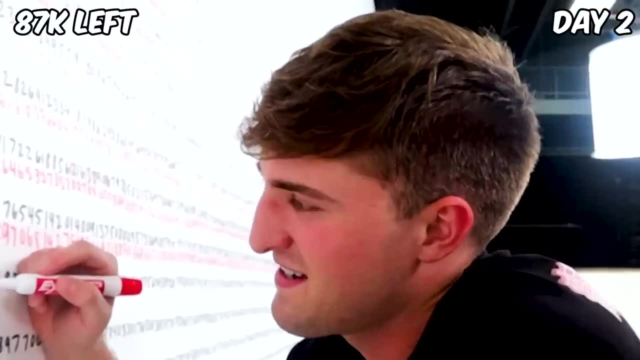 Yes, Oh wait, I can't help you, I'm just going to cry. So 64 minus 8, 56.. Yeah, Despite all odds, Jake is starting to get the hang of it, but there are still times where he had trouble remembering basic math. 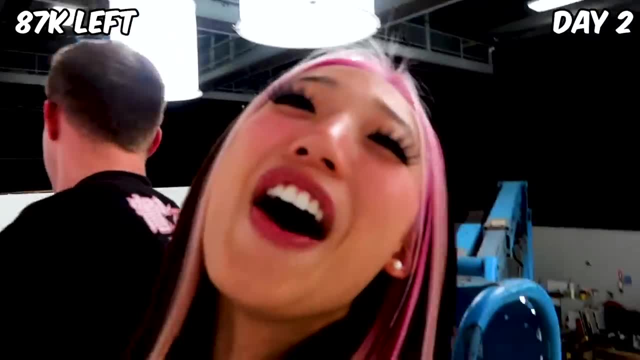 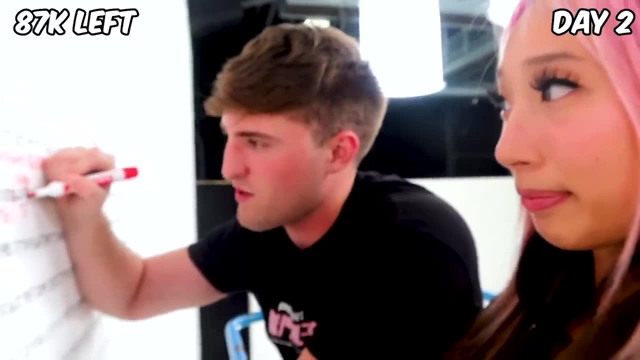 Wait, No. No, Zach couldn't have chosen anybody else, but he chose Jake. Okay, so then the 4 goes to Okay. so then the 4 goes to 44.. So then it's 5 again, but that's a 0. 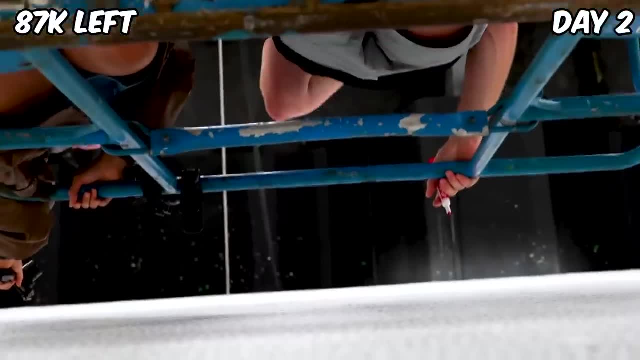 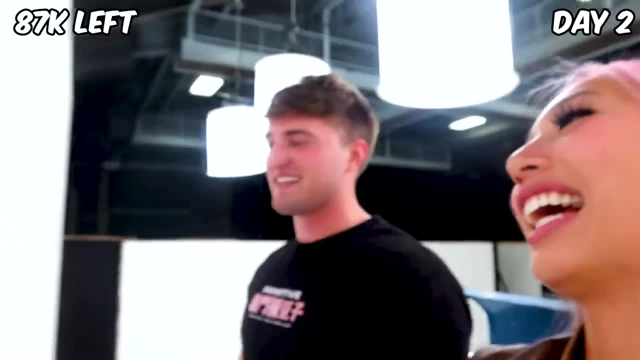 0 minus 5 is negative 5.. Yeah, Yeah, yeah, that's the one. Now do I do 50? And I say that it goes in 6 times. I can't help you, but you are on the right track. 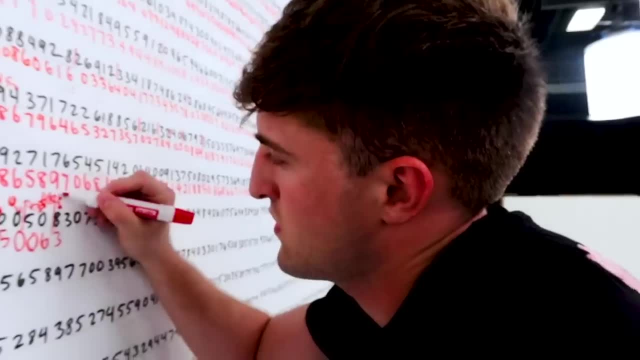 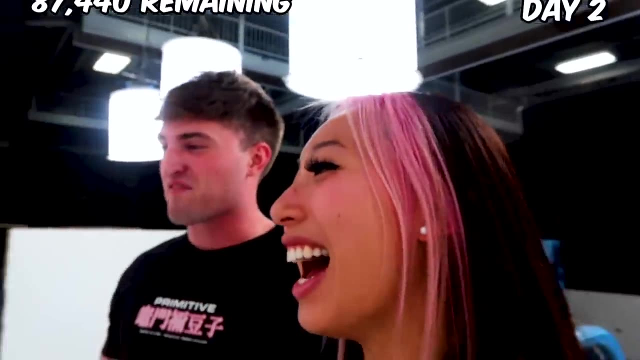 Surprisingly, against all odds, Jake actually started to get the hang of it: 43 by 3.. Yay, Good job, Jake. Wait, did I finish? That's enough, right? Yeah, that's 10 digits. 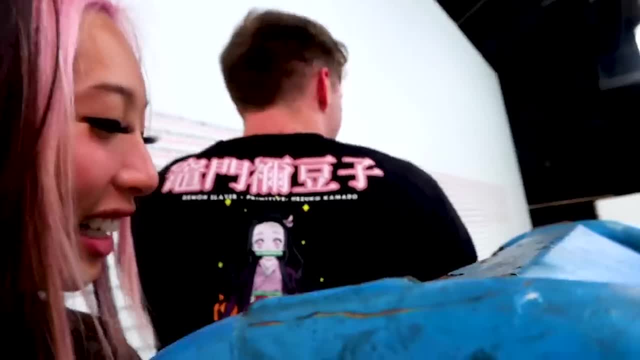 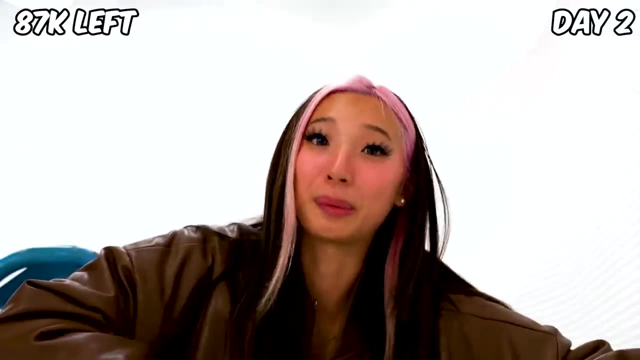 Woo. Oh my god, I was sweating. I did it. Alright, let's bring you down so you don't write any more digits. Yep, get me out of here. I think Jake did a great job, but I'm glad he's not helping me anymore. 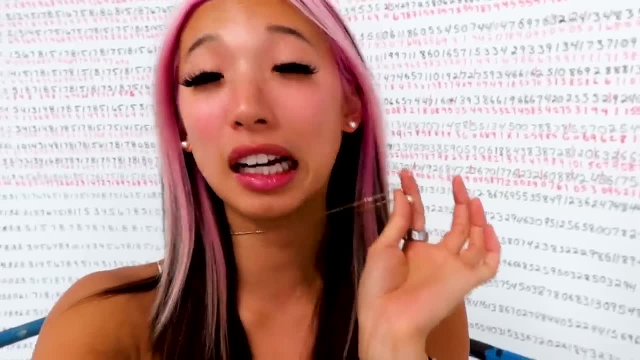 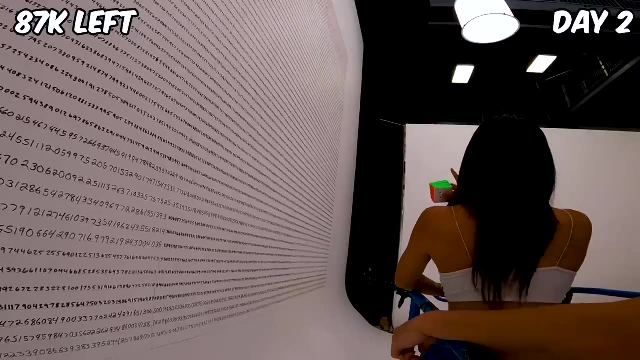 It's the middle of day 2.. I'm slowly getting a little bit tired. To make things a little bit more fun, I brought Ben up on the lift with me. Alright, Ben, if you can solve this Rubik's Cube before I solve 100 digits, you win $100.. 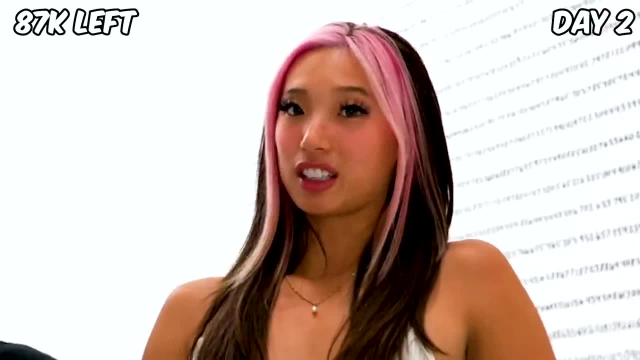 Might as well. just give me the $100 now, And if I lose I have to wear drunk goggles for 30 minutes. How fast can you solve a Rubik's Cube Like 10 seconds? Definitely can't solve 100 digits in 10 seconds. 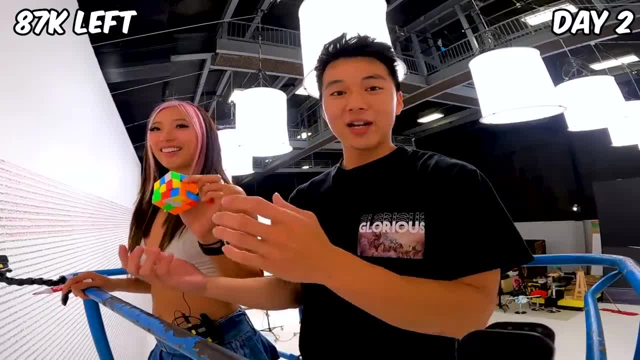 Alright, let's go up. You guys are so small down there. Fun fact, I just learned how to solve a Rubik's Cube, like a day ago. Wait, let me mix this up a little bit more. No, I think that's fine. 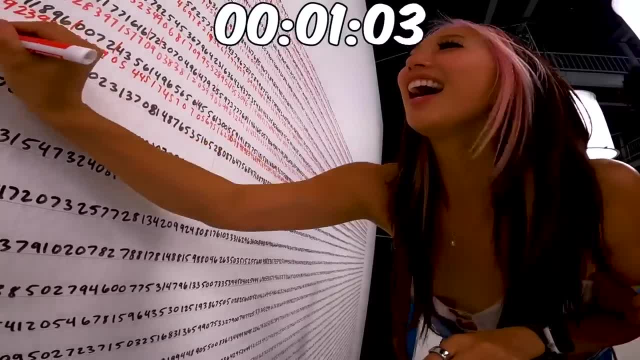 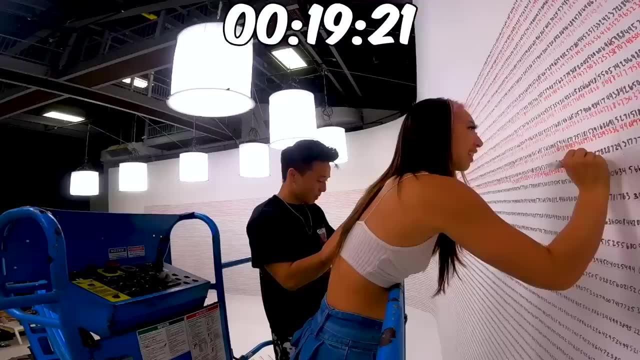 Okay, 3,, 2,, 1, go, Oh god, Ah, Where is 0, 0?? Oh my god, Michelle, I'm almost done. No, you're not, I'm going so slow, Okay. 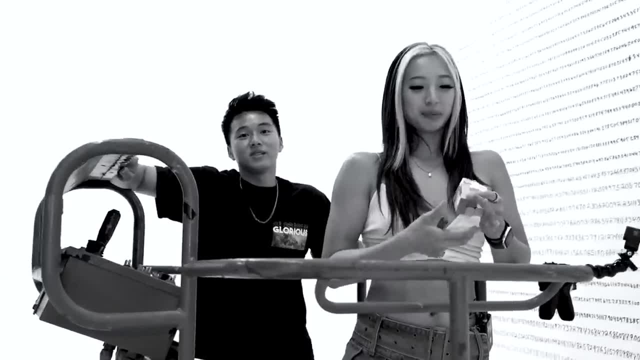 Wait, I think Michelle's actually going to destroy me. How fast can you solve a Rubik's Cube Like 10 seconds, Bro? 3, 2,, 3, 1, go Done. Just kidding. Oh my god, you scared me. 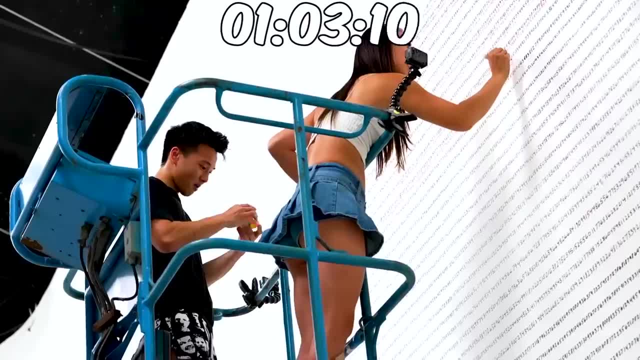 I still have like 20 more to go. I'm almost done. I'm almost done. I'm almost done too. No, I'm almost done. I'm almost done. No, no, no, but I'm almost done. 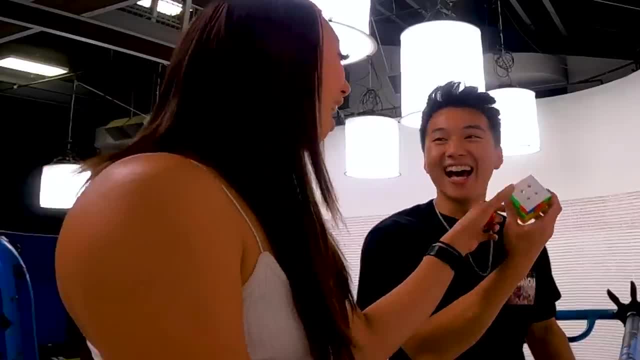 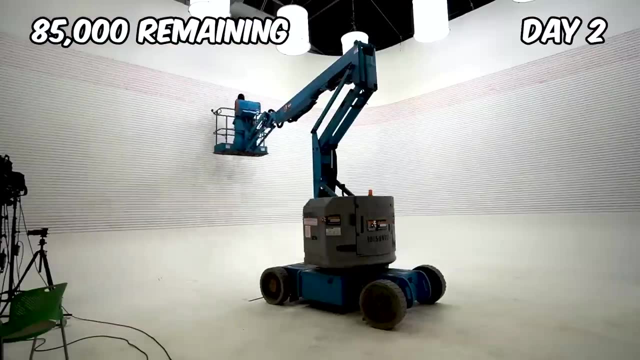 1, 3,, 1, 3, done. Did I get it right? Solved one side- Whoa, Thank goodness. I did not want the goggles, I got absolutely destroyed. After Ben left, I was able to concentrate on my math problem. 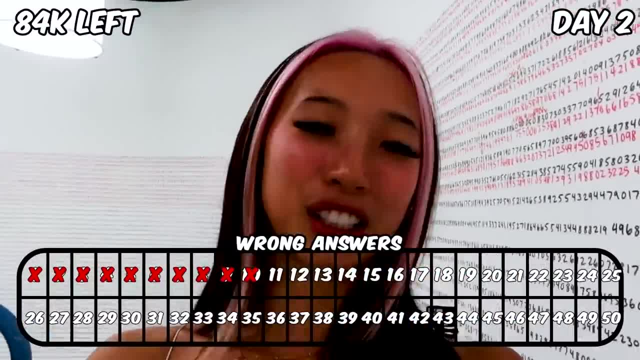 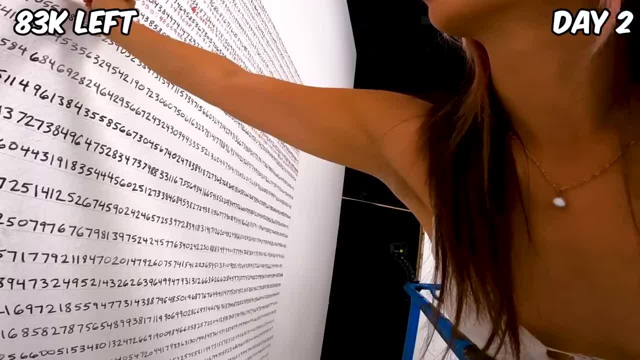 Oh no, I got this digit wrong. Now I have to redo 12 digits. Alright, I am about 16,500 digits in and I'm getting really tired. I'm going to grind out till I hit 20,000 digits. 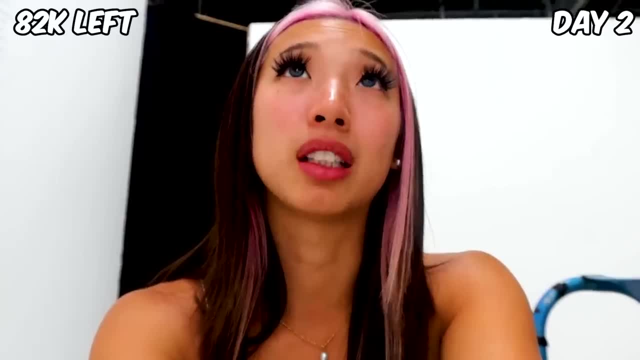 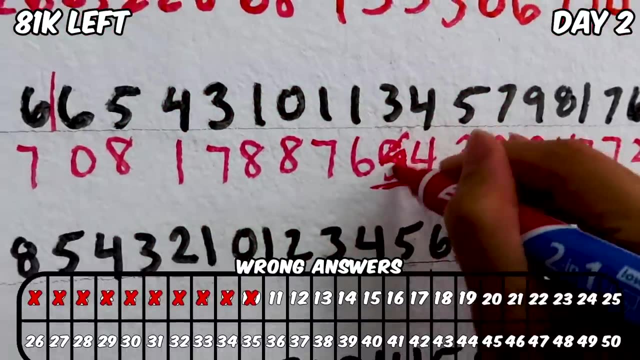 Otherwise, I'm going to be really, really behind. This math problem is a lot harder than I thought it would be. To make things worse, I just made another mistake, which means I'm at 11 mistakes, now 4,. it's getting pretty late right now and I think I'm going to go to sleep. 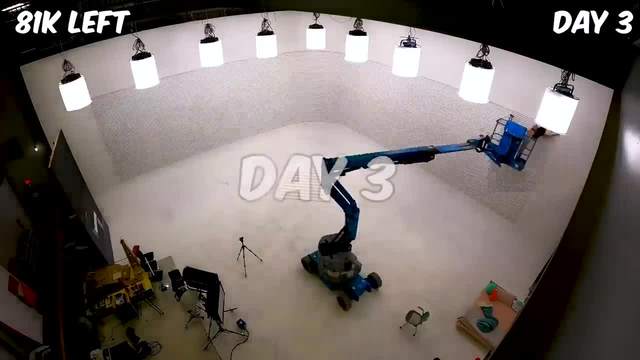 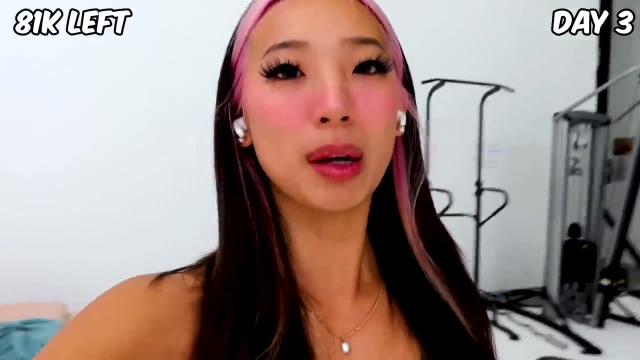 I'll just do more on day 3.. Hopefully It is officially day 3 and I got tons of sleep and I feel super energetic for today. I'm going to go work out and then start on the math problem. I am a little bit behind. 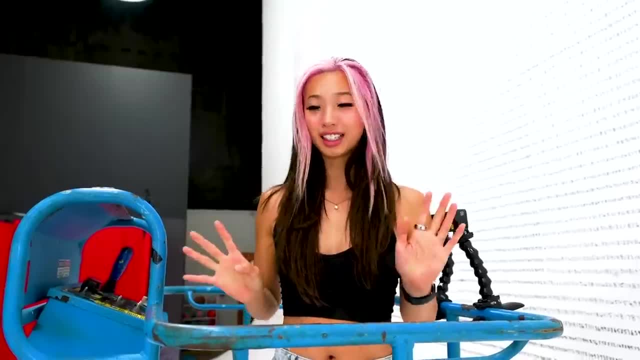 I need to hit at least 30,000 digits. I have to be very, very careful today to be on track. I really do not want that taser. I am at 11 mistakes. I am not on track to hit under 50.. 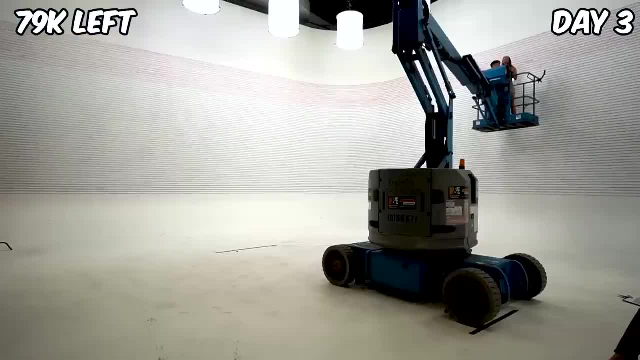 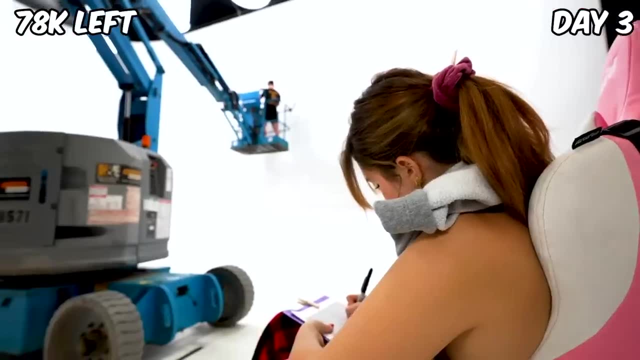 I have to be very, very careful today. Oh wrong one: 4, 9,. 8, 9, 0,, 4, 7.. And just when I thought things were going well: 8, 5.. 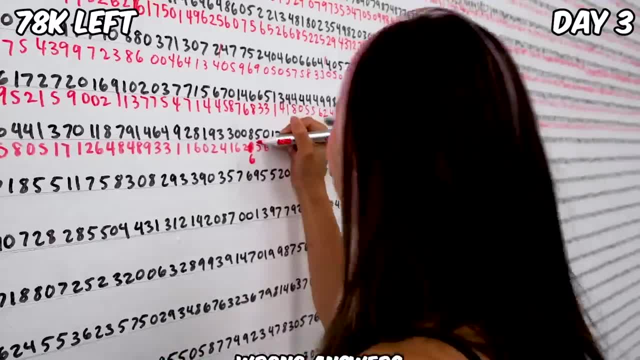 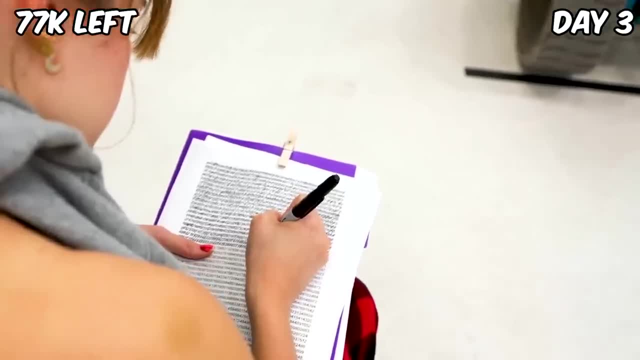 Did you say 8?? Oh, no, I got it wrong 6. Yes, Yep, Oh. Even though Michelle is behind, I still think that she can do it. I have a lot of faith in her. I needed a small break, so I let Jake control the lift for fun. 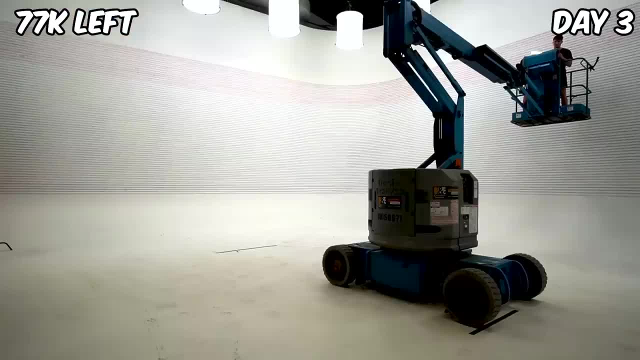 What did that do? What did that do? What's that doing? Let's go down, Wee. There's a lot of arrows and I'm not really sure what they mean. Wait, what's this one? That one's the scary one. 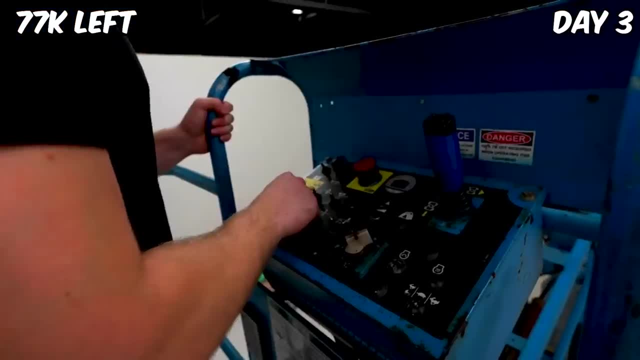 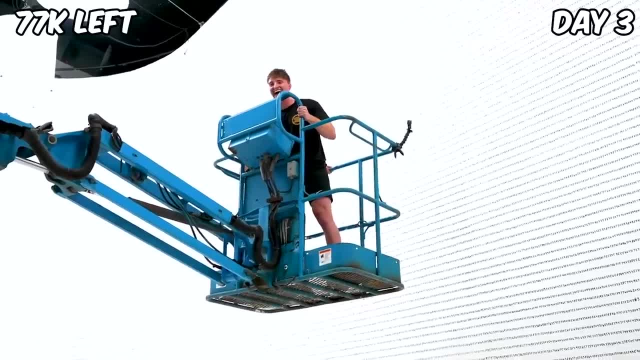 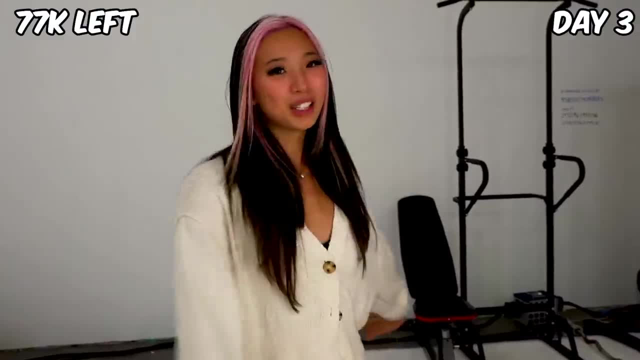 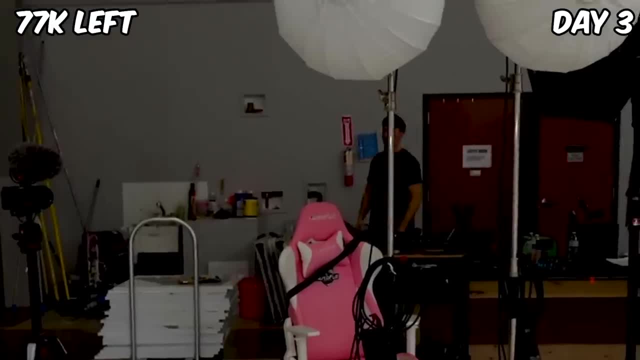 So relaxing Stretch. Do you want to give me a back crack, Back, crack. Uh-huh, I'm ready. Did you hear that? I couldn't tell if it was a lot or a little. It was a lot. I should get back to work. 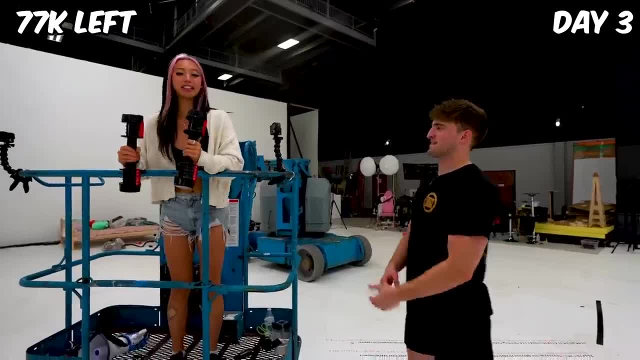 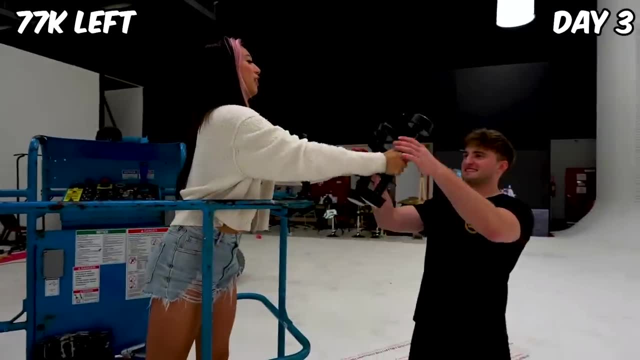 All right, Jake, I have an idea to keep me motivated. It gets pretty boring solving this problem, so doing these challenges definitely helps keep me entertained and focused. If you can do 100 curls before I finish 100 digits, you get to bother me for 15 minutes. 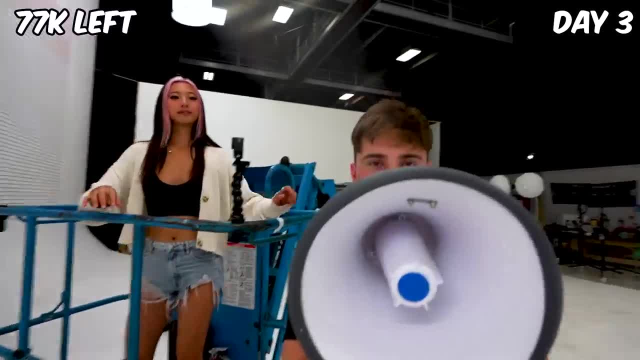 And you win $100.. 100 digits, easy. Michelle's going to lose And then you're going to have to deal with this. I said yeah. I said yeah, I don't like this idea already. All right, let's do this. 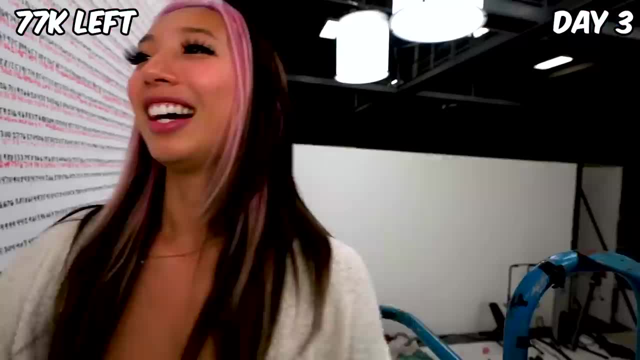 Three, two, one go One, two, three, four, six, zero, six, nine ten. Oh wait, I forgot to count Three, two, one go. One, two, three, four, six, zero, six, nine ten. 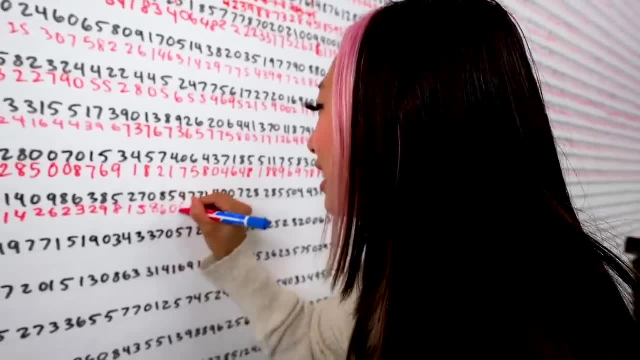 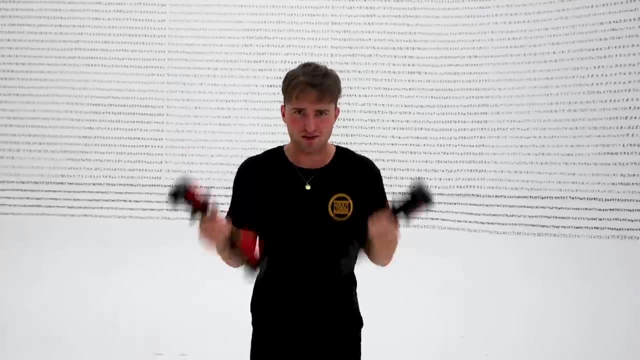 Oh wait, I forgot to count Three, two, one go One two, three, four, six, zero, six, nine ten. I think I was going a lot faster than I thought. This is not looking good for me. 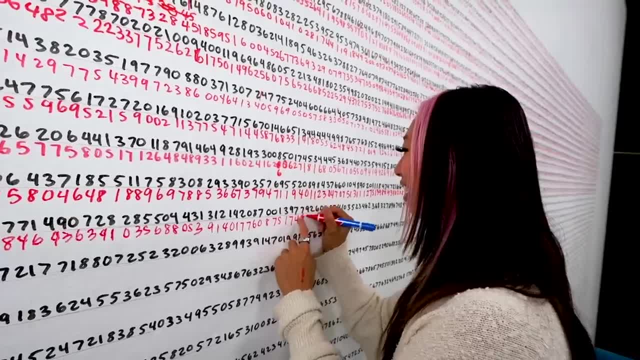 Think I'm halfway there now. Oh, oh, what, what? I need to go faster. 71, 72,, 73,, 74,, 75.. Oh my god, 79,, 80.. 91,, 92,, 93,, 94,, 95. 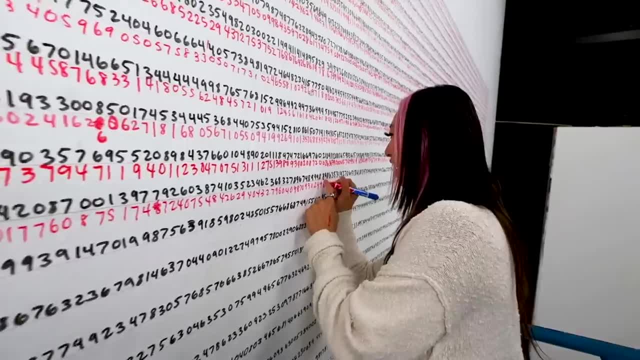 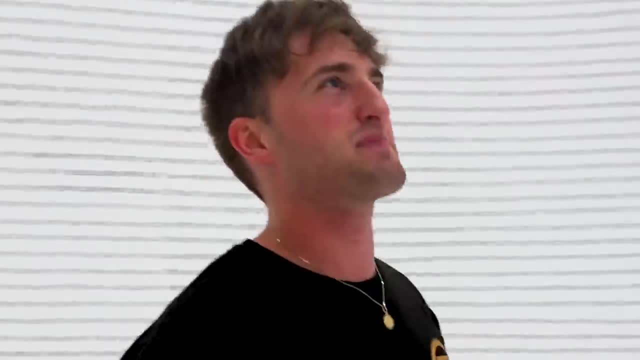 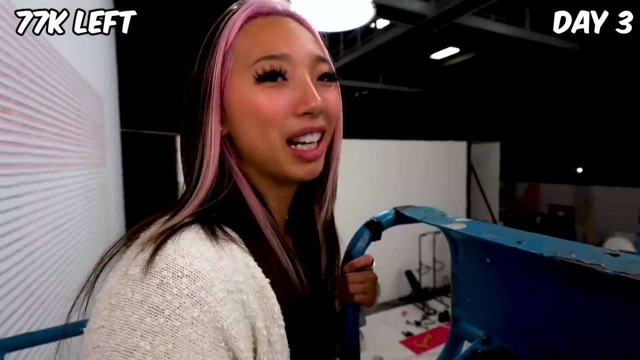 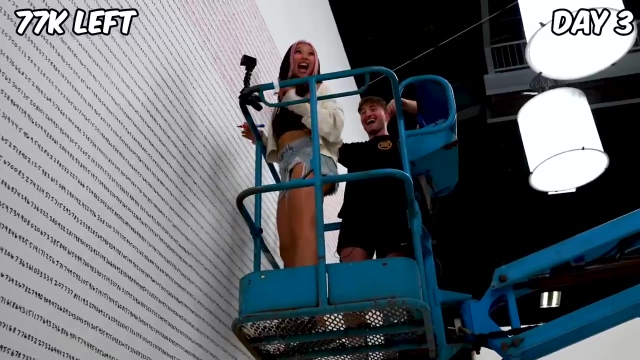 Ah, next, We're close 100.. My biceps actually burn way more than I expected. I have about 24 left. I'm already annoyed. 15 minutes have passed. What is up, Ms Munchyfab? 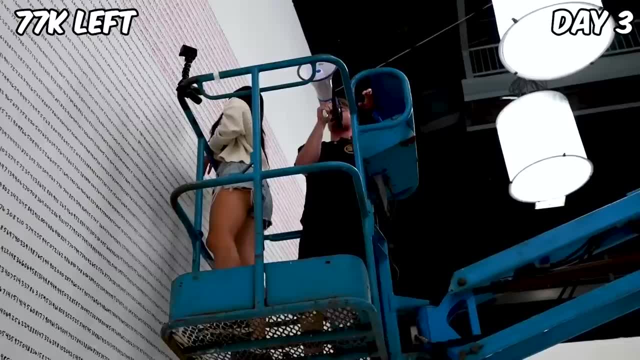 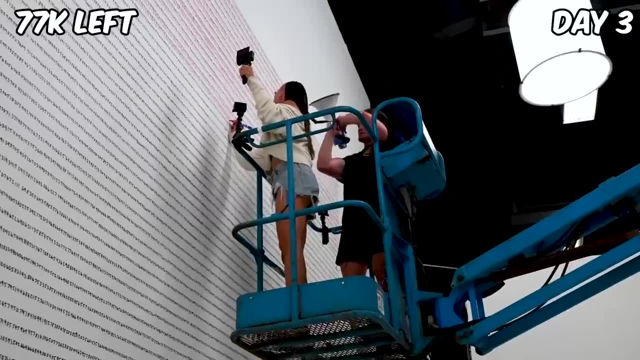 She's currently over 20 Ls in digits. Can she finish? How much longer? You'd think Jake would eventually get bored and stop, but he didn't Ow, And unfortunately for me. I think Jake was actually having way too much fun bothering me. 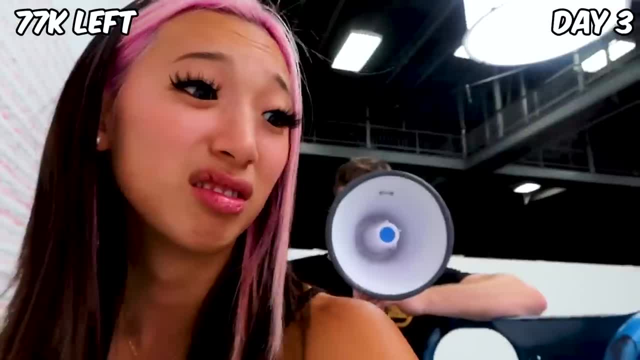 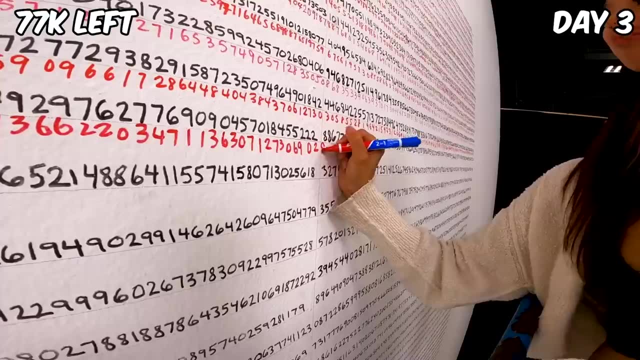 Hurry, Are we done? Are we done? It may seem like I'm pretty annoyed with Jake, but deep down it was actually the most fun I've had all day. Thanks, Jake. She's writing. When will the first mental breakdown come? She's writing. 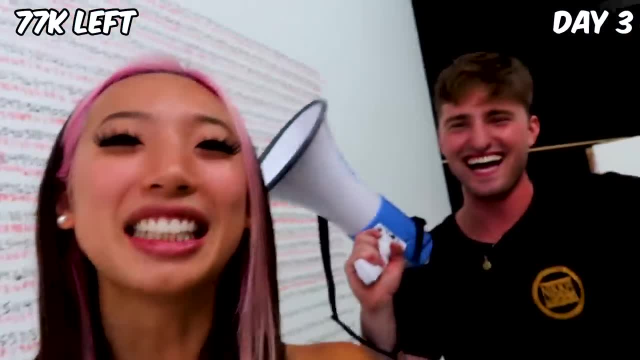 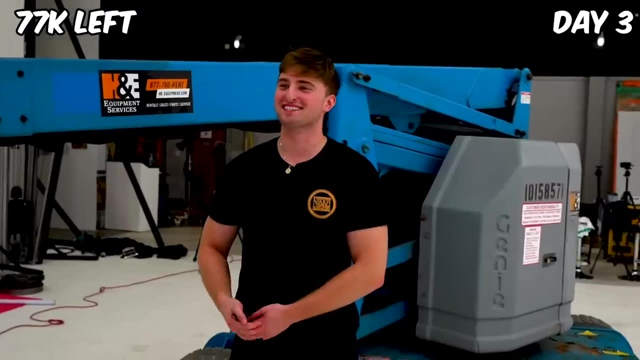 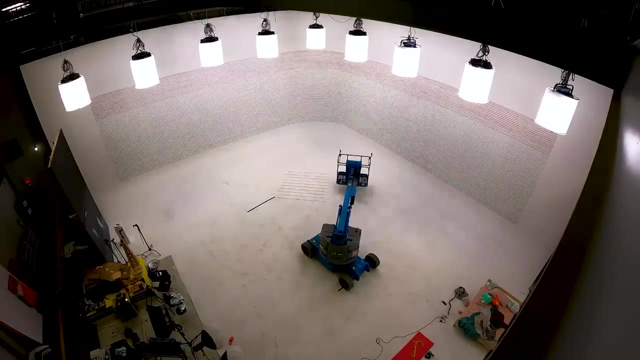 I like that, And the 15 minutes is finally up. Even though Jake was super, super annoying, Math was actually quite fun. I thought you were going to say it helped you work faster. Well, it really didn't. I've been doing math for a while now and I am so, so, so bored. 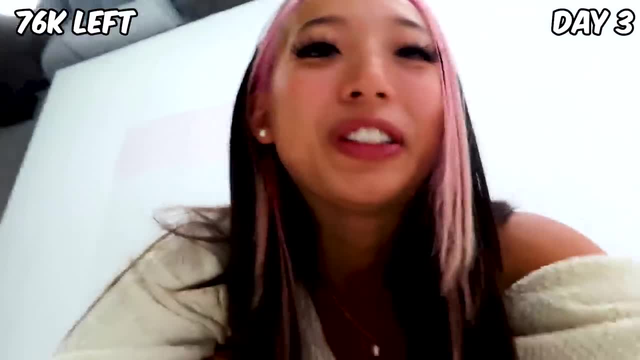 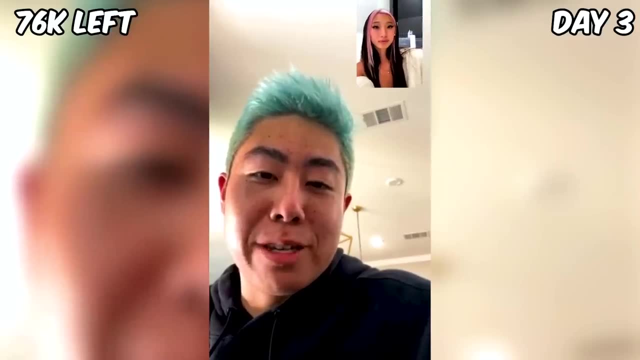 I'm going to call Zach. I miss him a lot. Hi, I miss you. How many have you done? I'm like about 23,000 today. I'm kind of behind. You should run a quarter marathon and then you'll be grateful you're doing math and not running. 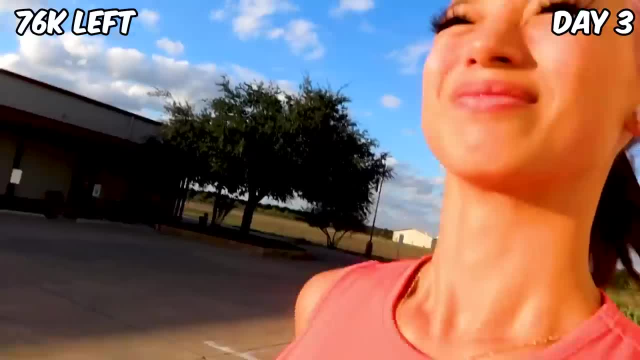 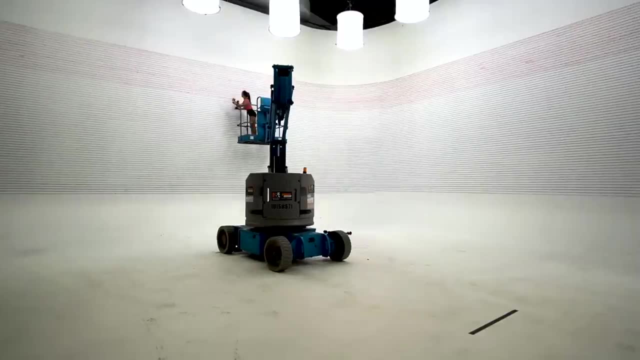 That is very, very true. I hate running. Let's go run. After going on that run, I feel pretty good now and I'm going to try to do two full rows without stopping. I don't think I'm going to do 30,000 digits by the end of the day. 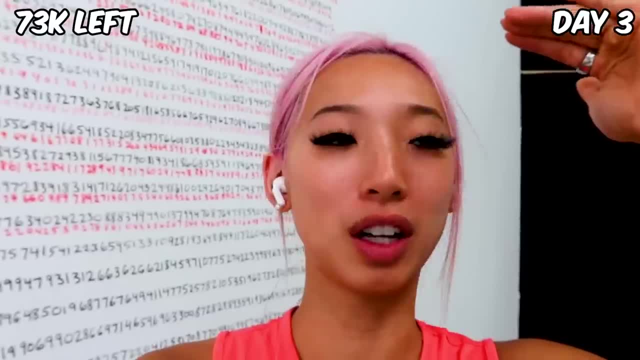 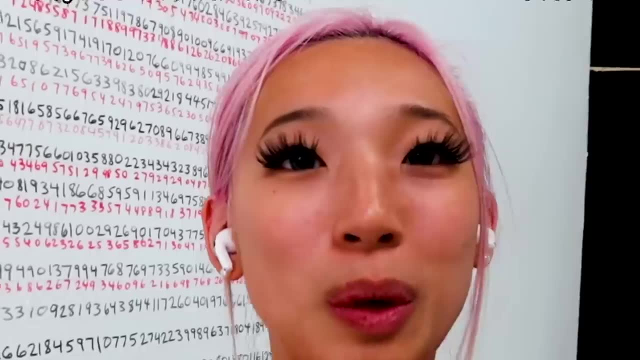 but I'm going to try my best. I just worked two whole rolls, Rows, Whole rolls. I can't even speak now. I just finished two whole rows and now I am officially at 27,000 digits. I am still a little bit behind. 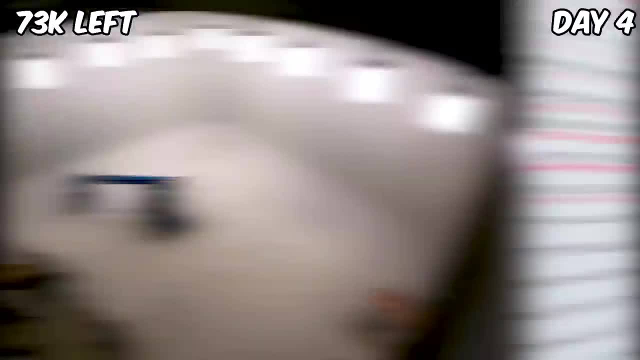 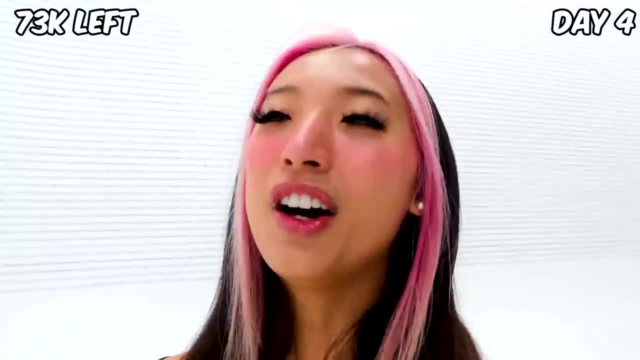 I am so exhausted I'd rather start fresh tomorrow. Good morning, It is day four. I did not get much sleep last night. I think I'm going to get an ice bath to try and wake me up, and hopefully today will be a very, very productive day. 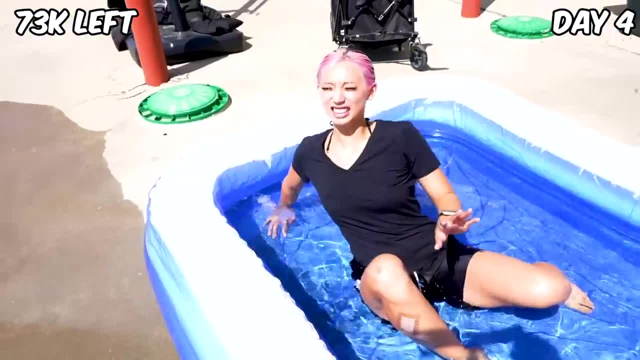 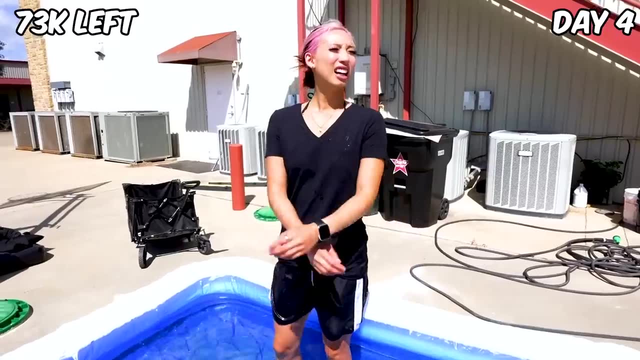 Wow Cool, This is really waking me up. I'll do a quick dip. Okay, it looks like I'm peeing. I feel good. I feel good, Get to work. Not long after taking the ice bath, I encountered a huge problem. 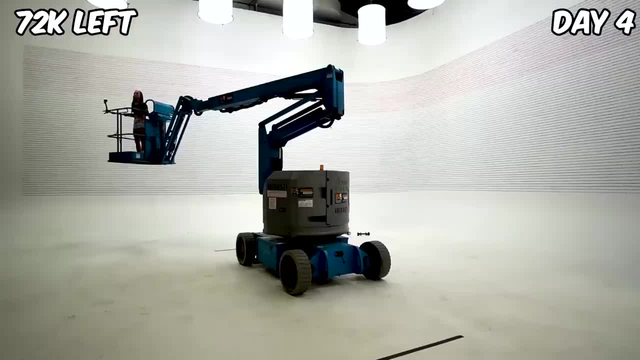 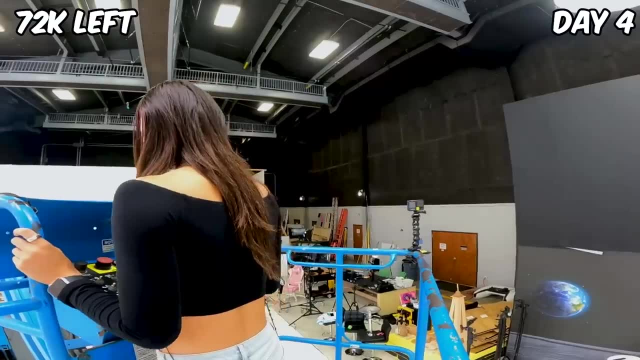 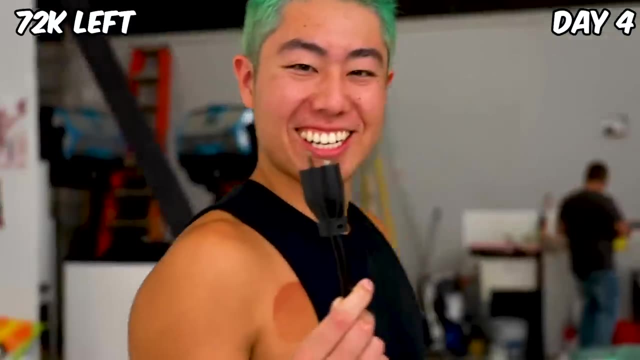 Guys, Guys, Mar. Oh, I think they said they went out for lunch. What do I do? Hello Guys, I don't have my phone. So it turns out the battery died on my lift. I think it's because I broke the charger on the first day. 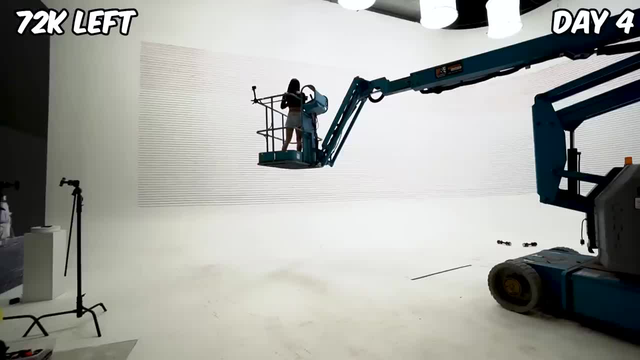 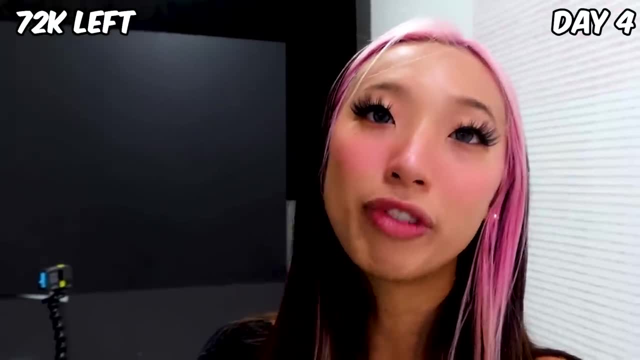 and now it's finally out of battery. Nobody is here And I am stuck. How am I stuck right now? No, Oh no, I know, I know, I know I also left my phone right there. This cannot be happening. 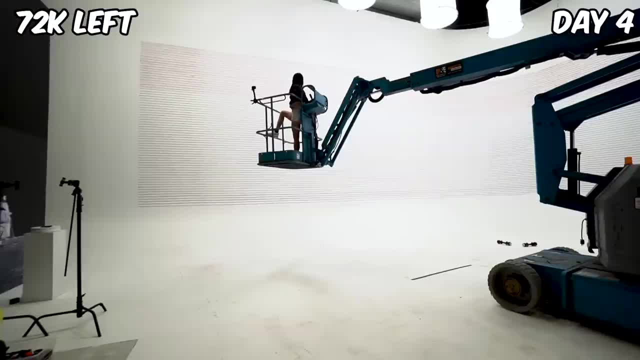 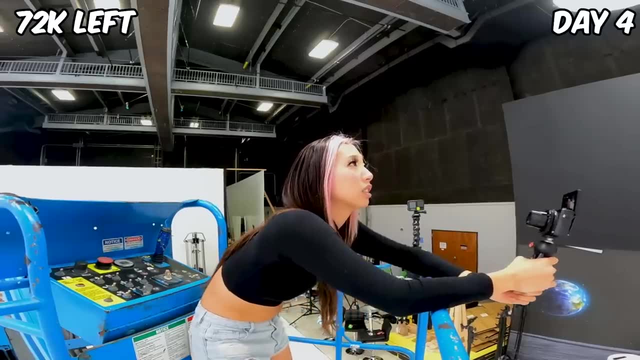 Lunch is only like an hour. They'll be back soon. How am I going to finish the math problem? I'm already behind as it is. No, I'm not going to finish at this rate. Somebody, Somebody, help me. Well, let's make noise. 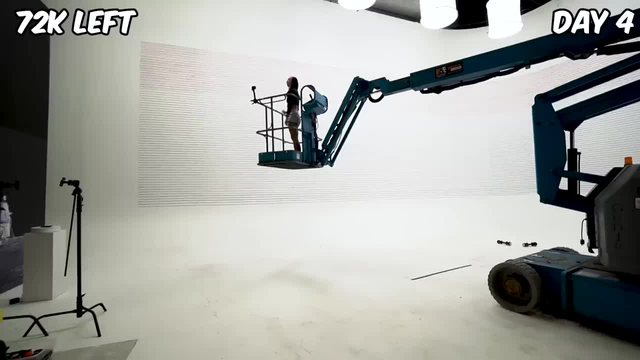 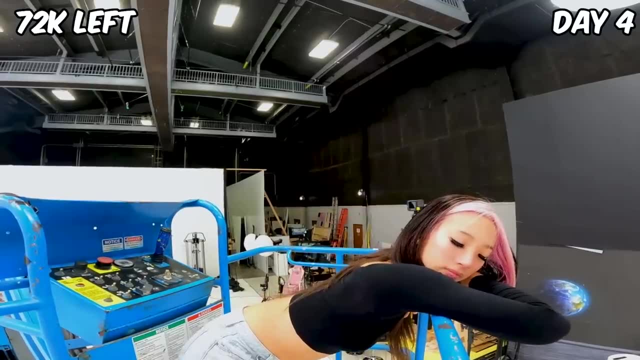 Help, Help, Help. Literally nobody is here right now. After yelling for help didn't work, I tried figuring out different ways to get down. I'm already falling behind, so I might as well try to get off this thing. First I tried to see if I was low enough to jump down. 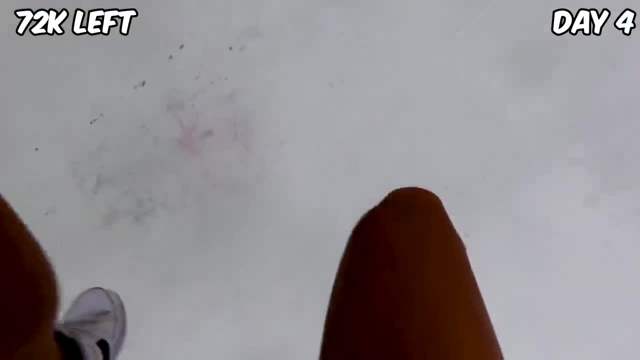 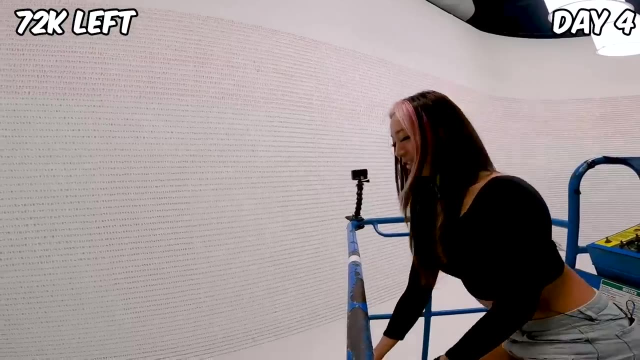 I think I'm a little bit too high off the ground, And Never mind, never mind. I even tried to make a rope out of tape. Is that strong enough? I'm scared, though, And then I went to just calling for help. 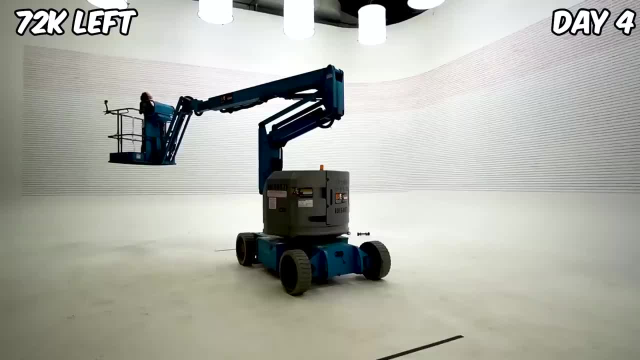 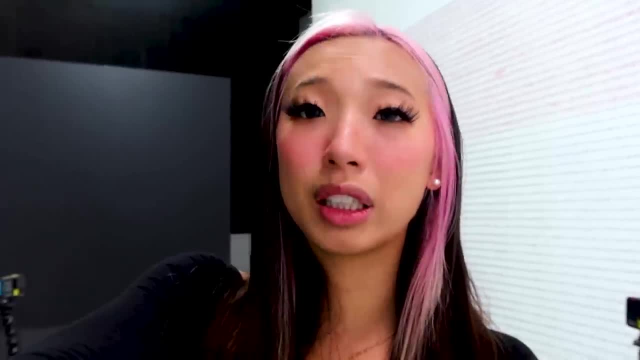 Come on guys. Peace Anybody. This has got to be like the worst day so far. I did ask Jake to bring me my lunch yesterday, so hopefully he'll be coming in soon. I'm trying not to cry. I'm going to get through this. 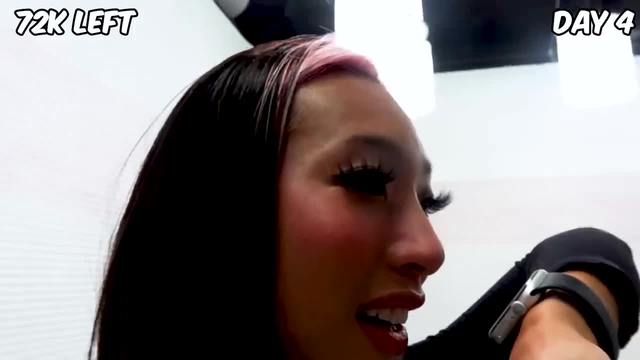 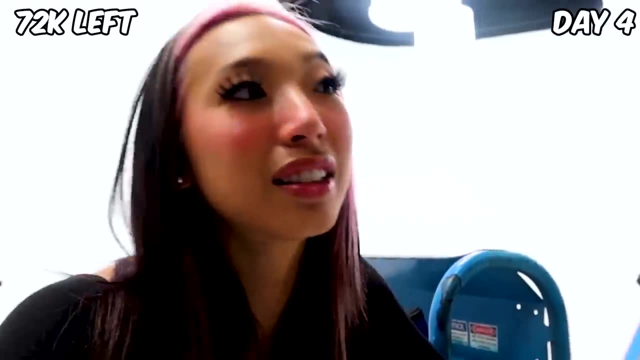 But then I had a really good idea that might actually save me. I asked Siri to call Jake for help using my watch. Hey, Siri, Call Jake Riley. It worked, it worked, it worked. Hello, Are you almost here yet? 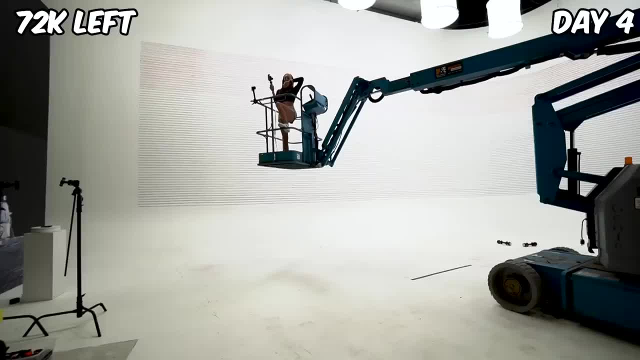 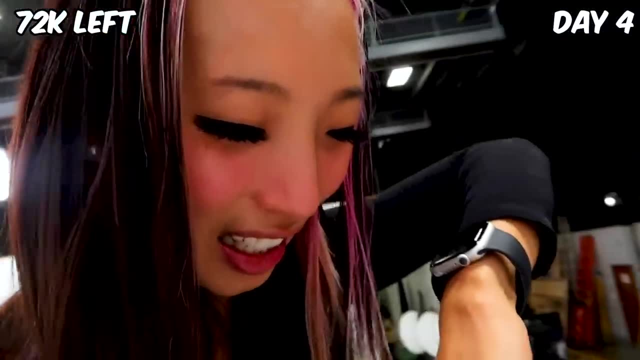 You're 30 minutes away. Okay, The lift broke. Yeah, and I'm stuck. It ran out of battery. I need you to help me get down, Okay. okay, He'll be here in 30 minutes, Even though it's only been a couple minutes. 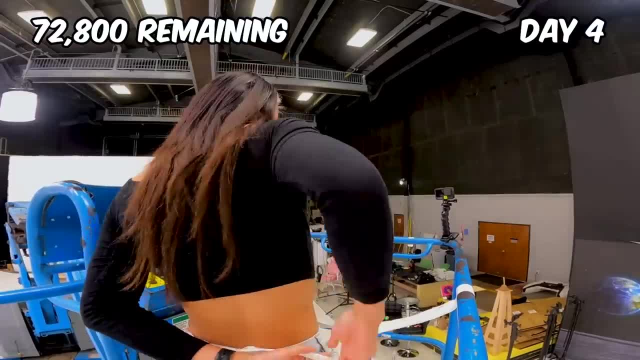 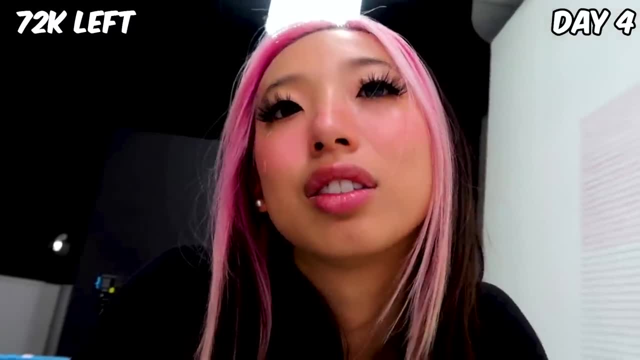 it felt like I was waiting for hours. I don't have my phone, I can't do math, I can't even use the bathroom. There's literally nothing to do up here. I want to go home. This is just too much. 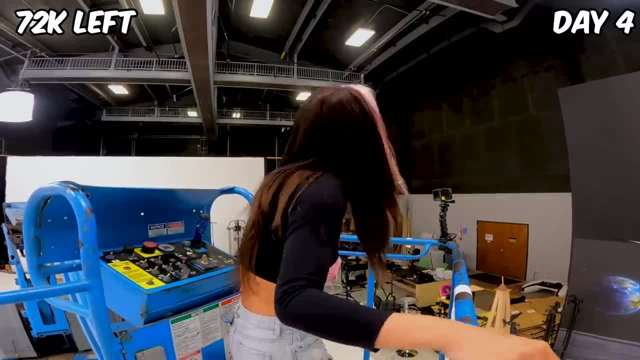 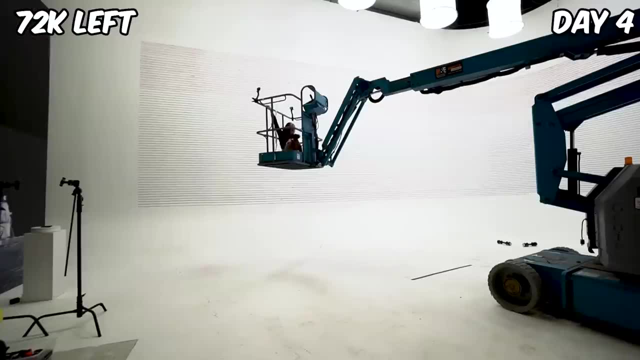 But finally I heard someone walk in: Jake, Jake. I was stuck out here for like an hour. Jake, Finally, Help me get down. Help me get down, Jake. I have to use the wash. Oh, thank God we have a long ladder. 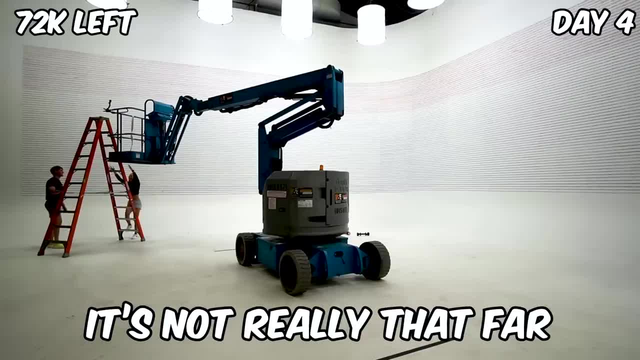 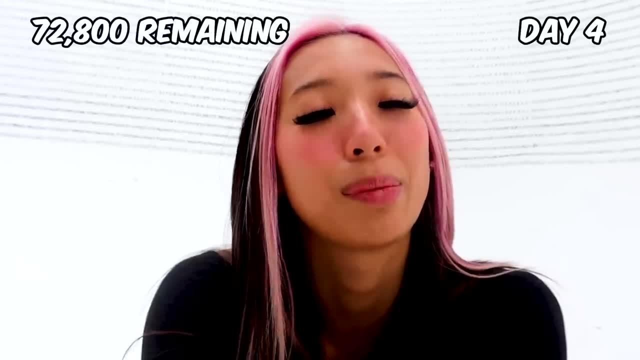 I need to call the technician. Michelle, looking from here, it's not really that far to jump. Oh, I'm just stuck up here, but now I land. I'm so happy, I'm so, so happy to be on the ground. 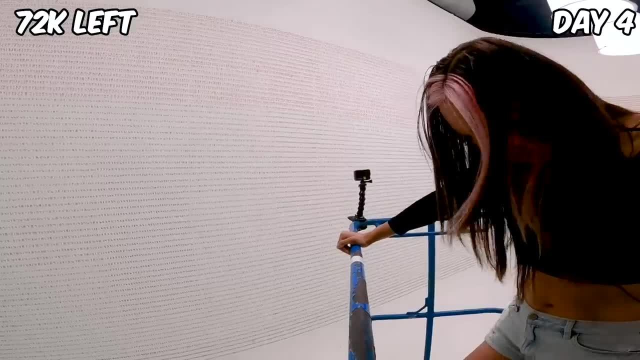 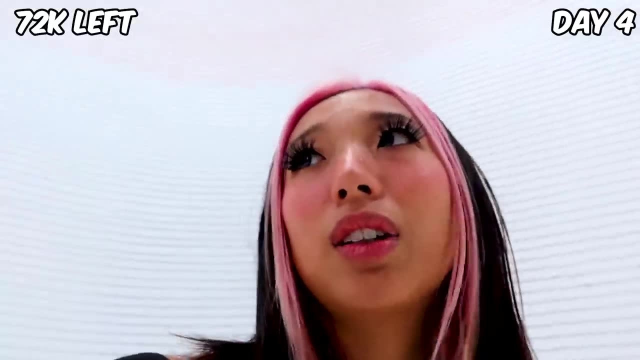 I already wasted an hour on that lift and I still have so many more digits to do today. Maybe, if I move this around, I could possibly do some math problems. The ladder didn't work. The ladder's only this tall and the math problems are all the way up there. 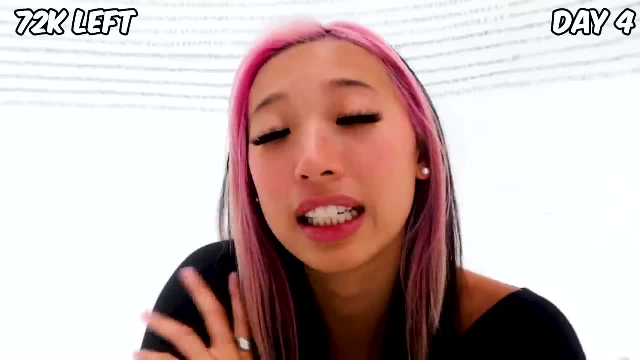 I have no idea how I'm going to finish this. The technician said that he wasn't going to be able to come for another three hours. I think what I can do, though, is work on the math problem on a piece of paper. 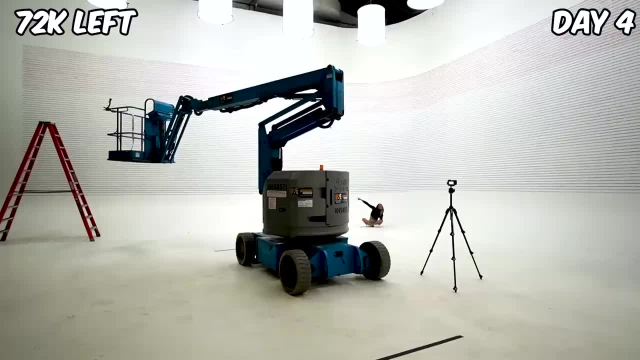 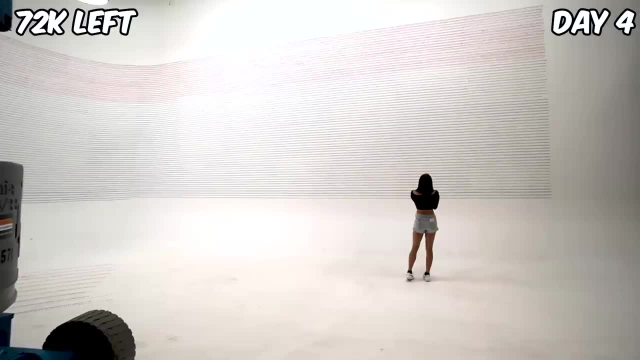 so when I finally get the lift to work, I can just copy the answers onto the wall. Okay, let's see where it left off. Four, five, five, three. Okay, Six, nine zero one, eight, one, five. 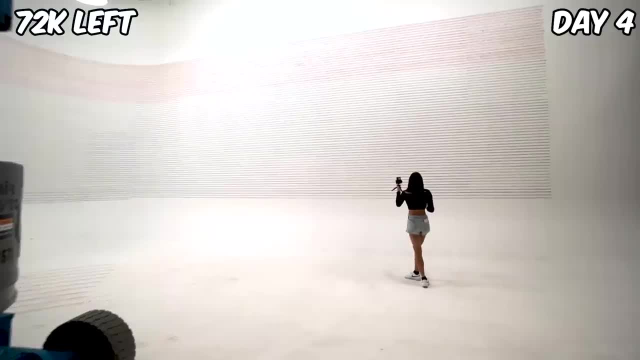 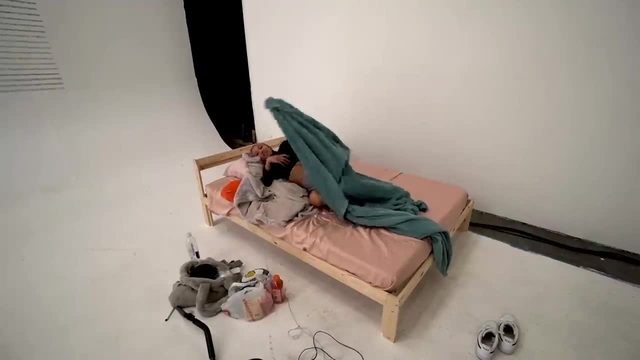 Actually, I don't think this is going to work. I looked away for one second and now I lost track of where the math problem is. Okay, plan B: Take a nap until the technician comes. Ugh, Oh no. 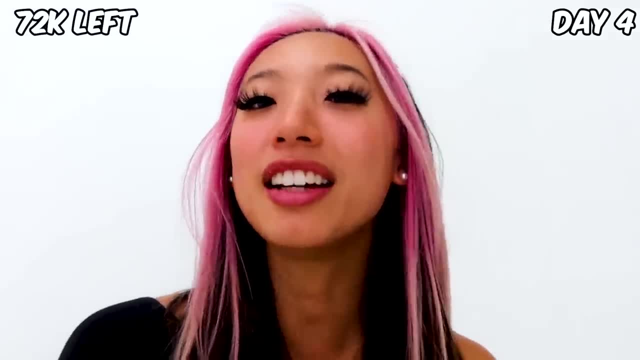 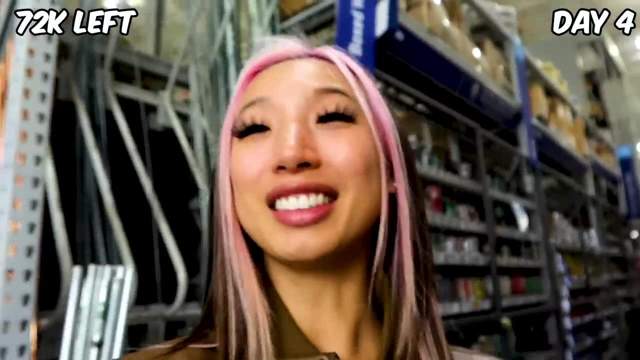 Okay. so I just found out that the people coming to help us fix the lift is not coming anymore. I don't want to spend another day waiting. I'm going to go out and fix it myself. I haven't been out of the studio in four days. 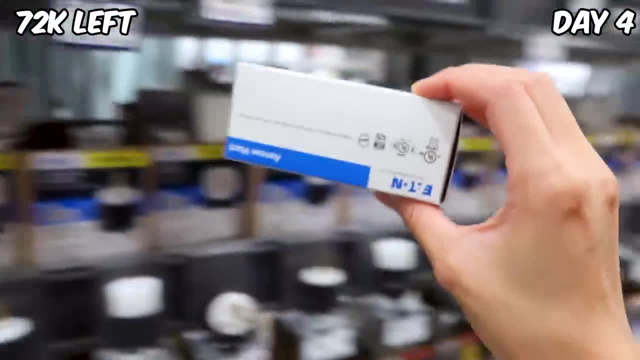 This is amazing. So we're getting this one. We don't really know anything on how to fix the lift, so I'm not sure if what we grab will actually help, But let's head back to the studio to figure it out. What do we do? 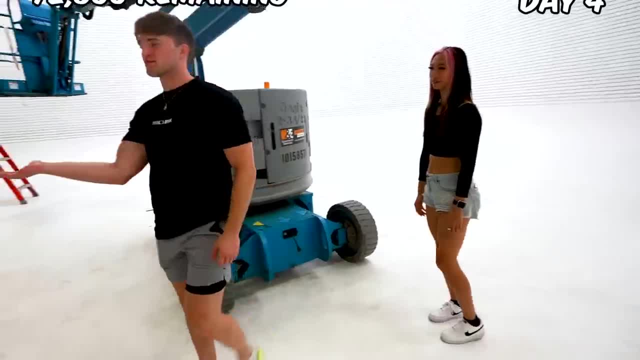 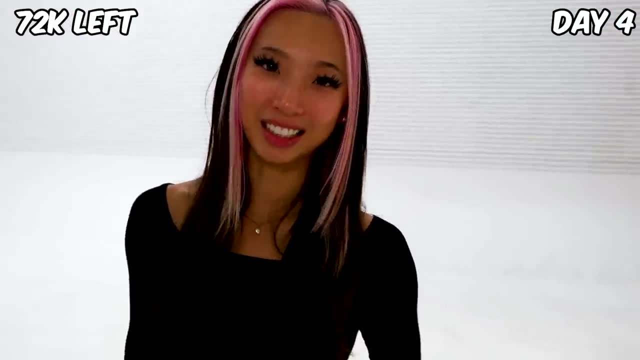 Help. What do we do? Actually, I know what to do, Flyers. First thing we do cut the giant wire. Just kidding. No, we actually have someone on our team that knows how to do it. First step is unplugging the battery. 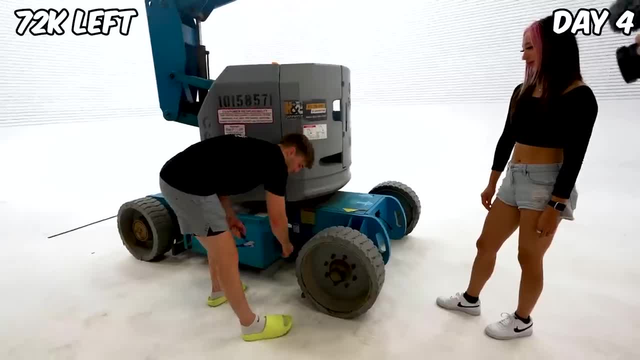 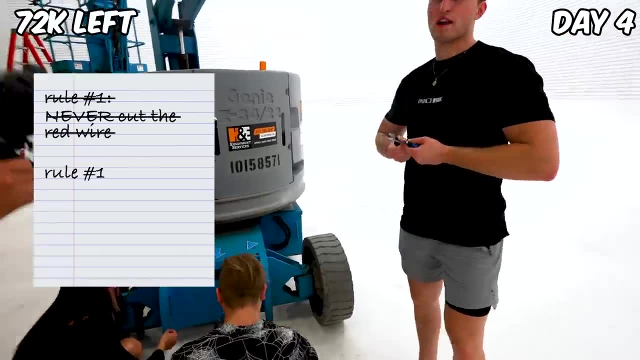 First step: take out the battery pack, obviously. Thanks, Charles. Next pliers: Rule number one: never cut the red wire. Not always true, no. Rule number one: never cut the red wires unless you have to. I want to cut Michelle's hair with this. 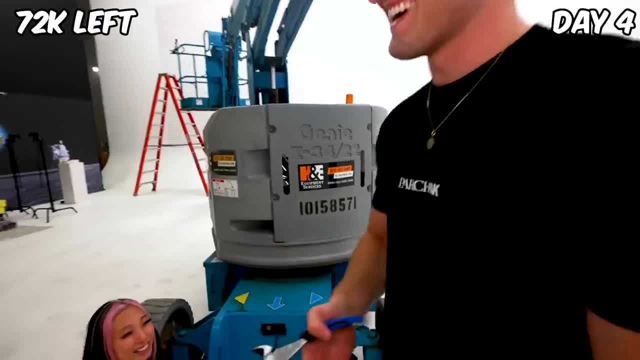 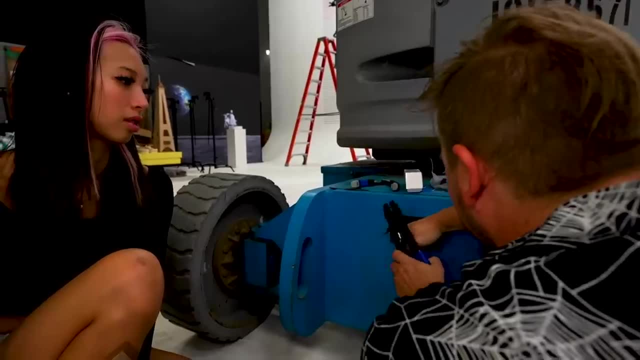 I don't need a haircut. It's been ten days, It's only been four. Next step: hand everything off to Charles. Help me fix this, because I do not want to get tased. I'm sorry, I'm about 75 hours in and I've only done 27,000 digits. 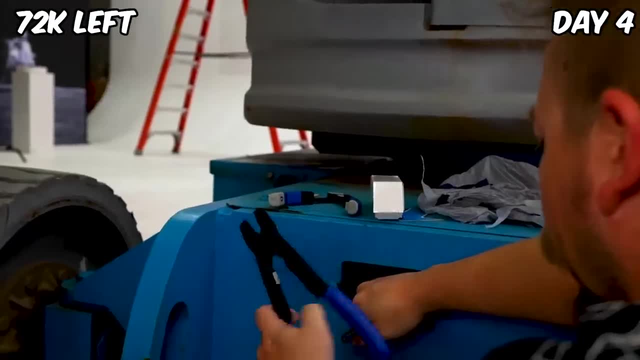 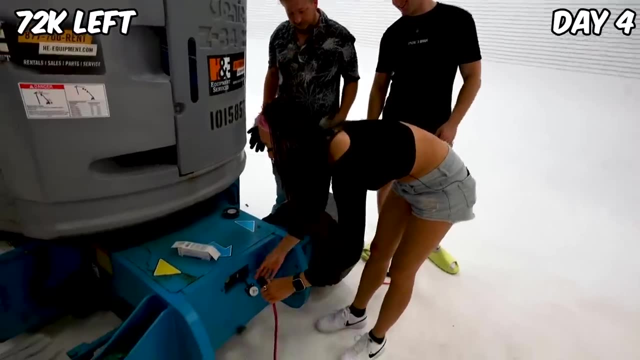 I should be around like 32,000.. Hopefully I can catch up a bit. But tomorrow I'm going to wake up early and I'm going to start on the math problem from morning till night. Let's see if it really works. 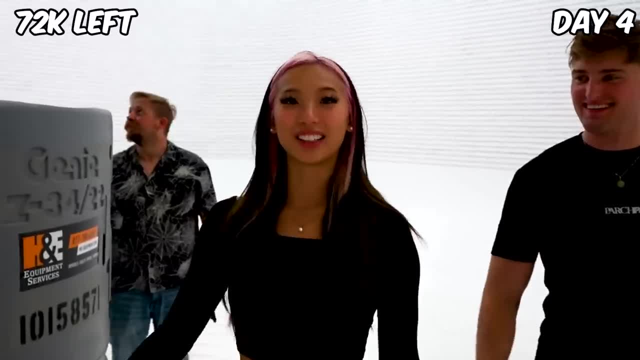 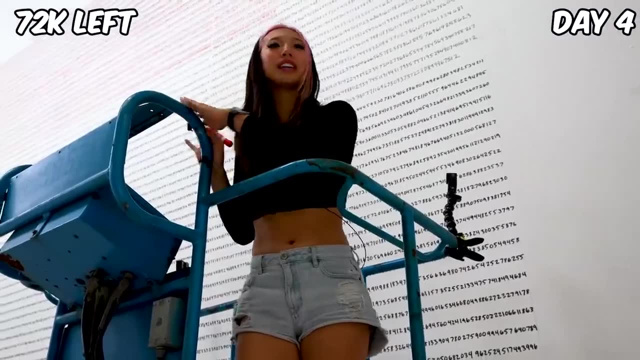 Yeah, The light is on. Time to wait for it to charge And then I can work on the math problem. I'm so glad the lift is now back to 100% and I can continue working on the math problem. Tomorrow will be a very easy day. 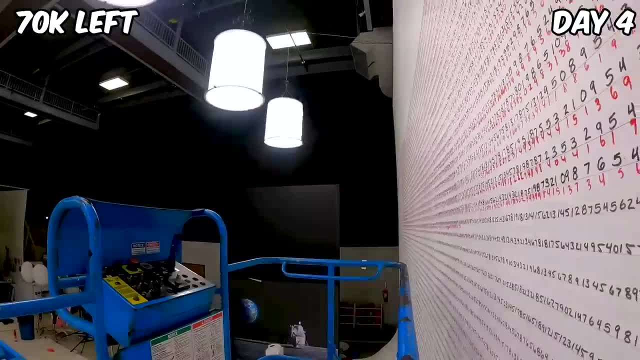 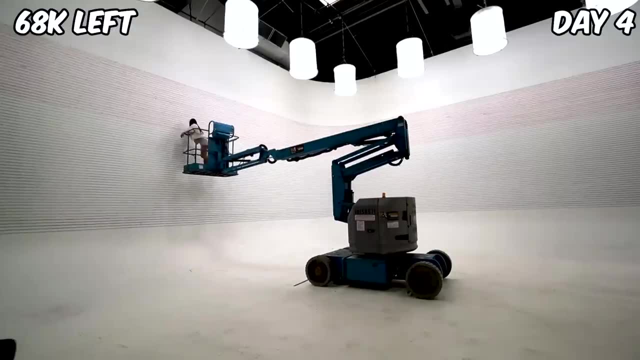 But today sucks. I hate today. I am slowly getting there. I am at 32,000 digits. If I hit 35,000 digits by tonight I'll be good to go. But I was bound to make another mistake. That puts me at 13 mistakes total now. 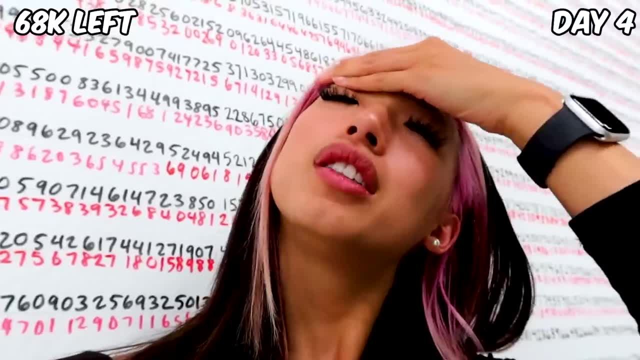 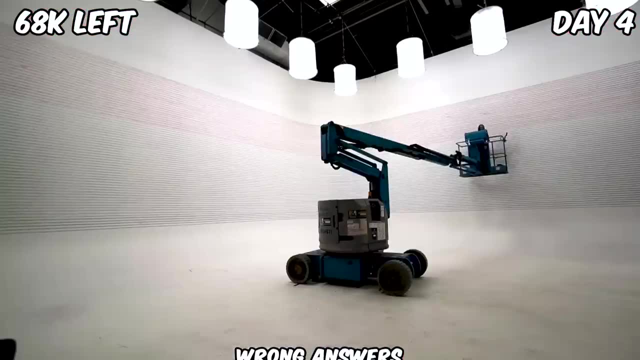 Seven, six, four. What am I doing At this point? I was making so many mistakes and, even though I'm not going to finish 35,000 digits tonight, it's more worth it to go to bed and recharge, so I don't make another mistake. 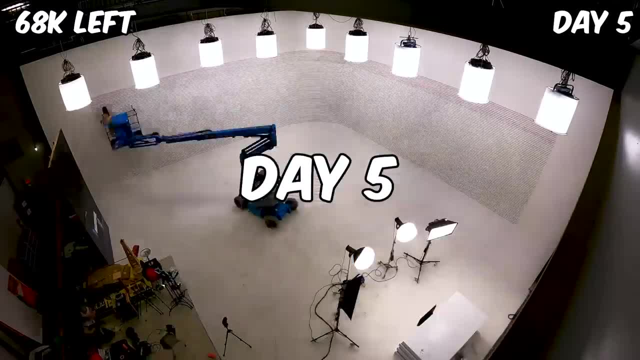 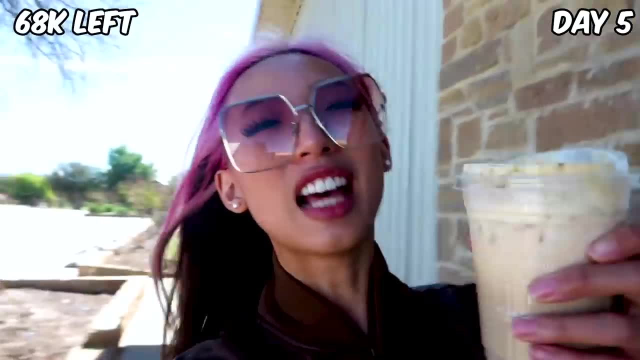 Good morning. It is day five. I woke up early so I can get a lot of work done today. First thing I'm going to do is get some Starbucks And maybe I'll go for a little hot girl walk. Just enjoy my morning before I work on this math problem all day. 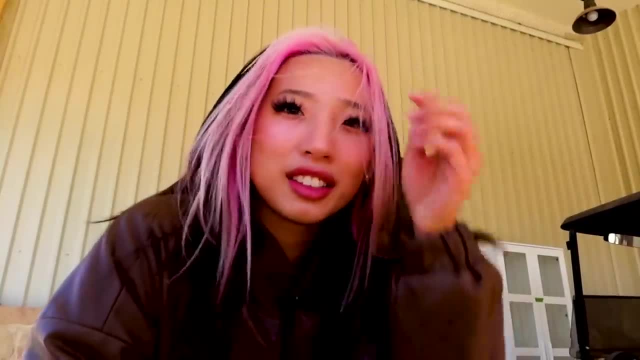 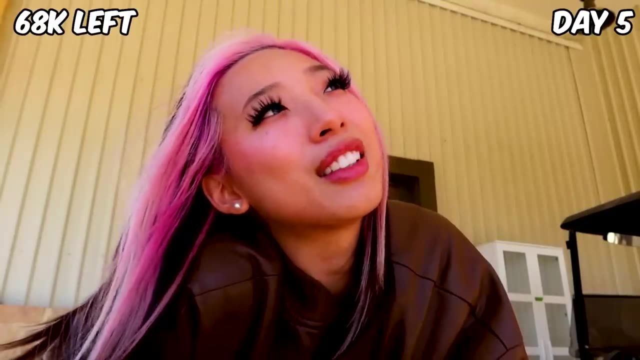 It's gorgeous outside. It's the weekend today, so none of my friends are visiting me. I feel like today is going to be a really lonely day. It feels good to relax outside, though before I start, Alright, let's get 10,000 digits done today. 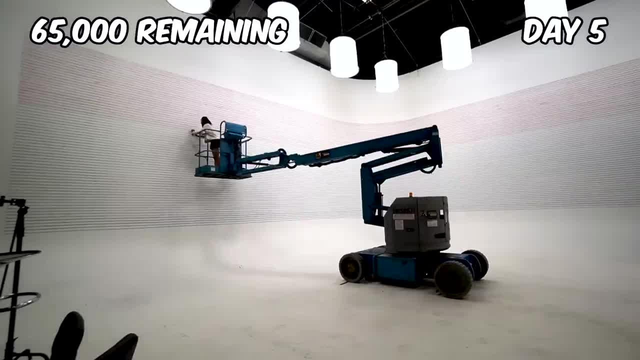 This weekend is definitely going to be tough, since I'm going to be all by myself, But it's a good thing, because the only thing I have to worry about is the math problem. I'm getting a little bit lonely. I think I'm going to call my mom. 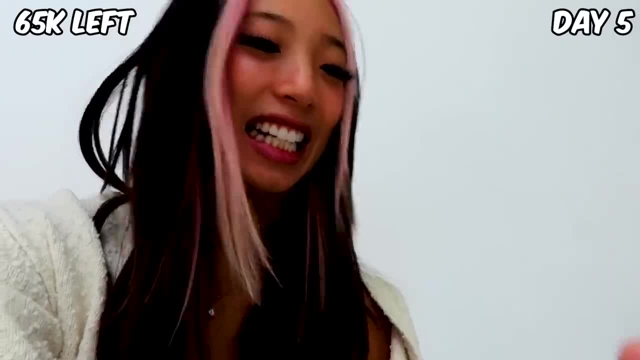 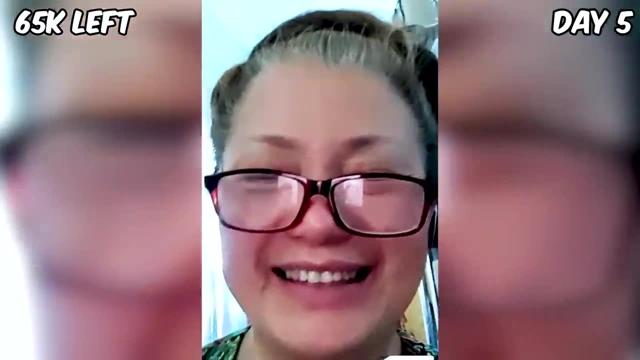 Hi Mama, Hi May, How are you? Good, Look at what I'm working on. Oh wow, Incredible. I don't know if I'll finish. You can do it. Yes, you can do it. After calling my mom, I thought it would be fun calling my friends. 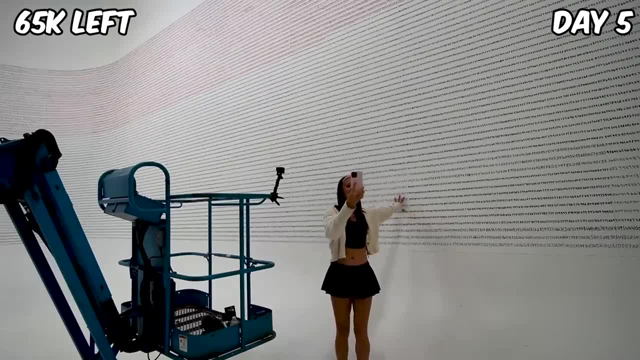 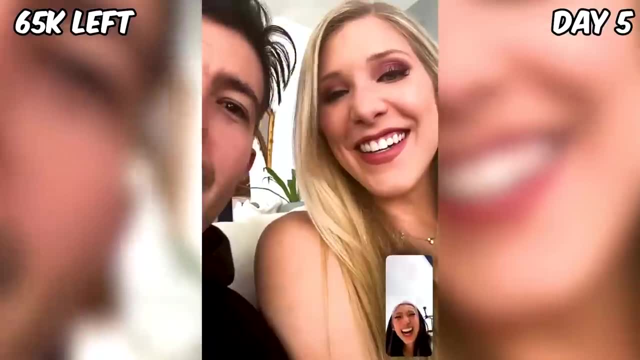 Hi, Wait, are those numbers? I am doing a 100,000-digit math problem. That's got to be fake, right? Unfortunately not. no, Do you have any words of encouragement? Stop while you're at it, Stop this madness. 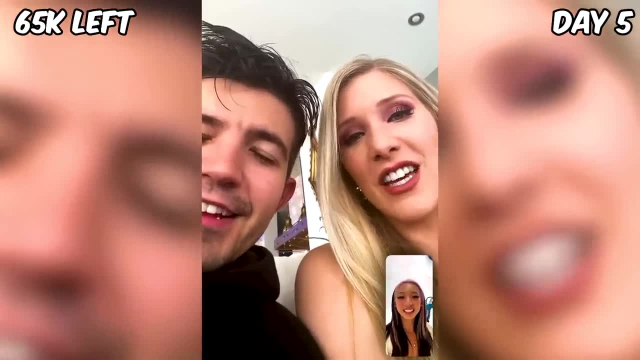 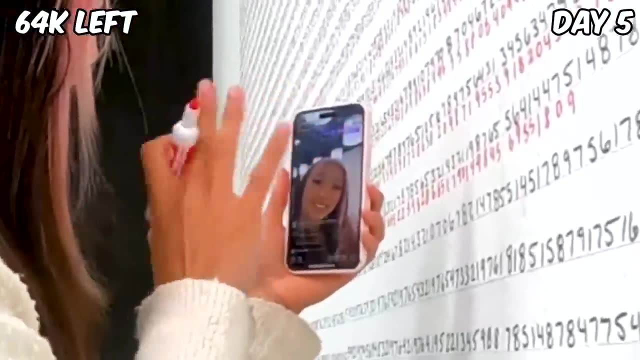 Oh my gosh. You know it's a big problem when you have a lip. Yeah, By the end of this day your hair might be gray. I still felt really lonely, so I did some livestreaming to help me keep going. 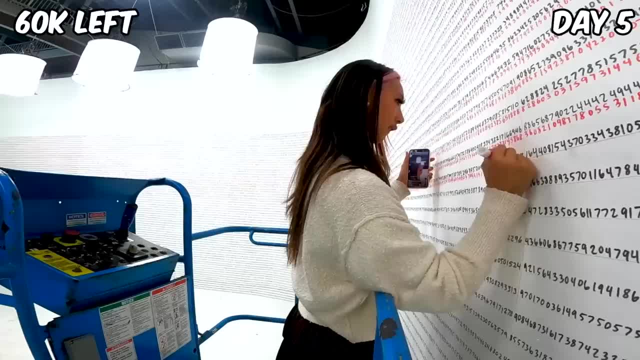 I am on, I think, 39,600 digits right now. As I was livestreaming, I heard some weird noises in the studio. I'm not sure if I was imagining it, though Did you guys hear that? I thought I heard something. 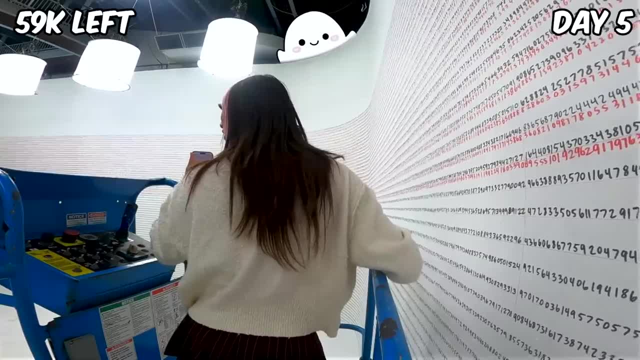 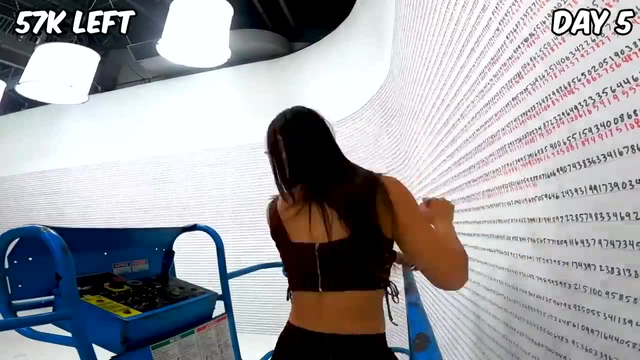 I'm the only one here. I hope it was not me. I swear I heard a voice. I don't want to look around, I'm too scared. After chatting with some people online I felt a lot better and I was able to get a lot of the math problem done. 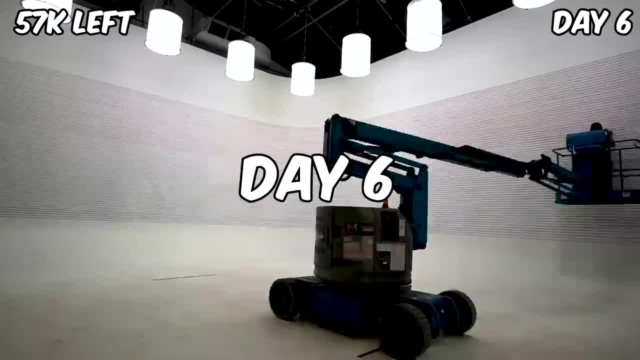 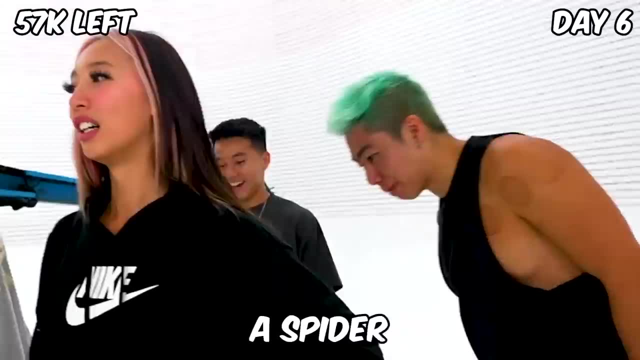 It is day six and I've been really lonely so far. Wait, Michelle, something just landed on you Where On her butt, right above her phone. Can you get it off? Can you get it off? Can you get it off? 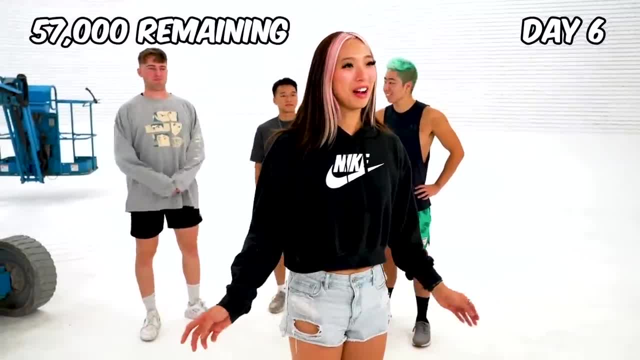 Today is day six and I've been really lonely so far. Today I have the boys with me. Hello Hi, We're the boys and we're fun. Do you guys want to come check out the wall? That is a big wall. 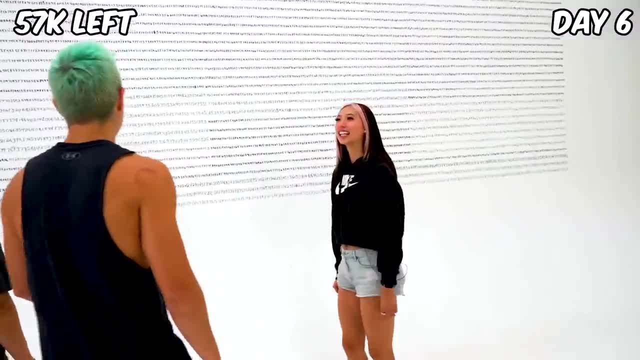 It's a lot of numbers. I think that there's not enough red. Wait, Michelle, I think you need some more numbers. This is 100,000 digits. Wait, why not a million? Wait, is this even sturdy? No, 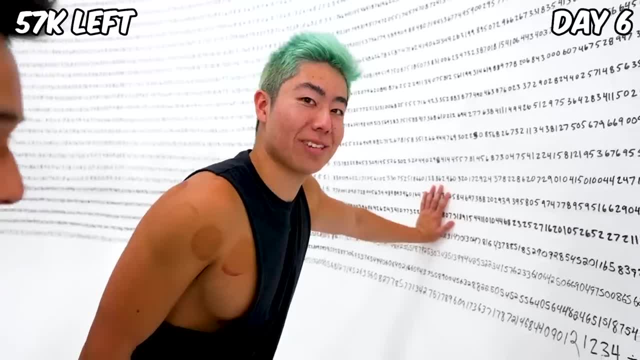 I think somewhere on this wall we hid Michelle's number. See if we can spot it and give her a call. Wait, my number's right there. Your number's right there. Wait, Jake, your number's right there. Don't give away my number. 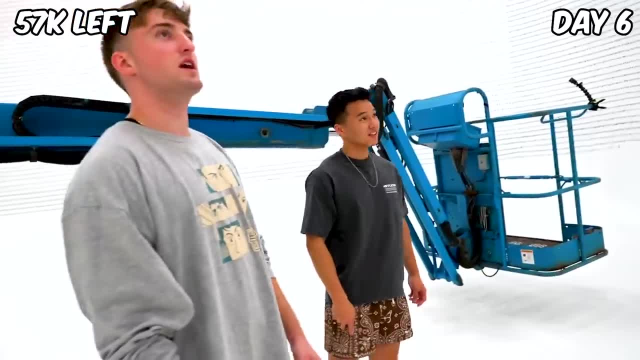 My number's right there. Can you guess how many digits I've done? 45,000.. 38,000.. 200,000? 10.. It's only a 100,000-digit math problem. Oh, this isn't the million. 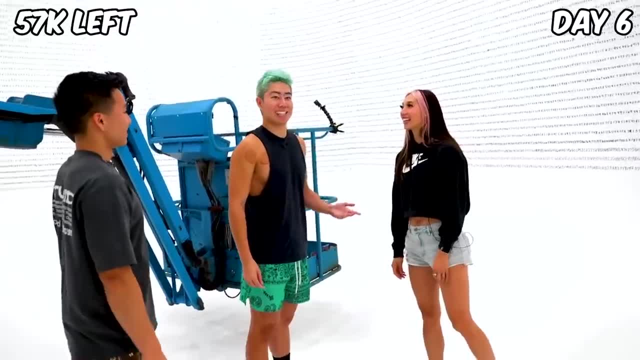 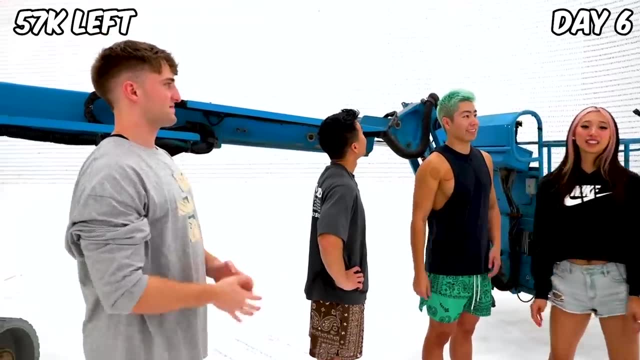 He really asked if you want to take it or double it and give it to the next. Was I right? I'm at 43,000, so Zach was the closest. Let's go. Actually, I'm really behind. I'm only at 43,000 digits. 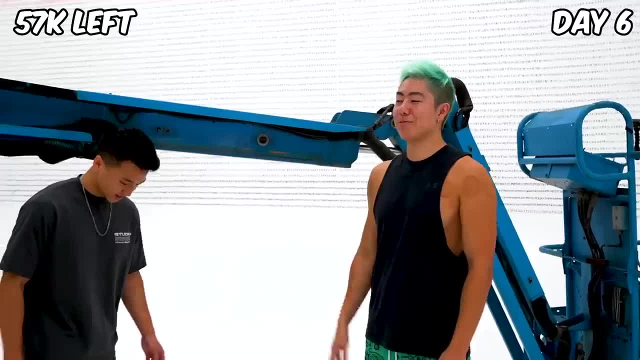 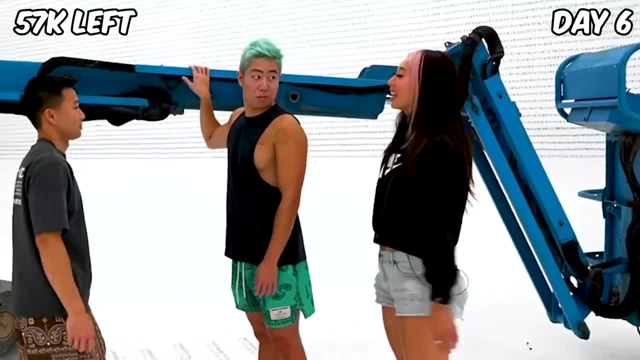 She says only 43,000, like that's not a huge number. Meanwhile, our pea brains over here Speak for yourself. All right, guys, I need some content today. Do whatever you want. Get me some good content. We can do anything we want. 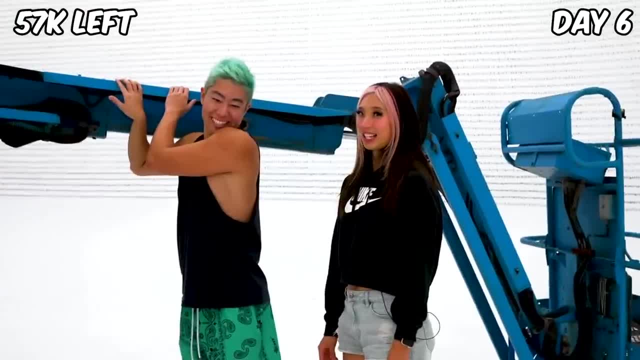 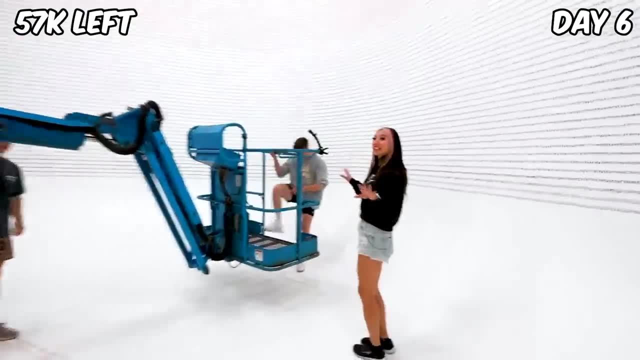 Anything you want, We can do anything. Yeah, I feel like I'm going to regret this. Did you hear that voice? Yeah, I heard it. We can do anything. I want to use this again. Anything, At least, let me work a little bit. 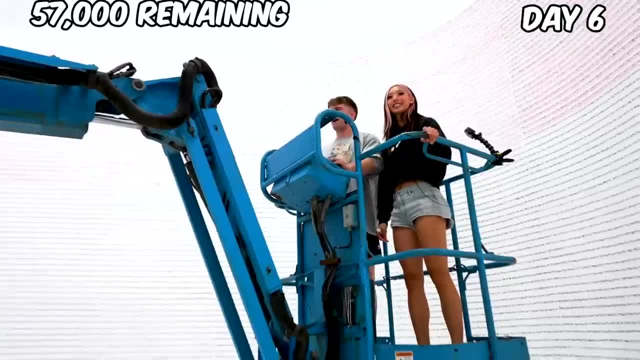 Michelle said we can do anything. We can literally do anything. We're going to have some fun here. How high does this go? It feels so nice to have the boys' company again, but I feel like I'm going to regret saying that they can do anything. 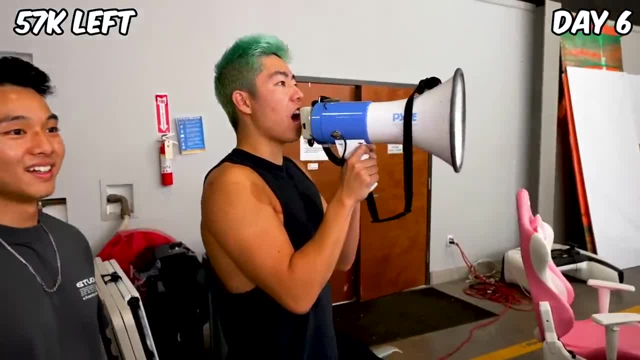 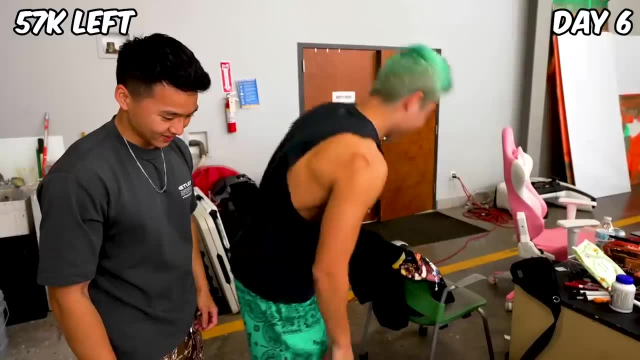 Put this back down. Hey, Hands off, Go, Michelle. That's enough. That's enough. That's enough. All right, we'll just leave it here. That's enough. Wait, how high does this go? And not long after things started to get pretty crazy. 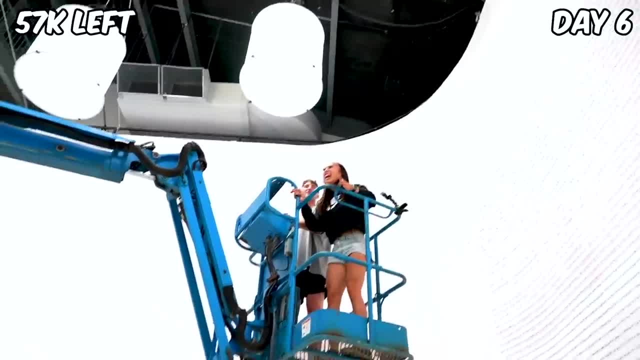 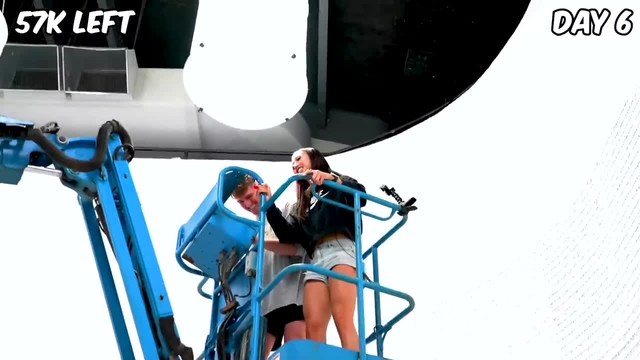 No, No, No, But you were working up here before. Take me down, Down, Down, Down Down. Don't touch that one, Don't touch that one. What about this one? We have, Michelle. Oh, we have to go up. 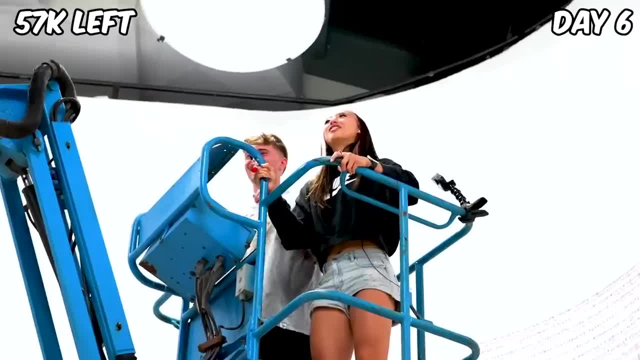 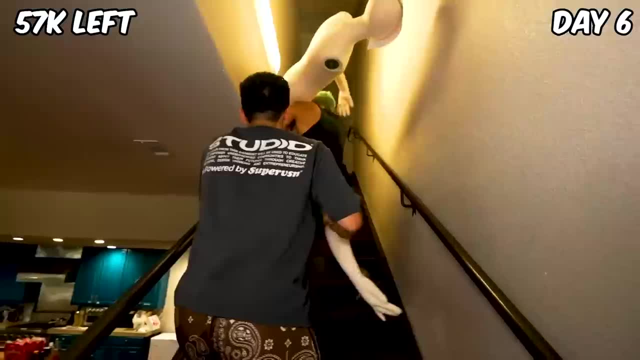 No, Michelle's about to say hello to the other. Michelle, We're really high up. Help me out here, Ben, I can wait. Actually, I got her arm, Sam, Turn it off. Turn it off. Hey, you're right. 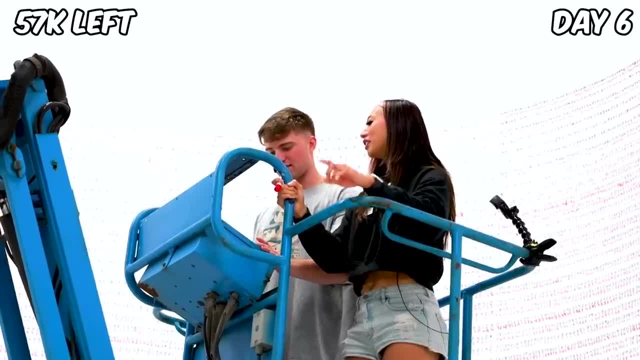 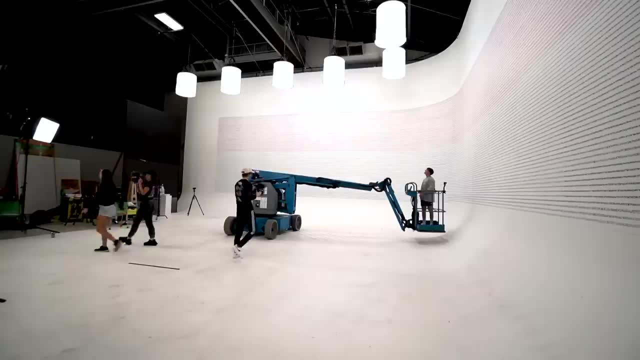 Keep listening, Wait, what are you doing? What turns us? No, no, no, This one. Wait, go this way. How much do you think I could sell Michelle's arm for on eBay? At least 20 bucks. I just really thought everything was starting to calm down. 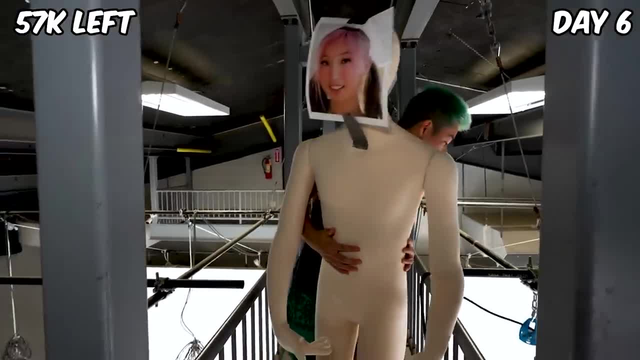 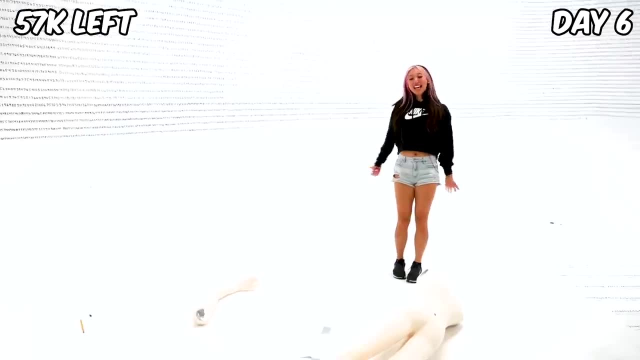 Hey, Michelle, It started getting crazier. We found another version of you Calculator human. Michelle. That is so good. You amputated my limb. Why would you treat me like this? I'm trying to work, Yo Oh. 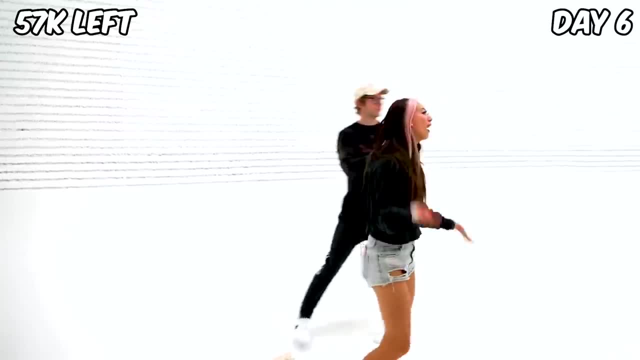 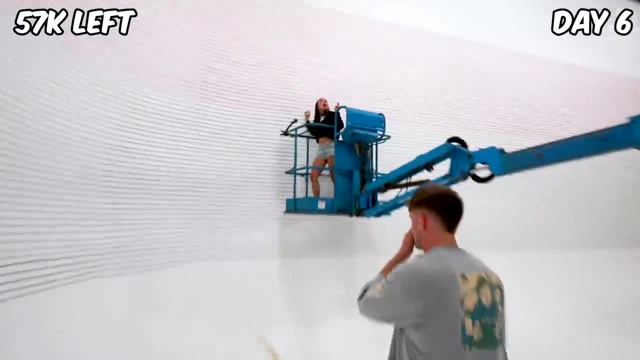 I got it. Woo Ben, high five And crazier. Michelle, I heard you did a Lego video earlier. I got some for you. Sam Whoa, That was sick. How am I supposed to work? Oh, Oh. 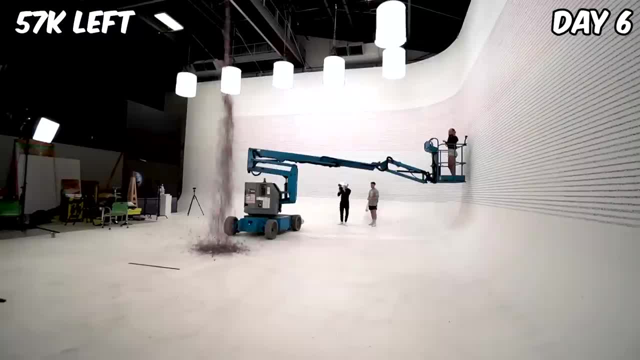 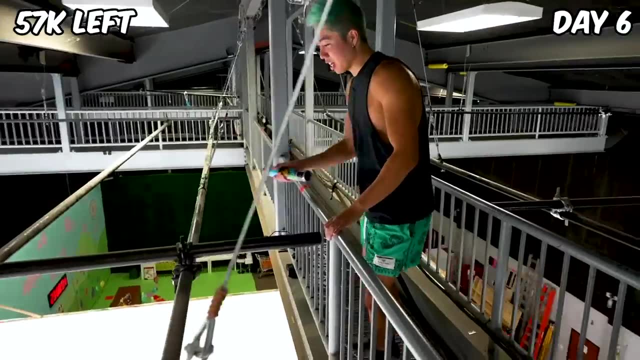 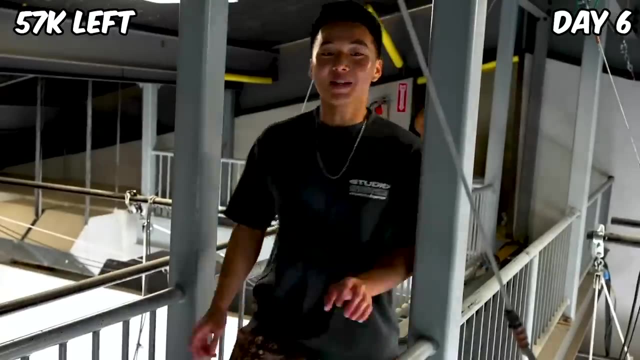 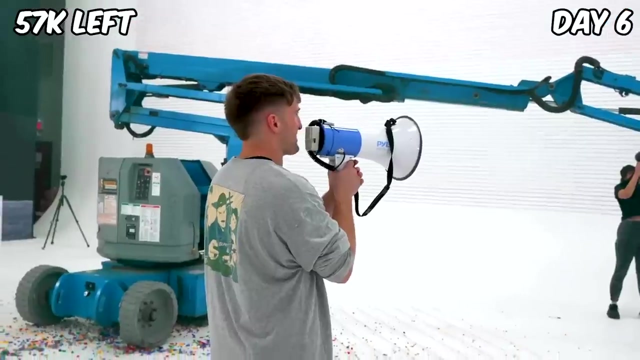 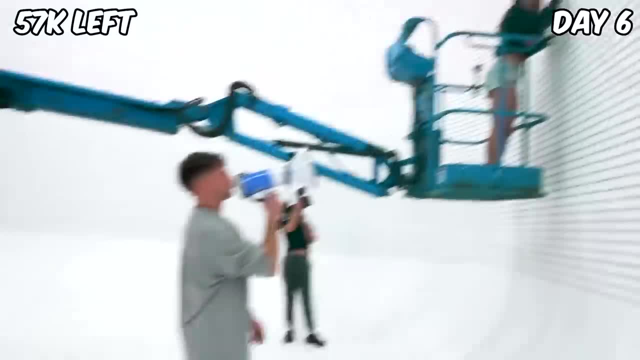 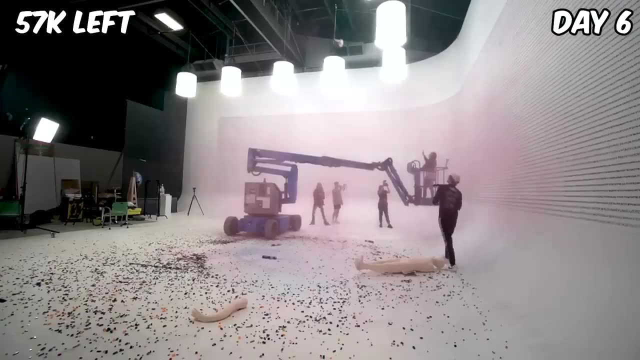 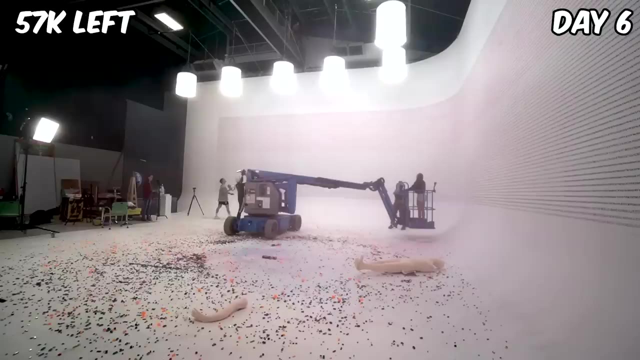 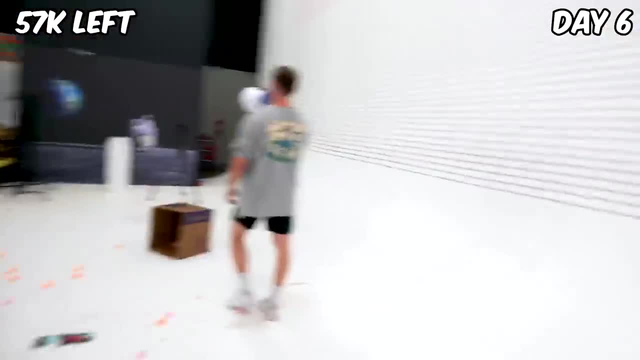 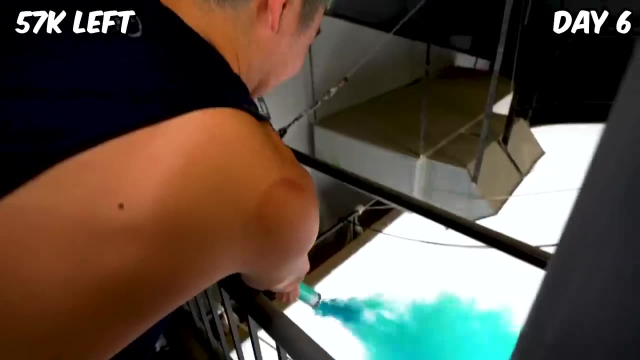 What am I supposed to do? We don't need this anymore. I can't even move the lift. All right, All right, guys, I take it back. Calm down. There was a rogue math user on the loose, Oh. 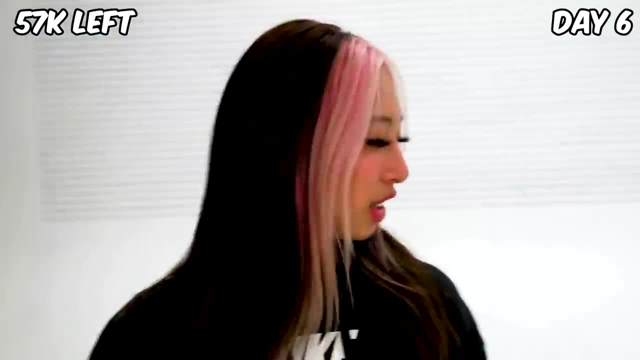 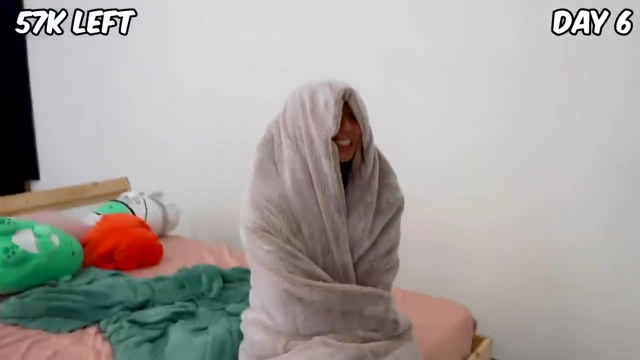 Help, Help. Oh You're kidding, Oh, my god, You're joking. I couldn't tell the boys to stop, so I just knocked off. I just decided to lie down. Stop the content. Stop the content. She's neutralized. 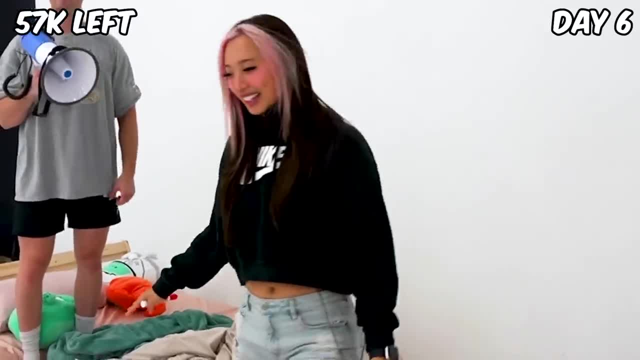 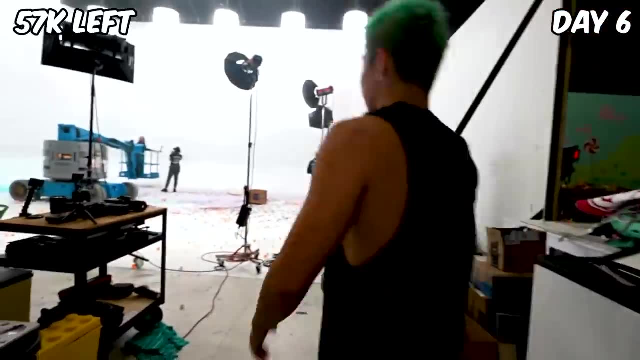 She's on her bed. I think they're done. She's in the cloak. I think they're done. I will keep going. I have a blanket in my hand In the powder. In the powder- Wait, my blanket. I need to mark my territory. 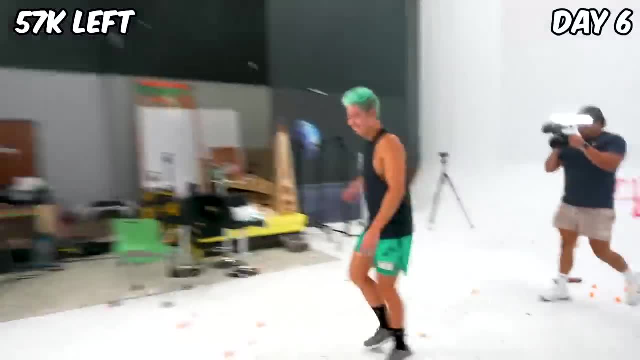 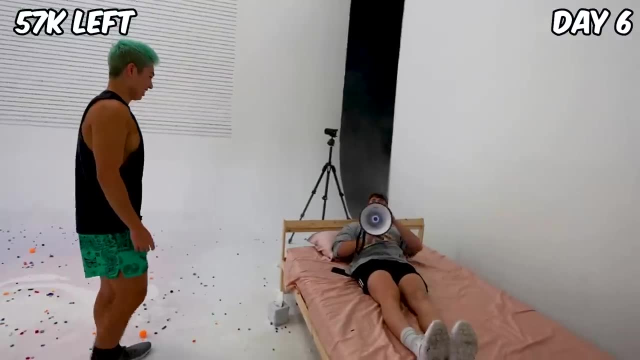 Zachary, what are you doing? Attention, Attention, Zach. I see a fire, There's a fire. I forgot the fire. The fire's put out. This is complete chaos. What the Did you fart? Who farted? 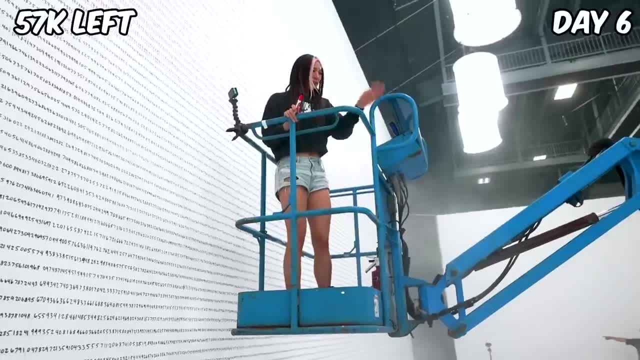 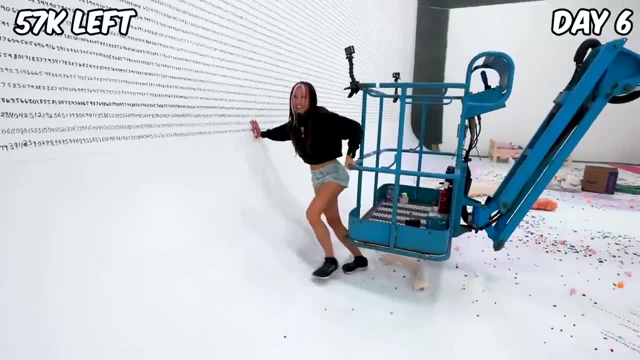 I'm tasting food At this point. I don't even know what was going on, but all the powder and smoke started to smell so bad we had to evacuate. Oh my God, I'm so sorry The boys weren't here. 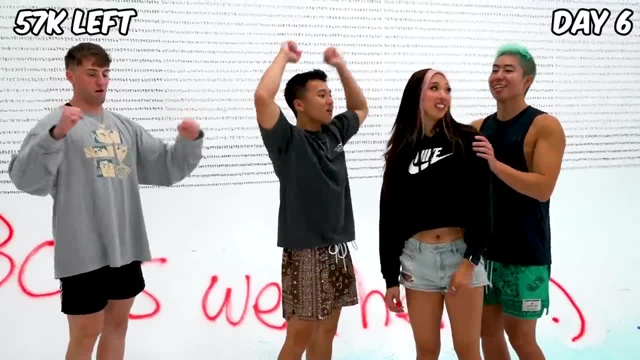 Michelle, Michelle, Michelle, Let's go. I'm taught Who's going to clean this up. I thought you were cleaning it up, Don't we have to be somewhere right now? Wait, Jake, were you going to clean the door? 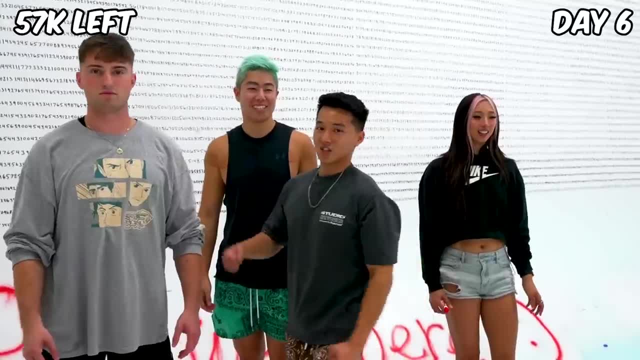 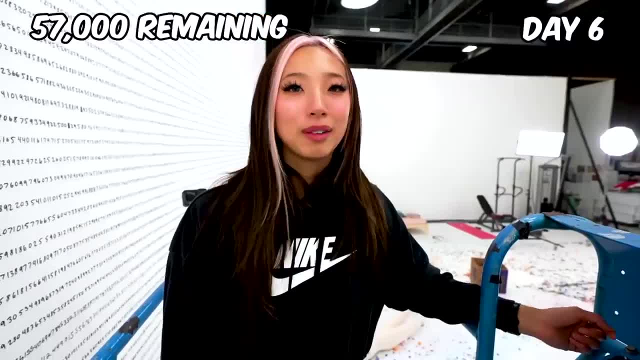 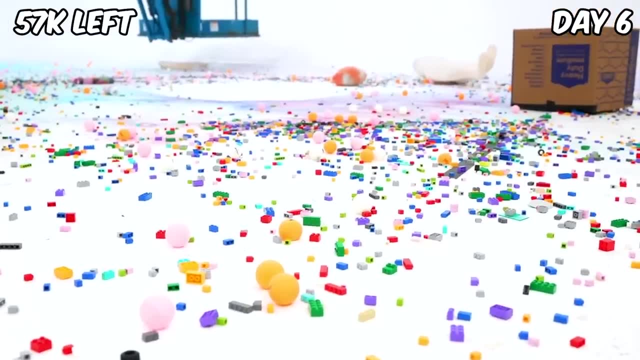 I'm going to go get a broom. I'm going to go get a broom. I didn't know what I was expecting, but I was definitely not expecting this. Look at this. It's a mess. The Legos made a complete mess. 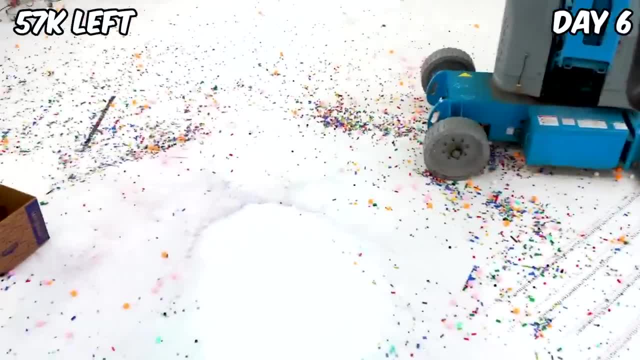 I mean, I can't even move the lift right now because it's all over the floor. The worst thing, though, was the powder poppers and the fire extinguishers. They both smelled so bad. Oh, actually, the worst part was when they threw the blanket on the ground. 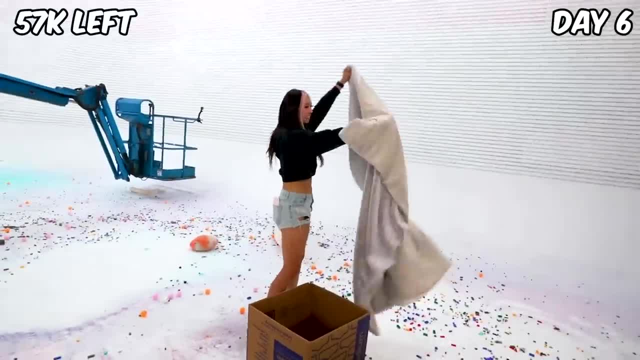 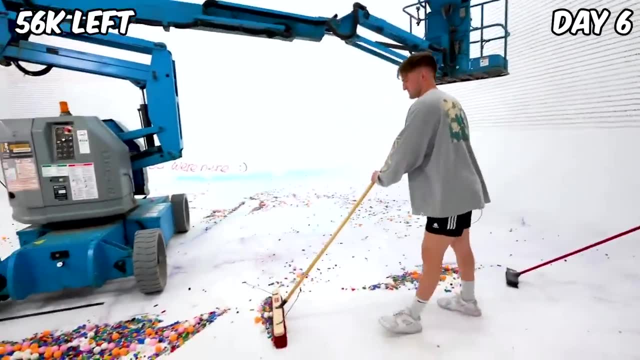 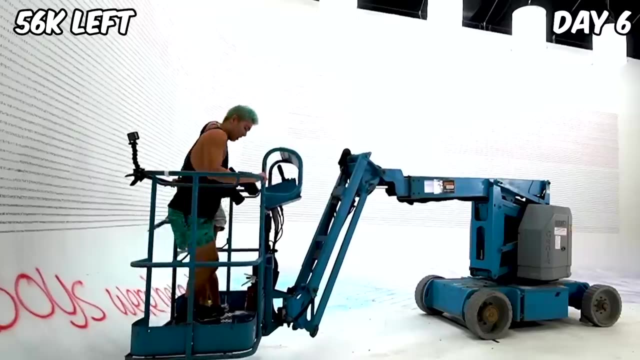 That was my favorite blanket. I should not have told them that they could do anything they want. I did miss them. Now I don't miss them as much. Hello, Can I join you? Yeah, After that disaster, I think Zach felt a little bad for me, so he decided to come up to the. 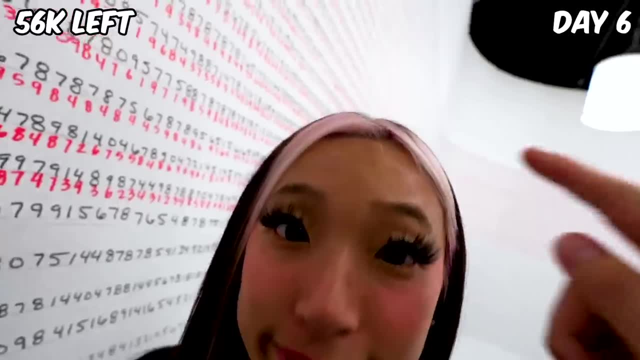 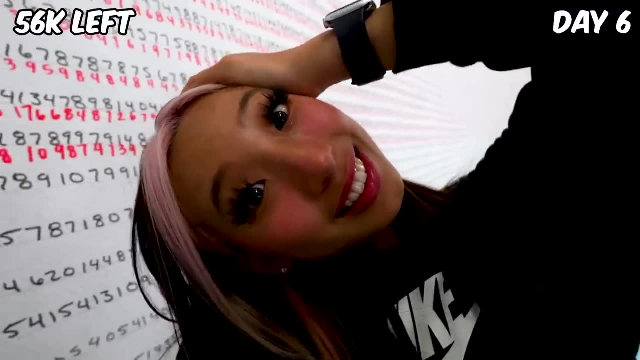 lift to cheer me up. Okay, so this is Michelle's POV. What's going on in here? It's a big mess. There's a fire. I see a lot of comments asking if you're a robot. I am not a robot. 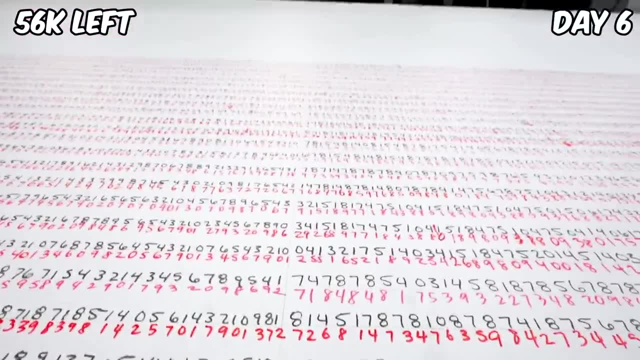 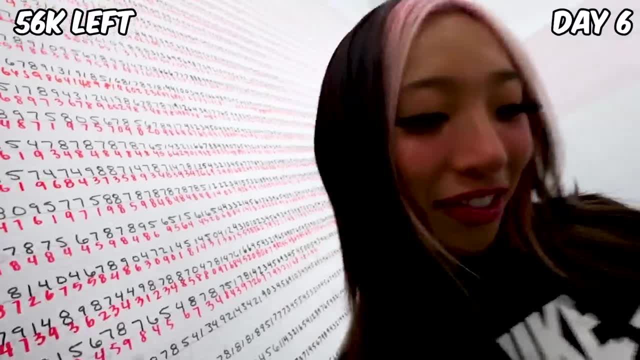 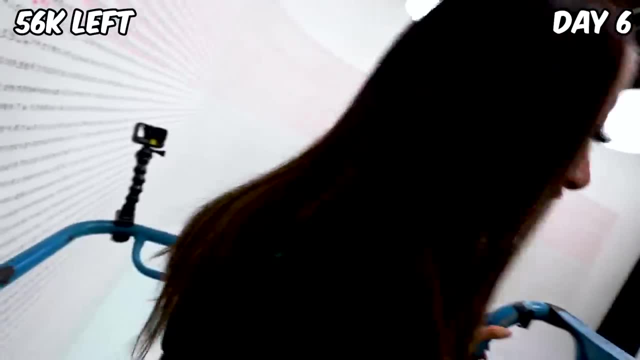 My girlfriend's beautiful and smart. Oh, you're so sweet. Let's go for a ride. Come on, It's scary. Oh, we almost hit the wall, Michael, Isn't it fun? Oh ow, Michael, I'm a good driver. 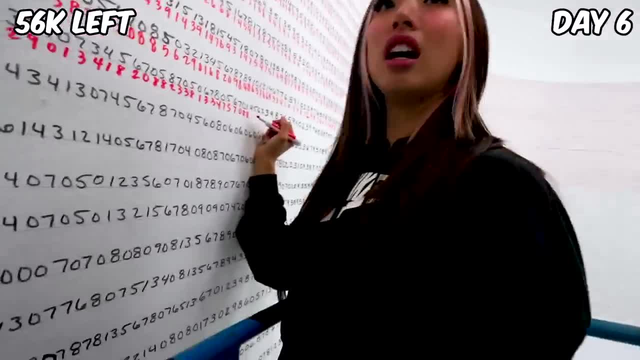 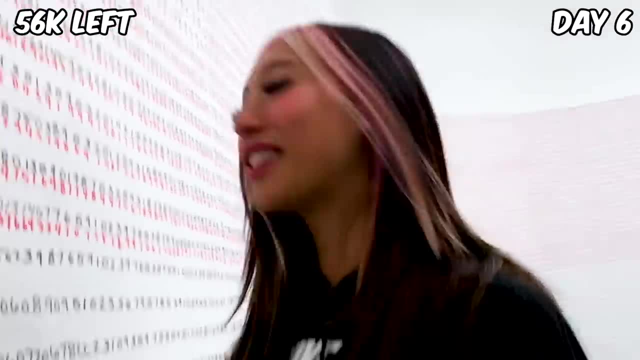 They also say, Oh oh, I got it wrong. Uh-oh, Oh oh, They hit 50 mistakes. They have to restart the whole thing. Oh yeah, I thought of that, I know. Lower it, Lower it. 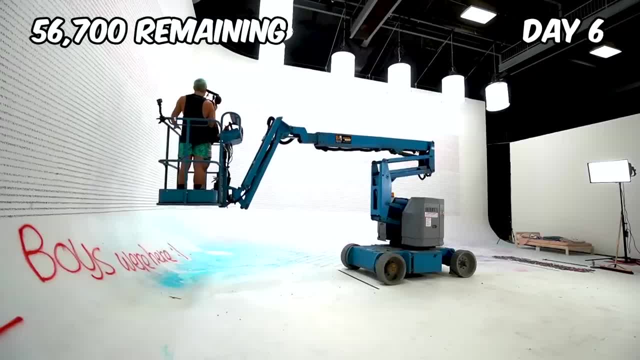 I want to get out. Don't give me that, Michael. this is Don't go. Oh, go down. There you go. Did you notice it's much harder to make them win convincingly? Before Zach left, he surprised me with one more gift. 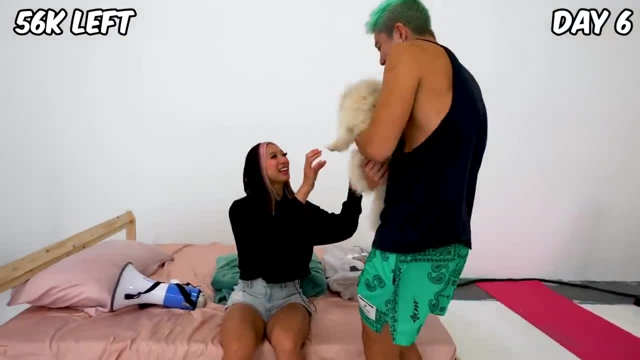 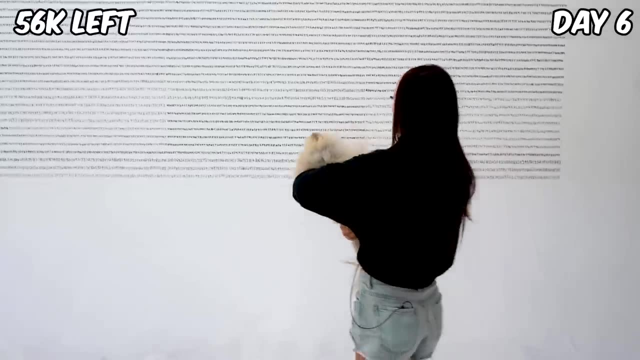 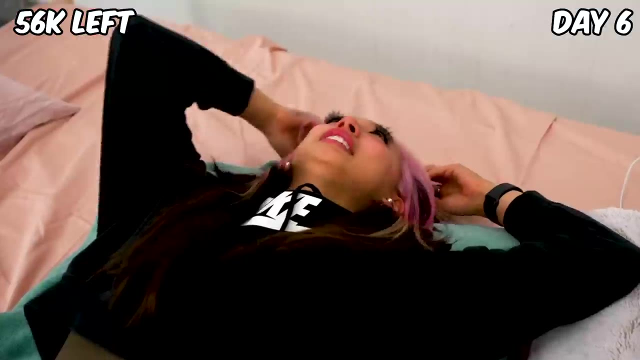 Aw, My baby, I miss you so much. I'm so excited to see you. You're so cute. This is what mommy's been working on. What do you think? Do you think you can solve this? This has made me miss my home so much. 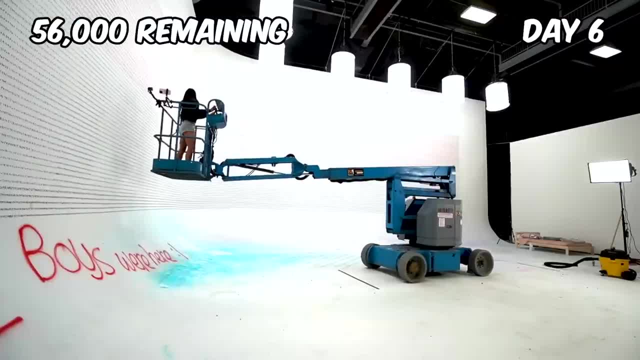 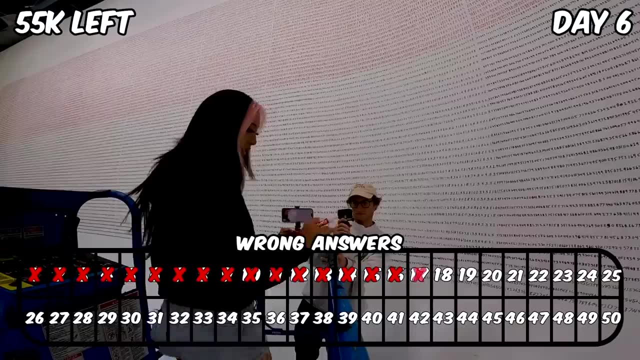 I need to finish this ASAP. Did you see that? I almost crashed it? I justέλtea 17. Five, not three. Okay, so Jake's gonna check my answers. Oh my god, she's going too fast. 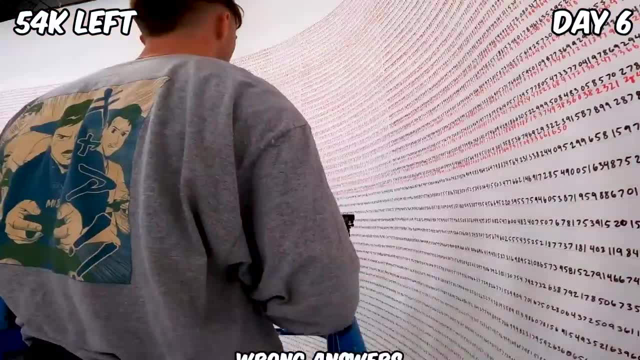 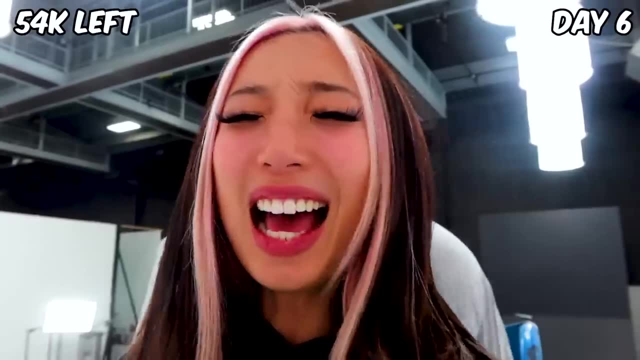 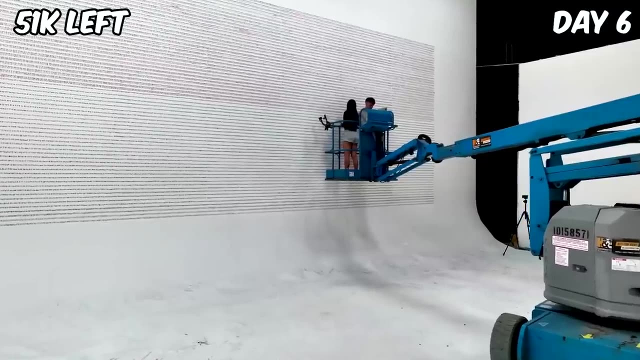 Oh man, I made a mistake. Yeah, it's wrong. Michelle found out. she made a mistake before me and I'm checking my answers. This is not a zero, It is a two. So I'm currently at 18 mistakes. I am at 48,000 digits. I really want to hit at least 55,000 by tonight. So that means I have. 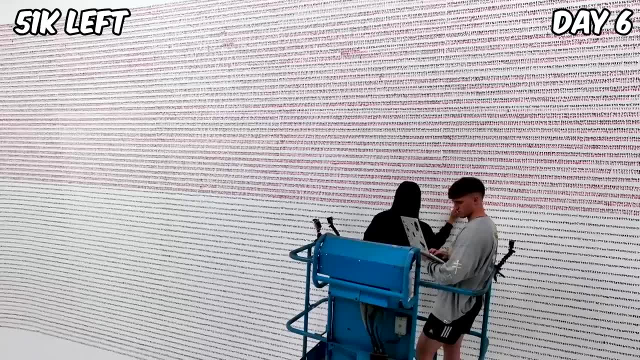 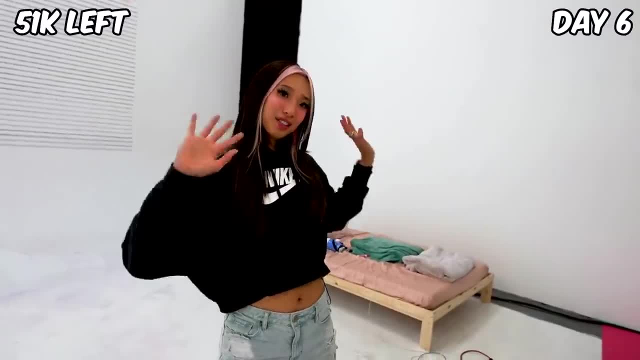 to work all night. Oh, I'm so tired. I'm gonna go on TikTok live, Maybe the chat will keep me company. And I'm really excited for tomorrow because I'm gonna get some things for my little room so I can feel more like home. Hi, Over 4,000 people watching me do math- Kind of scary, but 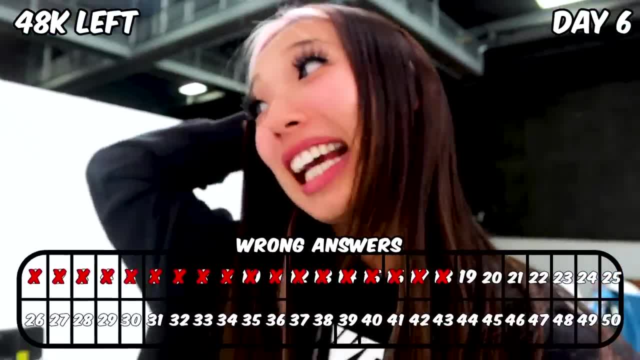 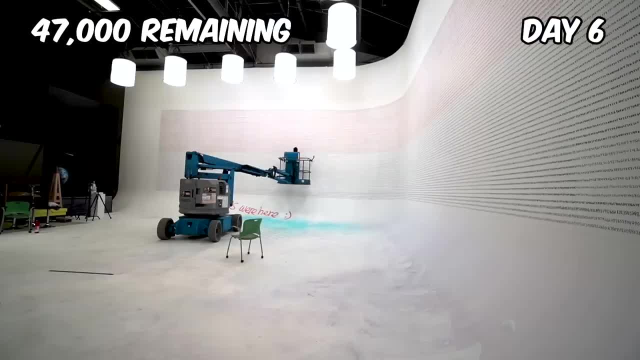 super cool. Oh, I made a mistake and I did it on live, which is super embarrassing. Nine, three, four, six, one one. I don't know what's happening, but I think I'm going a little bit too fast. 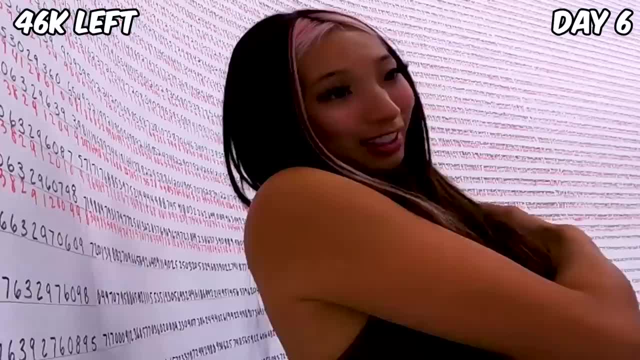 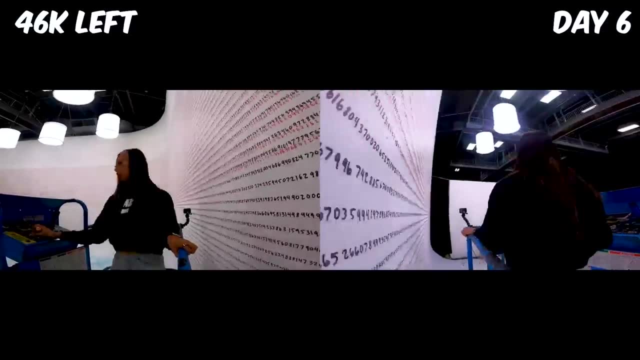 This is a seven: 20 mistakes. I think I'm gonna end my life. Thank you guys for watching. Oh, mistake number 21.. It's supposed to be a seven. Getting a lot of mistakes today. Maybe the more math I do and as the more days go on, it's harder for me to concentrate. 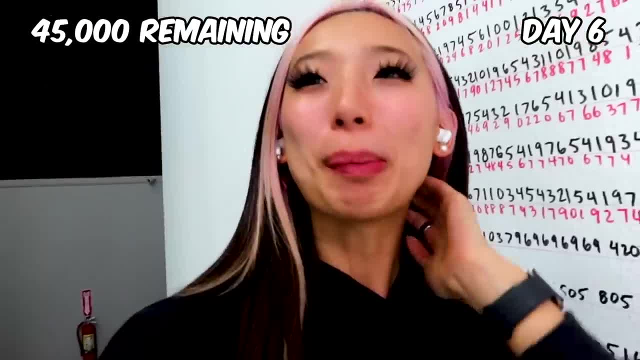 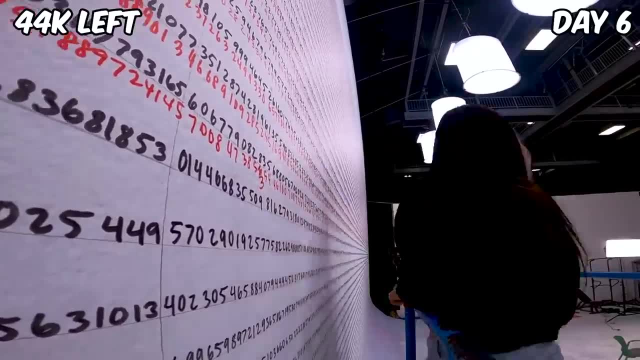 All right, I officially hit 55,000 digits, Super proud of myself. No, I'm starting to realize that working late is probably not the best idea, because that's when I start making the most mistakes. No, I made another mistake. It is not a six to three. 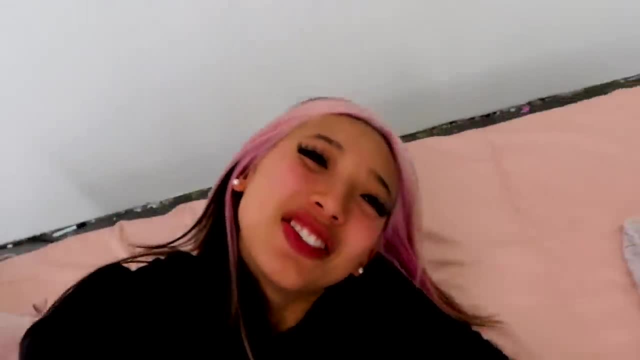 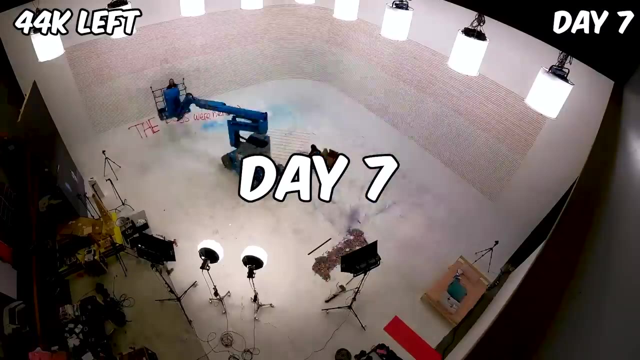 I'm at 23 mistakes, It is late and it's finally time for bed. Good morning, It is day seven and I'm tired. Yesterday I said I wanted to decorate the set to look like my home. Let's go shopping. The reason: 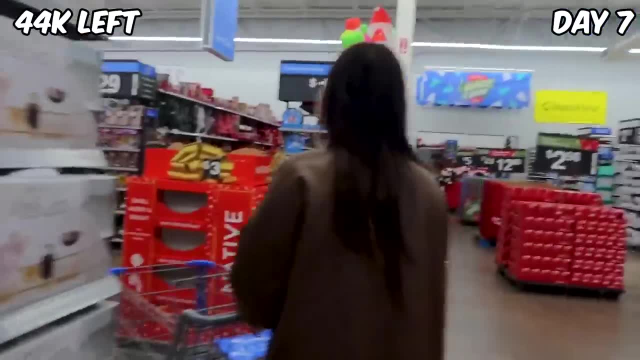 I'm doing this is because I haven't been home in a very long time. I really miss Zach and the dog, so I'm gonna go out and buy things to recreate a home. we feel I got things that I have in my house. 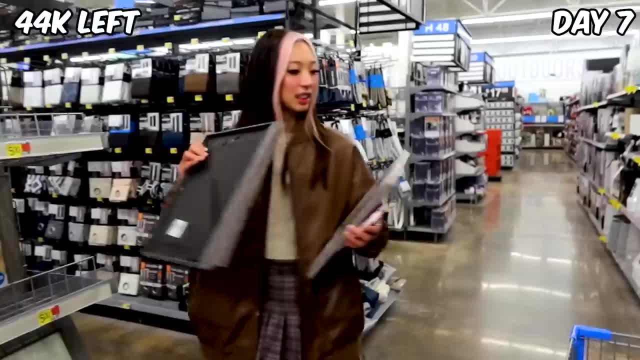 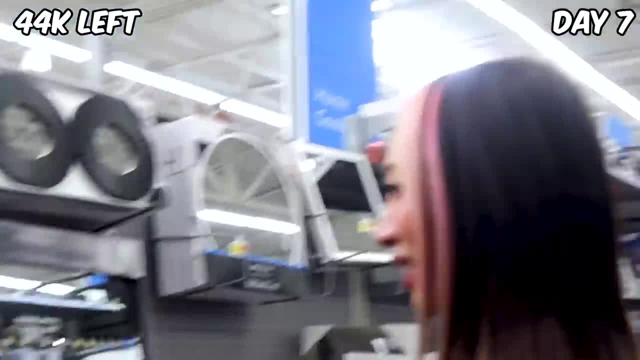 like a blanket, a rug- It's good to be home- And some plants. Let's go. This is so fluffy and cute. Your mirror might be kind of scary. What if I wake up in the middle of the night and I look at myself and I scare myself? 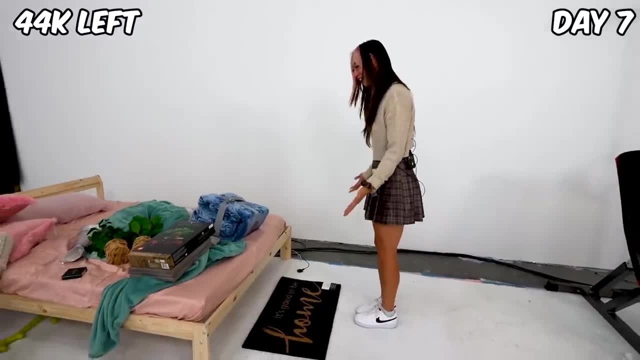 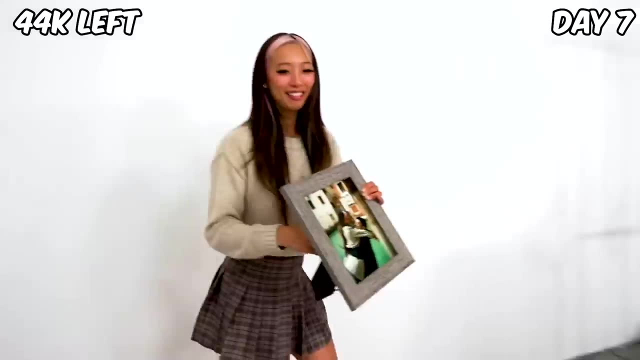 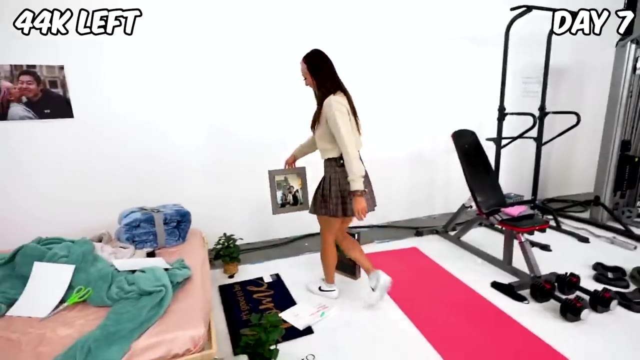 Shopping is a success. Let's decorate. It's good to be home. Where do rugs even go? Oh, perfect, Perfect. Too much Right here. Maybe just two is enough. No, I need one more. Ta-dah, Right here, Ta-dah. 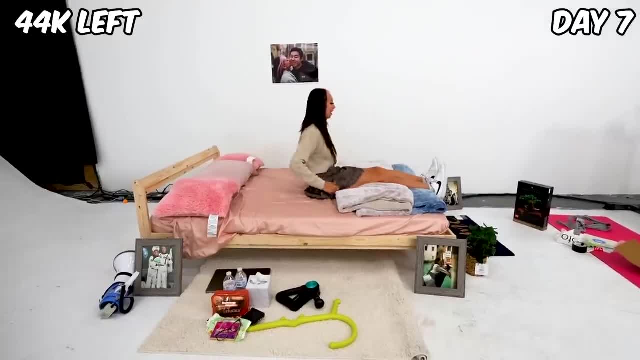 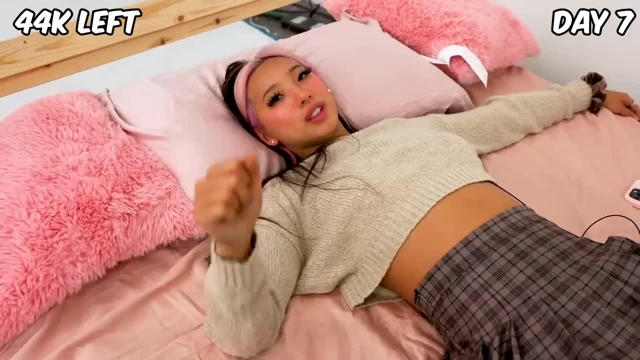 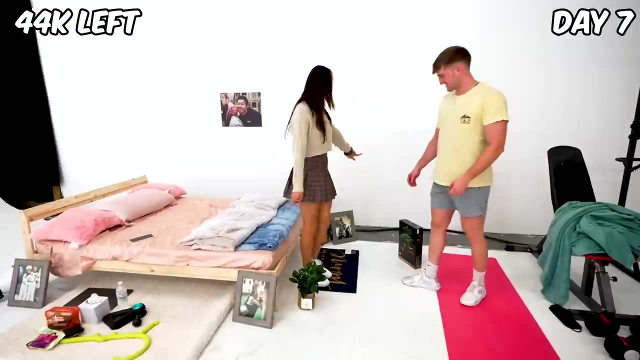 What do you think? Perfect, I don't want to do more math. no more math, no more math. I was so happy with the new decorations. of course I had to show it to my friends. It's good to be home. 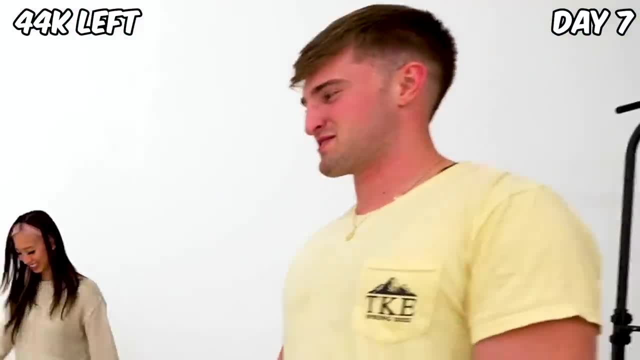 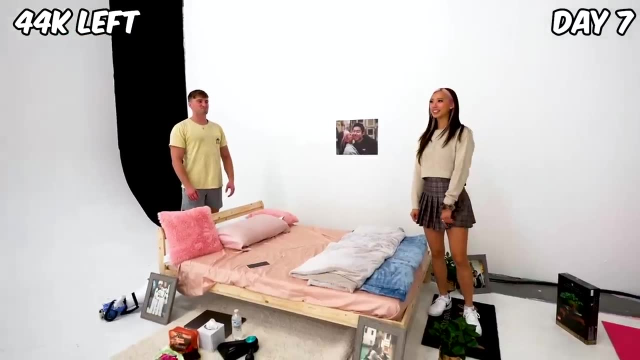 I have plants, some picture frames. Where's the pictures of me? Oh, I mean, it looks great, Doesn't it feel a little bit more cozier? Well, There's only so much I can do with math problems around me. She'll make sure you get the problem right in 10 days. 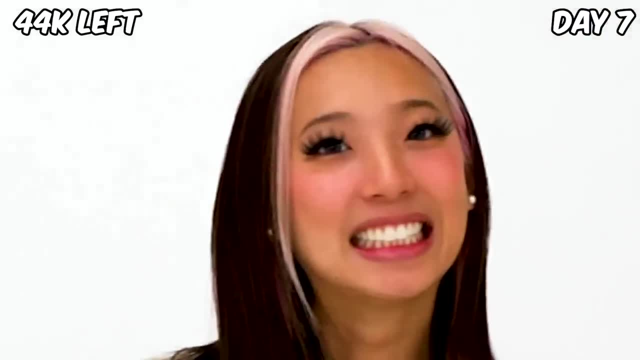 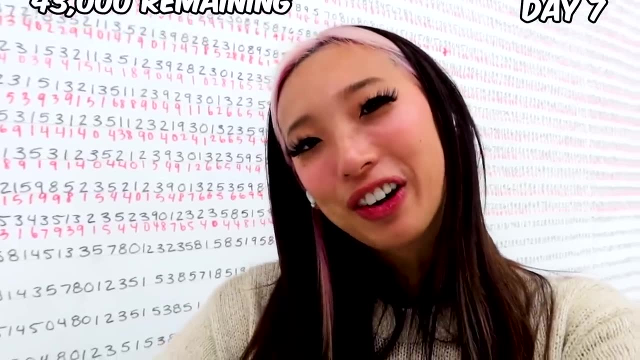 or else you're gonna get today's gonna hurt really bad. I guess this is my sign to go back to work. Woo hoo, math. This sucks. Mistake number 24.. It's supposed to be a four. I don't wanna do this anymore. 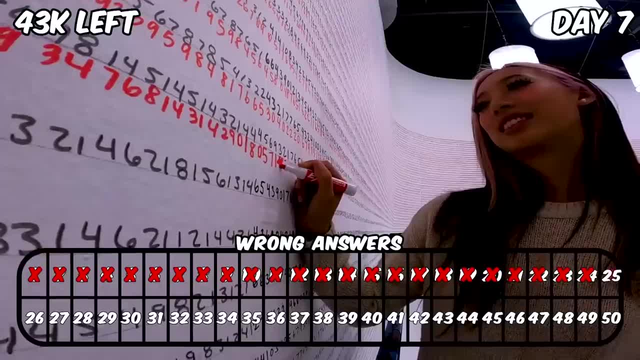 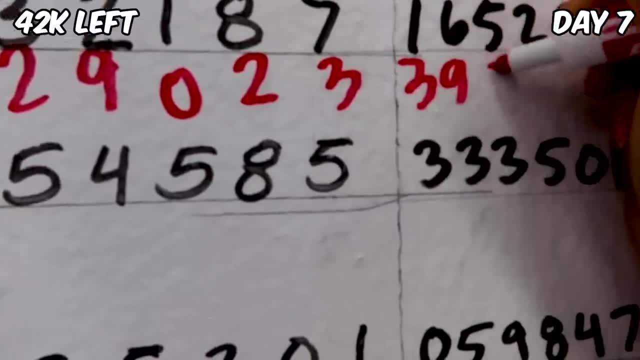 I do not think today was my day, because I just kept making mistake after mistake. Ah, no more math. I think, mentally, today is the worst day. I'm so tired I don't wanna do any math. The cool thing is though. 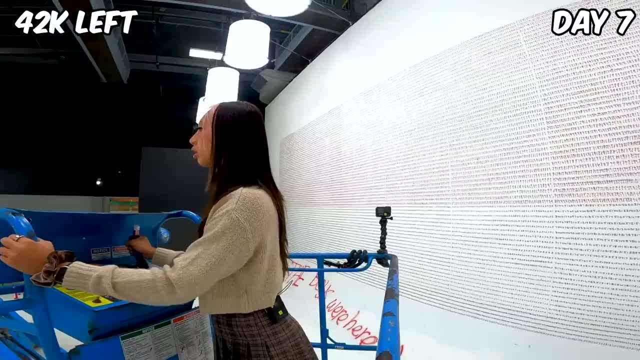 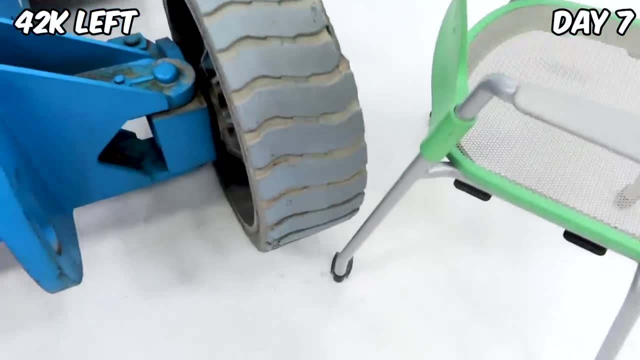 is now. I don't have to go super high up. That means I'm closer to the end. No, Oh, my god, I was so close. Look at that. I was so close. Chair, you are not supposed to be here. 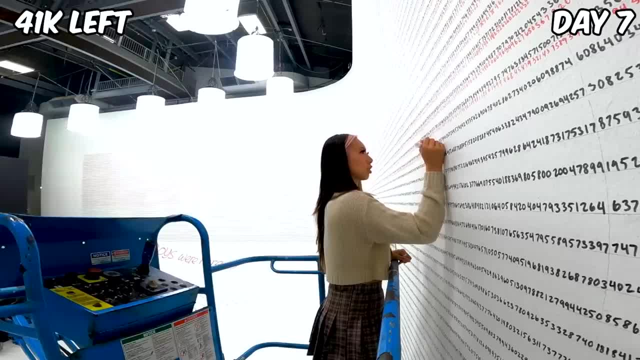 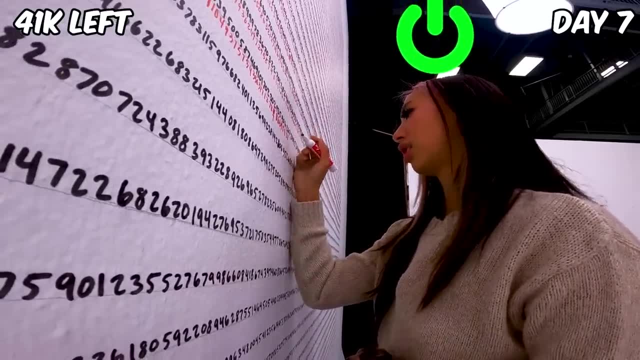 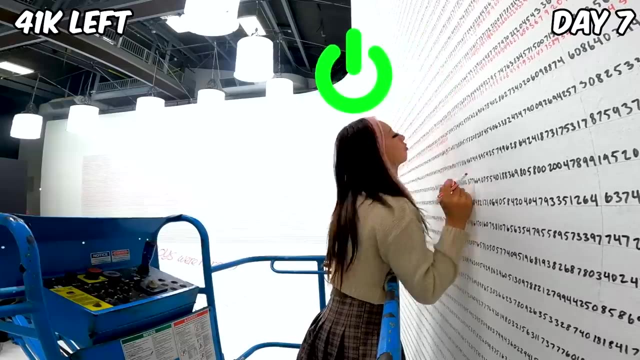 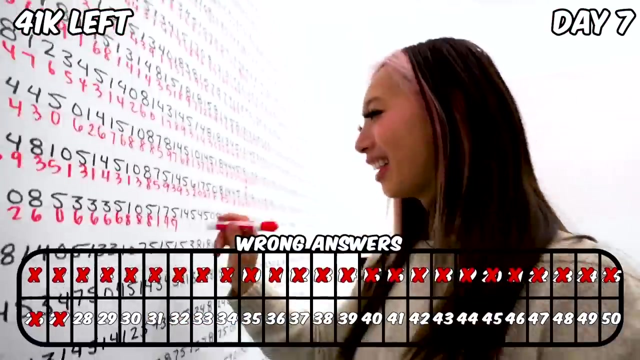 I feel like I'm going absolutely insane right now. I just made another mistake. It's supposed to be a seven. No more math. Ugh, What's going on? I made another mistake. I was gonna write an eight. 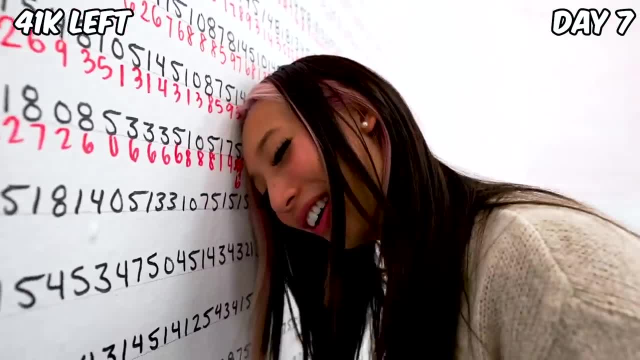 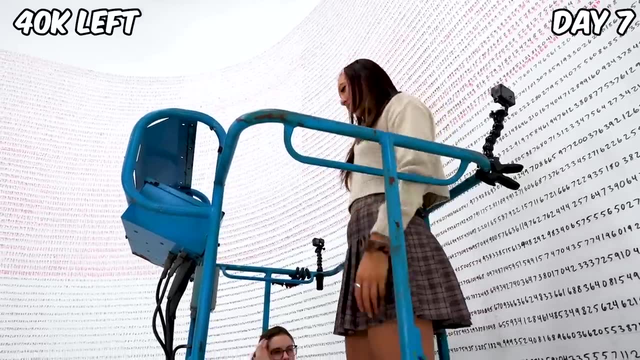 And then I changed it to a seven. it just breaks. Oh my, It's gonna be okay. When will it be over? I think I was going a little crazy earlier, So McKenzie's keeping me company, Yeah, Go machiko. 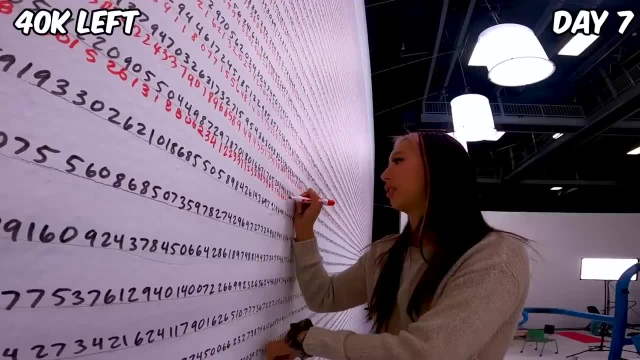 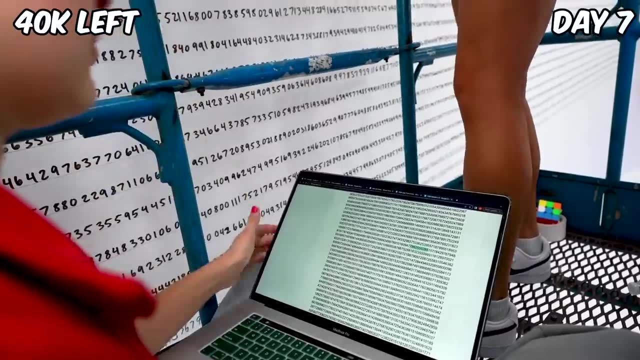 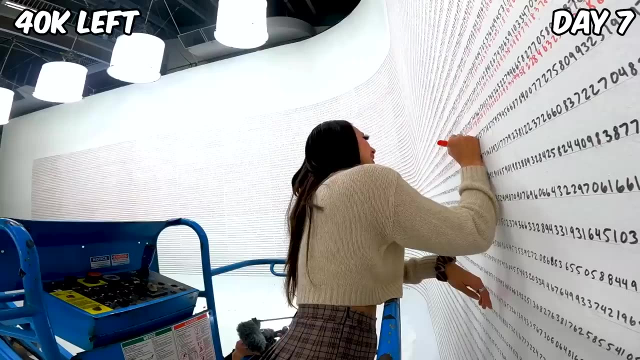 Oh no, can do it. six, two, one, two, seven, two. oh man, i wrote two, but it's supposed to be a one. you said it right, so i think between you and i that's not a mistake, thank goodness. stuff like this is why i love having mckenzie check answers for me. but good things don't always last forever. six, two, zero two. 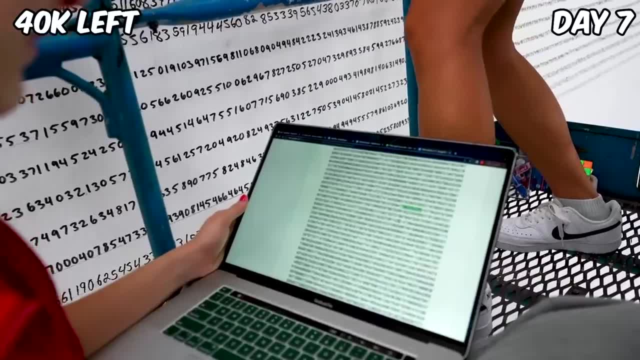 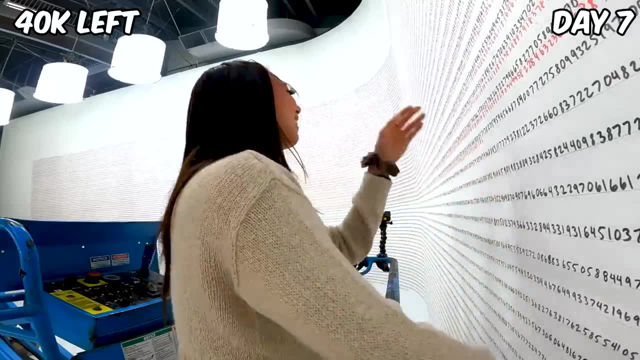 no, i got three. i wrote down three but i said two. i know, but i let you slide on the last one, so i can't let you slide on this one. i'm gonna keep going. munchie fans, don't attack me. my arms started to get pretty tired from writing all day, so i had the great idea of letting mckenzie write for me. 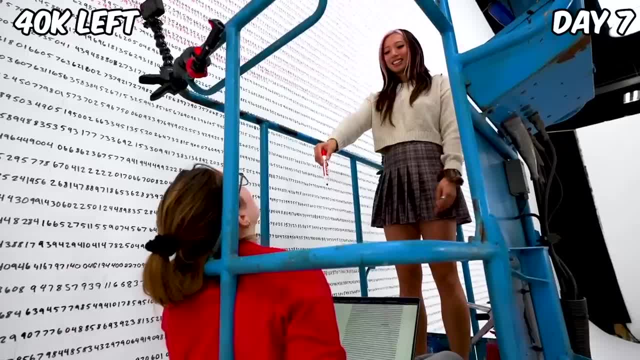 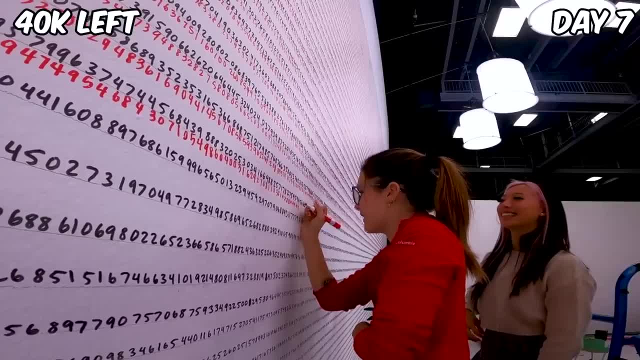 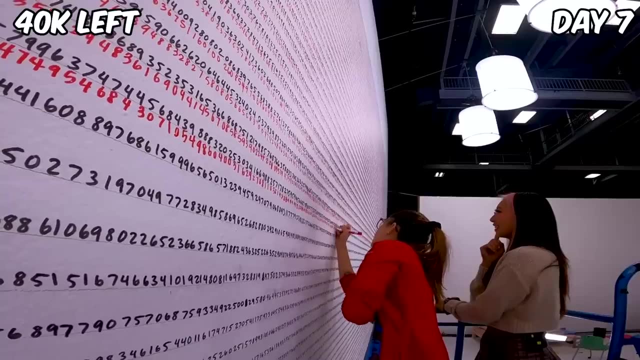 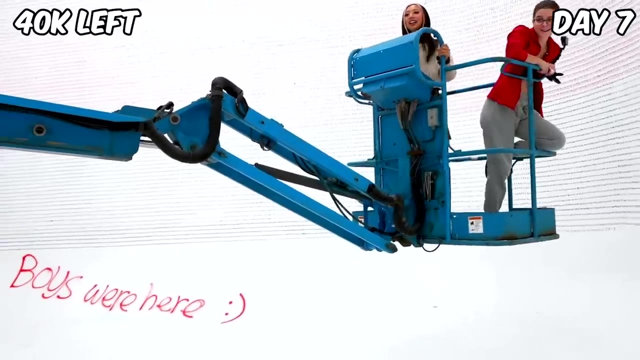 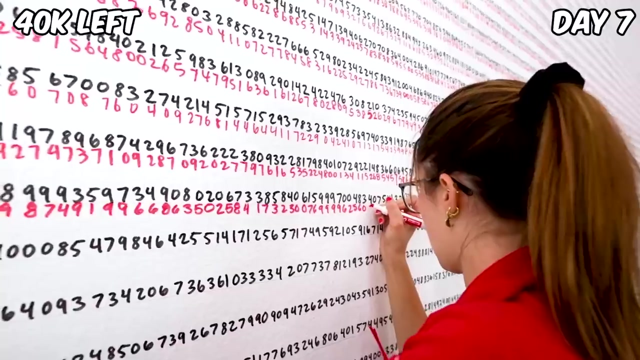 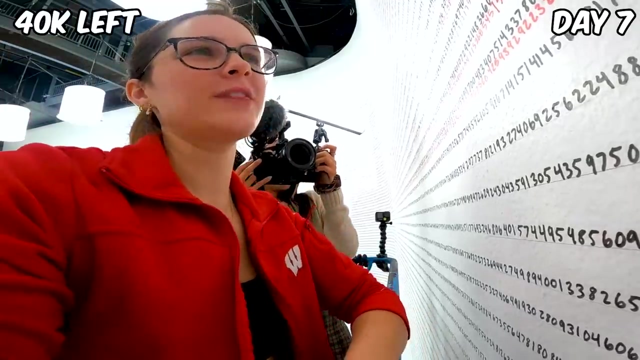 okay, mckenzie, let's switch. huh, you write, i tell you the answer: four, seven, four, nine, four, nine, nine, three, two, zero, zero, zero. another zero, four. six, zero three, one, nine. nice, you to keep going. six two zero four. that was so close to being a seven, i'm like messing up. and you're even telling me what the 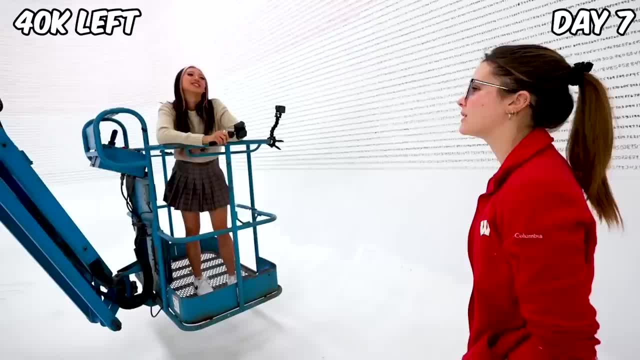 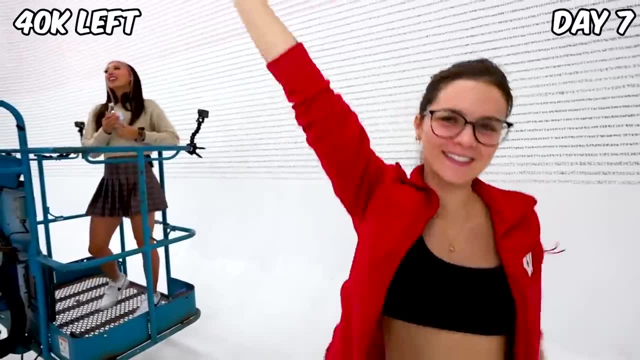 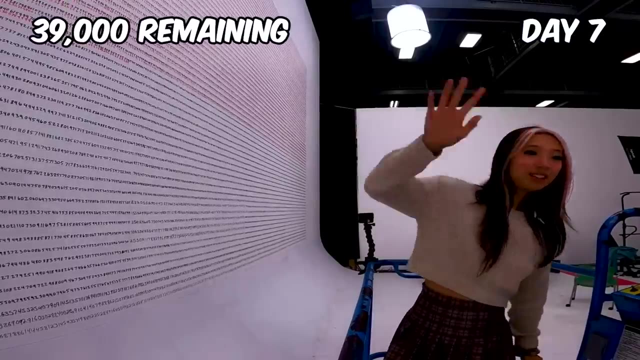 answer is: i'm really glad i am not you right now. the faster you go, the faster you're done. motivational speeches with kent. i really felt like giving up at this point, but i kept telling myself to keep going. i decided to go on, live to boost my spirit. hello day seven. let's start this thing. i finished about 60 of this. 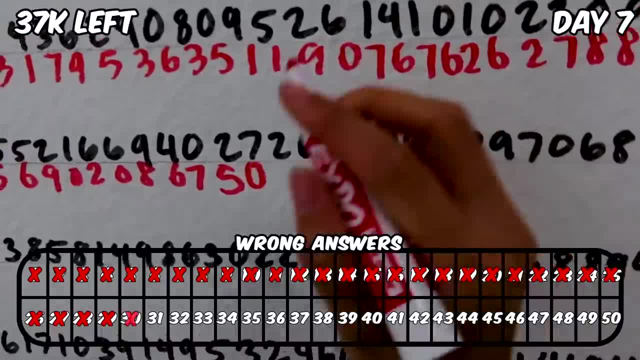 oh, i just made a mistake. mistake number 30. it's supposed to be a three. i'm slowing down a little bit. oh, this isn't supposed to be an eight, it's supposed to be a seven. i'm getting so tired. but they're so tired before even a million times. 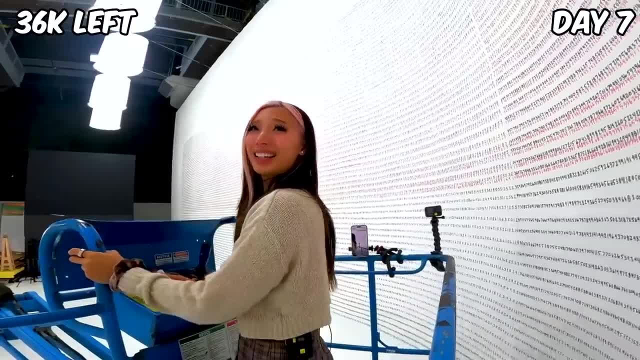 this isn't supposed to be an eight. it's supposed to be a seven. i'm getting so tired, but there's no point in damn it. i'm getting so tired, but there's no point in damn it. There's 12,000 people watching me, so I can't stop. 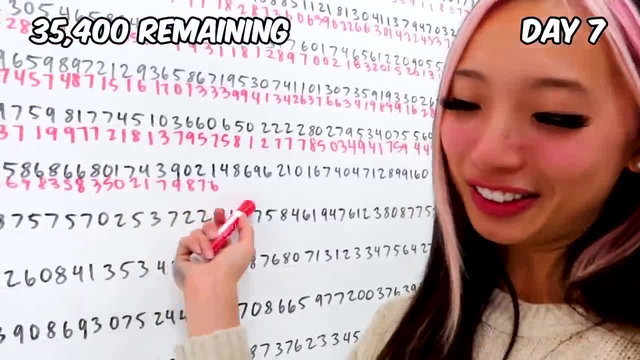 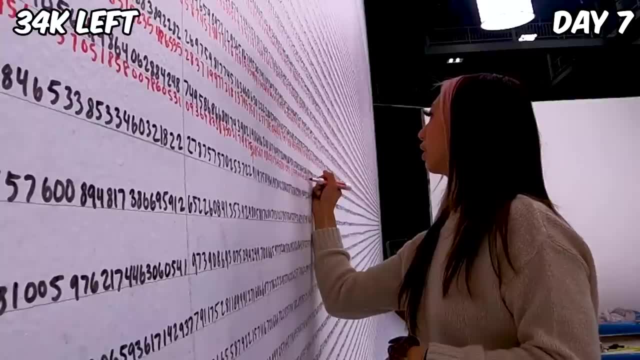 Dang it. I got a problem wrong. Mistake number 32.. Seven six eight five eight seven zero two six. I'm actually really glad I livestreamed. So many people were on and cheering me on. 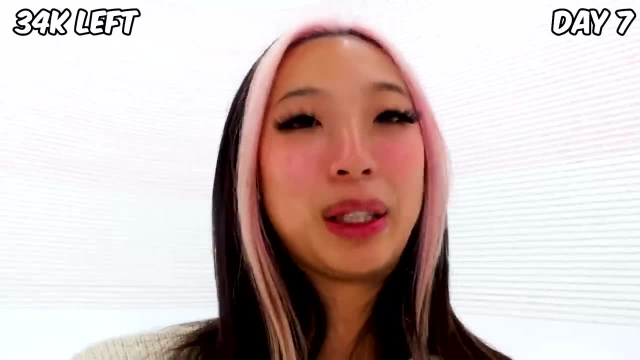 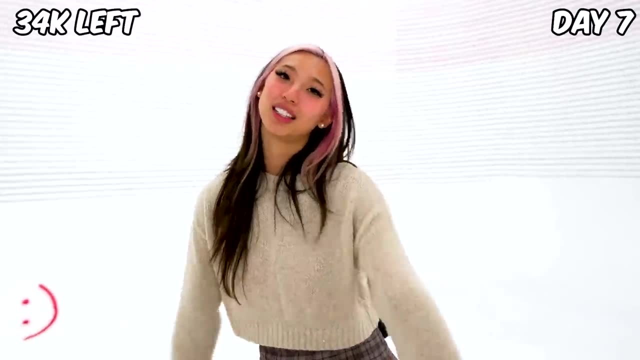 I don't think I've ever seen 13,000 people go on my live at once before. That was really motivating. I'm gonna work for another hour or two and end around 67,000 digits and then I'll be good. 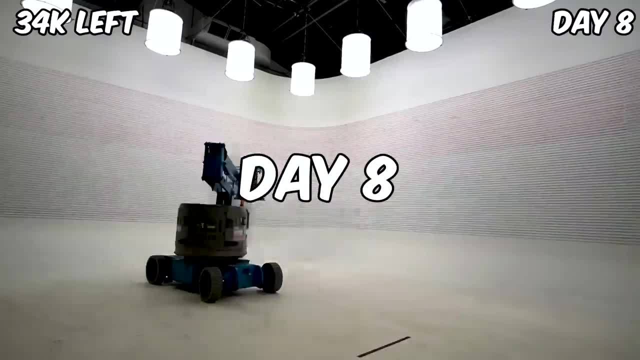 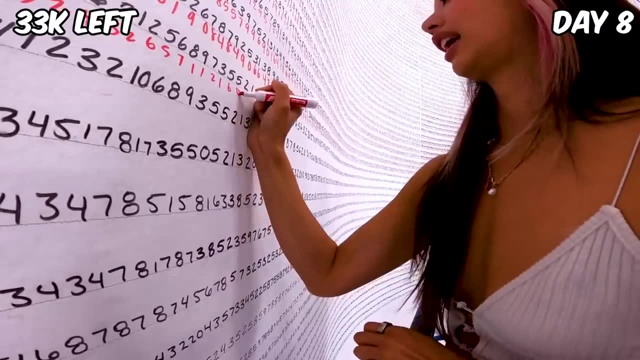 It is finally day eight. I'm pretty excited because I'm really close to the bottom. Today I need to hit at least 80,000 digits. Let's go to work. One, one, two, six, eight, No. 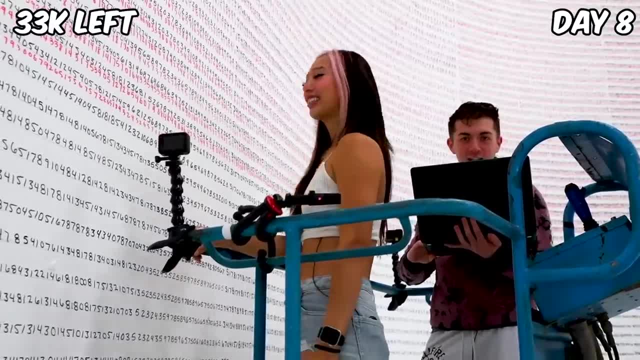 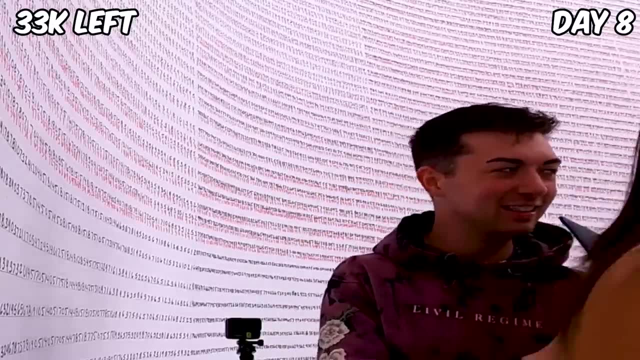 Woo, Six, nine, four, Nine four, That's number 33.. It's gonna be a little jerk. Okay, This has never happened before. We're so low now that the lift is hitting the ground. Eight zero, three, nine five. 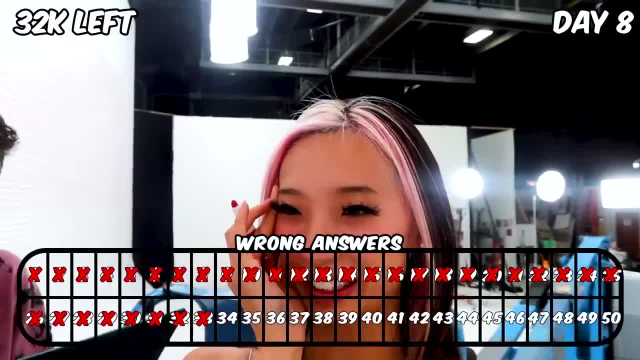 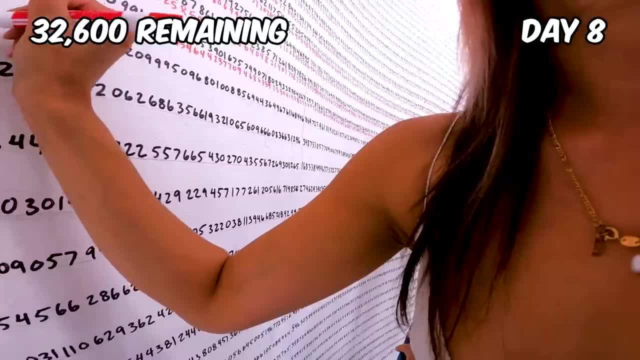 Oh mistake, Wait, actually I made a mistake. I'm not doing well this morning. Two, seven, zero, seven, Yup, Oh sad. Seven, nine, one, six, six, six, four, Oh. 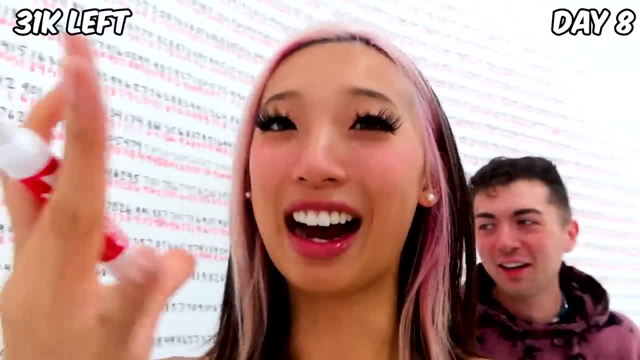 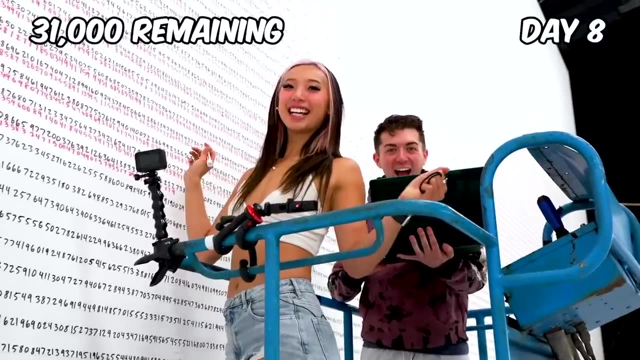 Dang it. Did I really mess up again? This is mistake number 35. We're gonna get to 40 within the hour. 68,998,, 68,999, and we just hit 69,000! Yay, Yay. 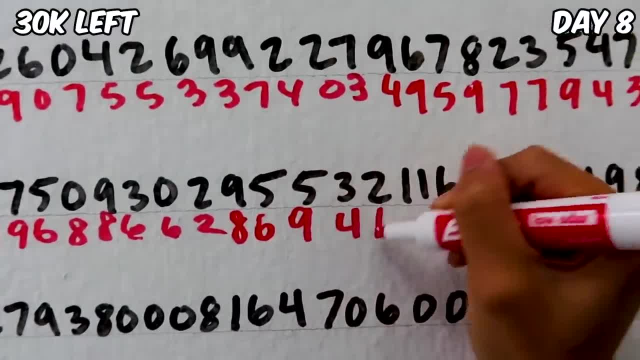 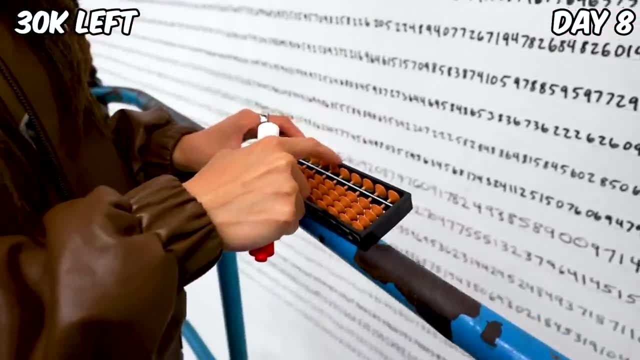 Zach's favorite number. I wanna show you how I learned to do math like this. I use an abacus. This is what I envision in my head. It's very easy to explain. This means number one On the top. it means number five, six, seven, eight, nine. 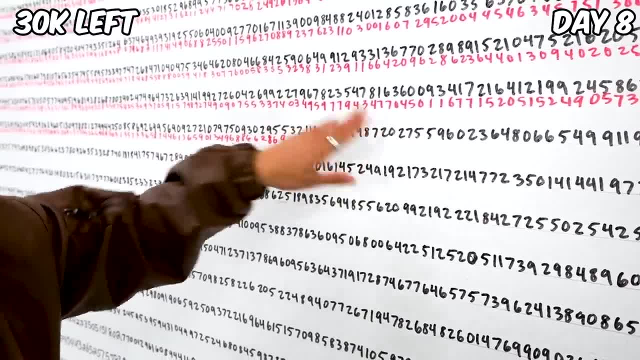 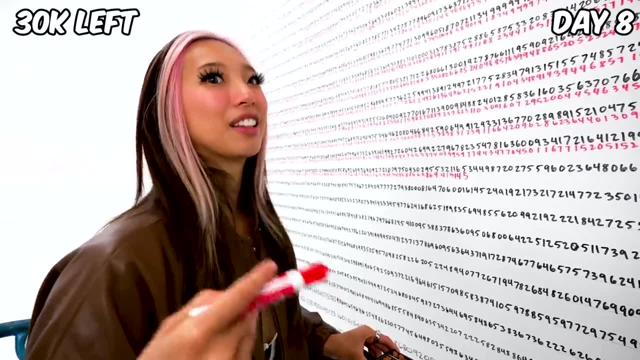 Let's say I wanna divide five, three, four, four, nine, eight, seven, two on the abacus: Five, three, four, four, nine, eight, seven, two. I have to see how many times eight goes into 53.. 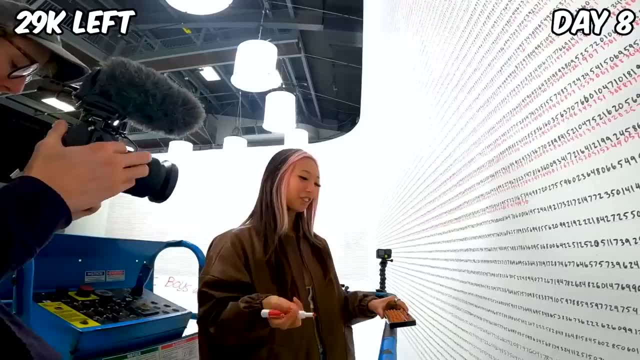 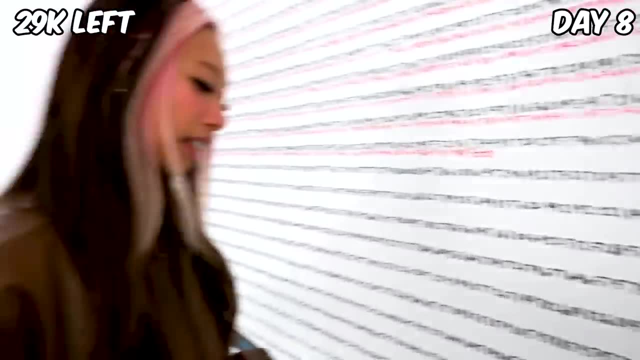 Six And then six times eight is 48, and you would subtract 48 on the abacus. The remaining numbers are five, four, four, nine, eight, seven, two, Eight goes into 54. six times again. Subtract 48 on the abacus. 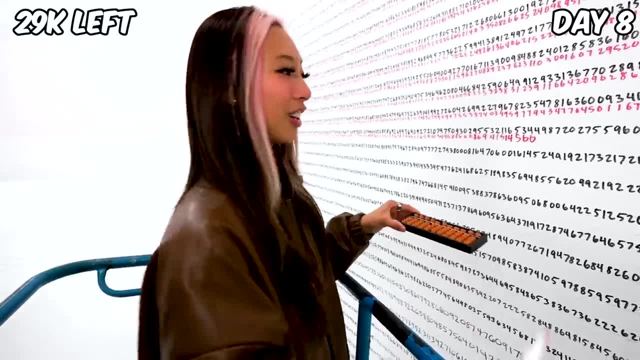 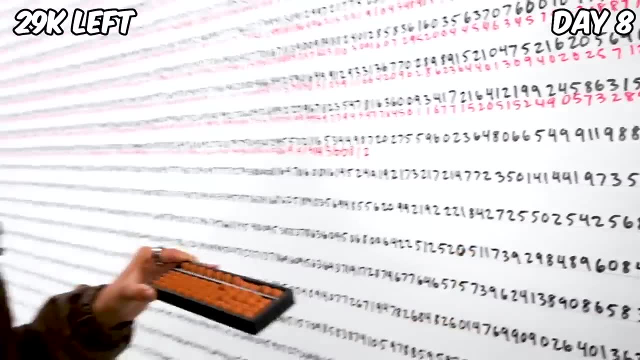 And now the remaining is six, four, nine, eight, seven, two Eight goes into 64. eight times minus 64.. Eight goes into nine. one time Nine minus eight is one. Eight goes into 18. two times Three times eight is 16.. 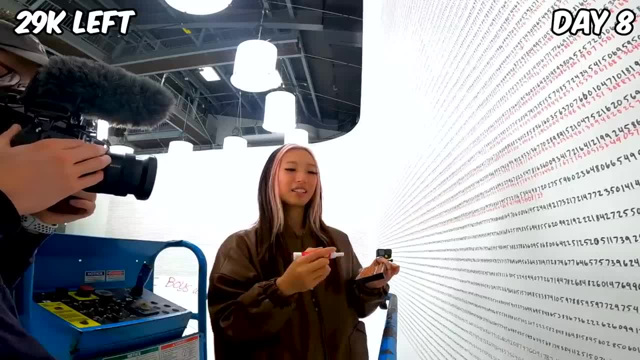 Eight goes into 27 three times. Three times eight is 24.. And then, lastly, you have 32.. Eight goes into 32 four times, And then you have the answer: Five, six, six, eight, one, two, three, four. 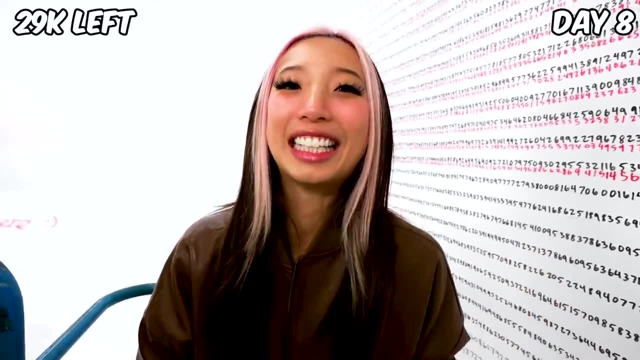 If you understood that, I'm very proud of you, And if you didn't, I'll try and explain it again some other time. I actually didn't learn this until five years of experience. Don't get discouraged. Now try dividing two seven five. 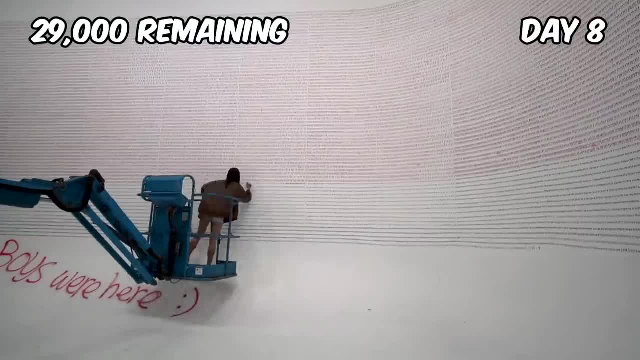 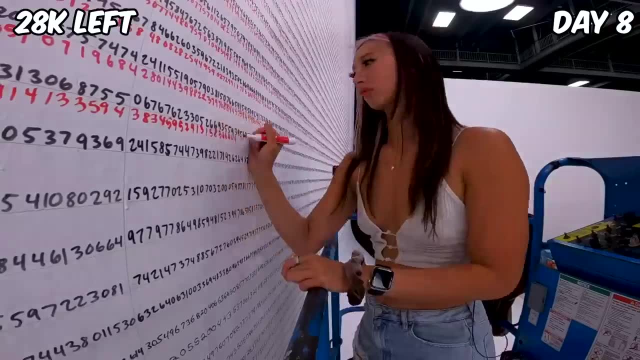 nine six by eight Comment below. if you figured it out, I never really give myself enough credit, but I'm actually really proud that I've been able to go this far into my math problem. I'm still a little bit behind, but I'm so close to finishing. 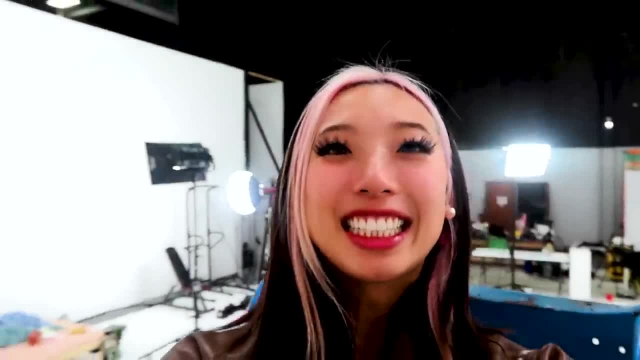 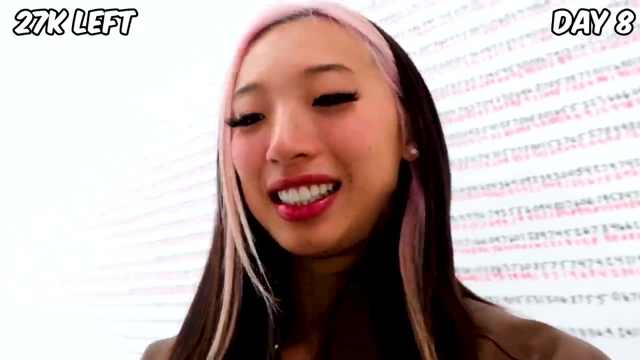 that it gives me the extra motivation to keep going. This is so crazy. Literally last week I was all the way up there And now I am so close to the end. I do see a finish line. I know I can do this. 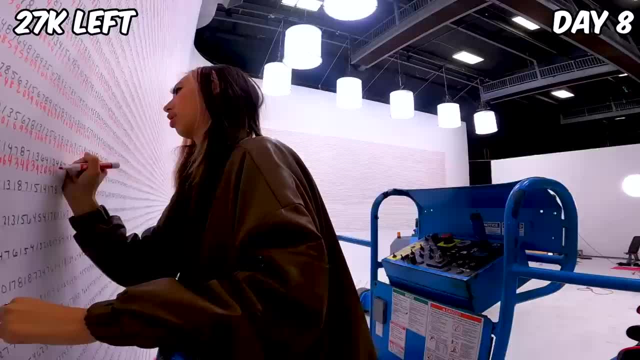 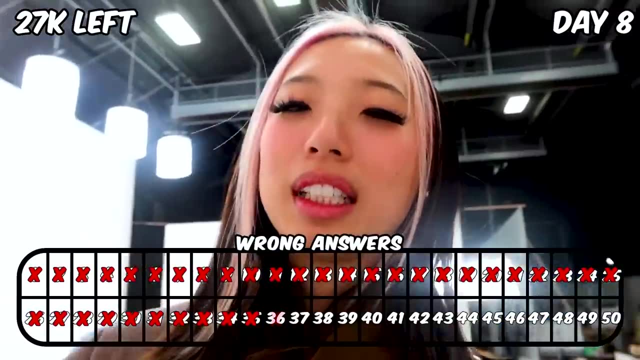 Even though I only have a couple rows left, these last few are definitely going to be the hardest to complete, just because my brain is so exhausted from all these numbers. No, All right, mistake, number 36.. It's a seven. This sucks. 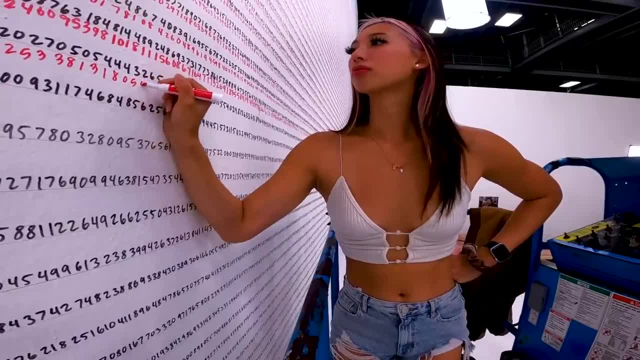 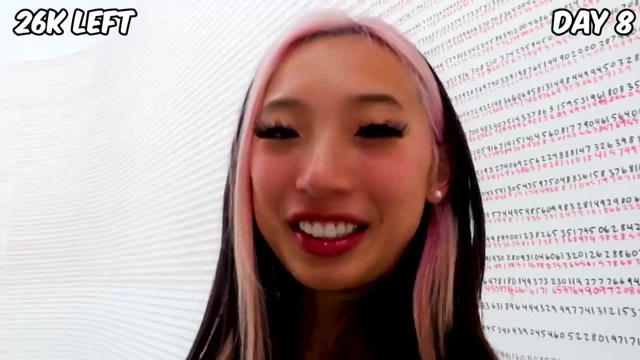 For those of you that are struggling right now in math or school in general, just know that you are not alone. I believe in you, And I hope this encourages you guys to get off your phone after this video and do something that you'll be proud of. 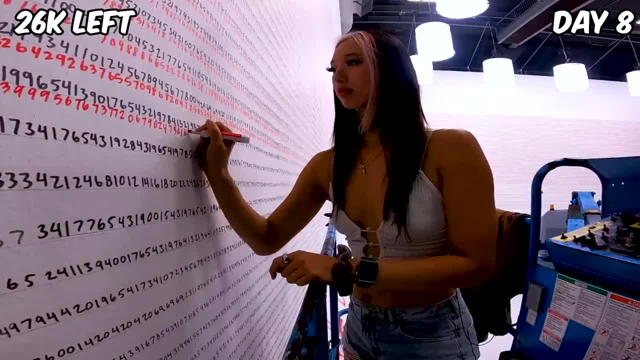 And I also want all of you to know that, as long as you put your mind to something and go after it, you can do it too. After I did the 10,000 digits in the previous video, never in a million years would I thought. 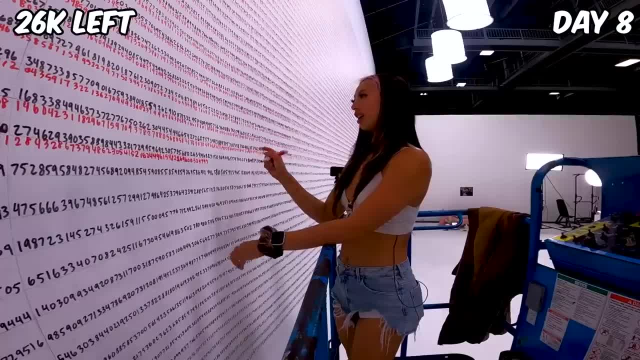 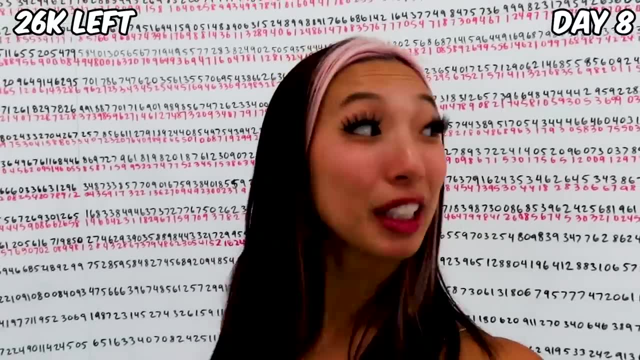 I'd be able to do something bigger than that, But here I am. Did I get this one? No Mistake, number 37, 3704.. I can only make 12 more mistakes from now on, which is really scary. 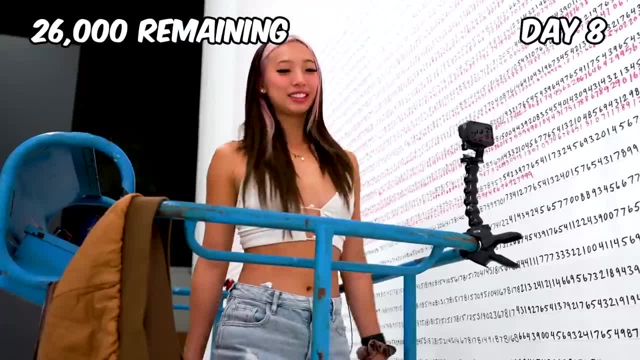 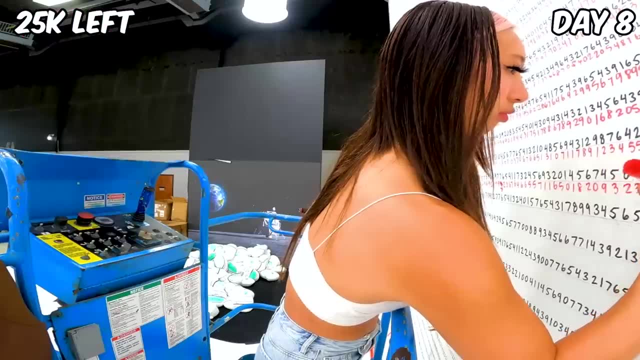 Oh, Good news: I just hit 74,000 digits. Bad news: I made another mistake. That puts me at 38 out of 50. Today's not a good day. OK guys, we need that stuff moved out of the way. 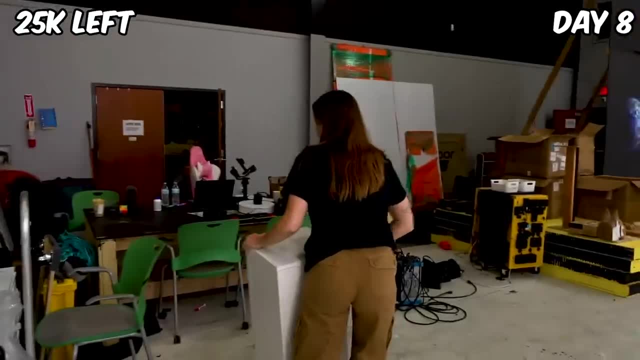 OK, Wait what? My friends saw that I wasn't having the best day, so they put together a surprise movie night for me to help take my mind off from all the math. Guys, what are you doing? Nothing, don't worry about it. 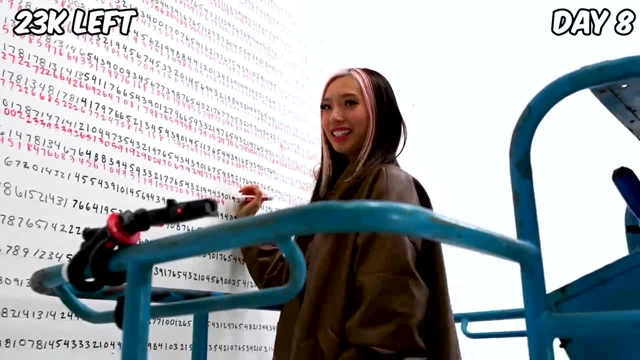 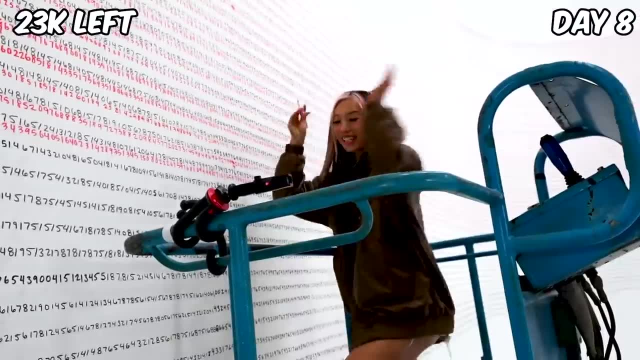 Nothing, Munchy, Nothing Estelle. That's suspicious. Just keep doing math, Keep writing down those digits, Munchy. No, just put that right there. No, because we're going to fail. Oh Damn it, I made a mistake. 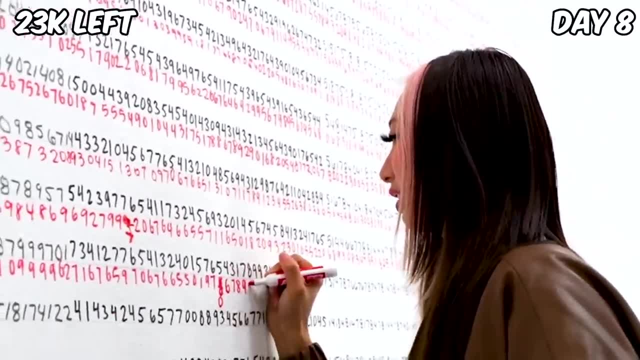 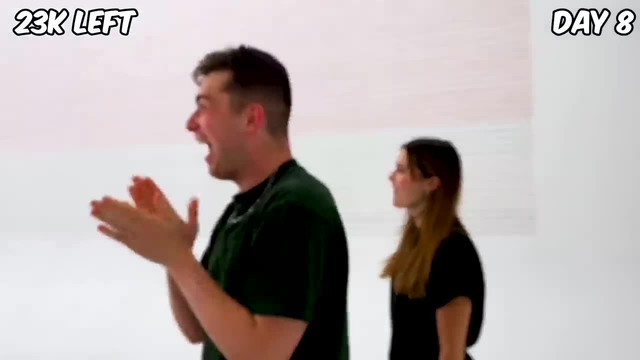 Mistake number 39, 06789.. They're very distracting. Fold the blanket, Guys. really, what are you guys doing? We're making a movie night because you've been working really hard. I like movies. I like movies. 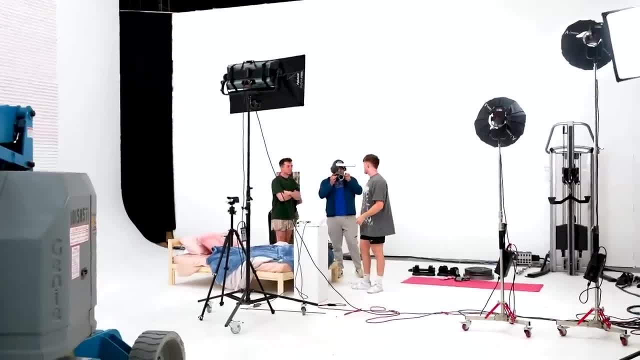 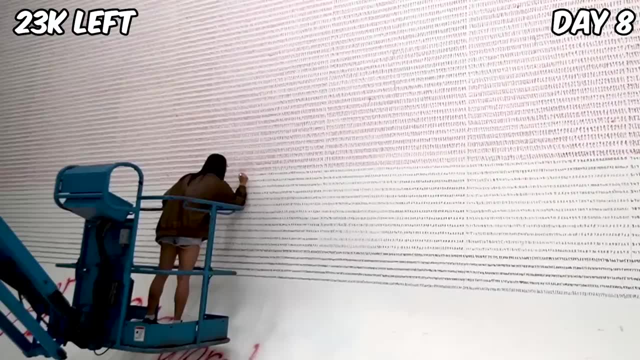 Why don't you just finish the next 500 digits and then come watch the movie with us? I mean, you still need to work. I'm going to do 500 digits so fast. I'll go get the popcorn You ready, Munchy. 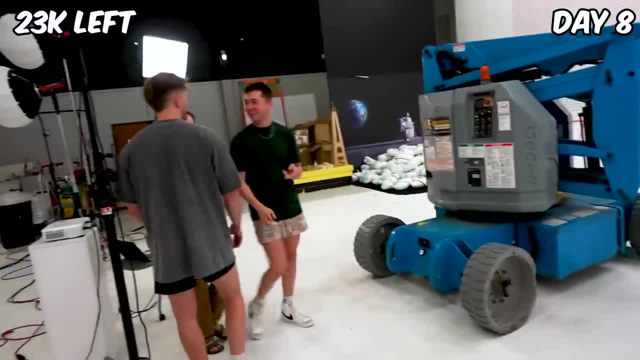 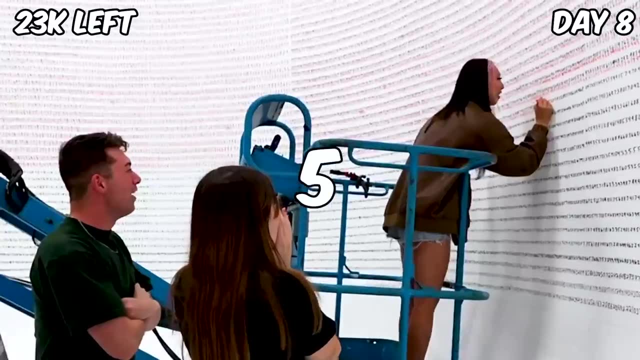 Munchy, how many do you have left? 150 left. All right, Munchy, let's go. My friends started cheering me on and when they started counting me down, I started to go so fast. Five, four, three, two, one. 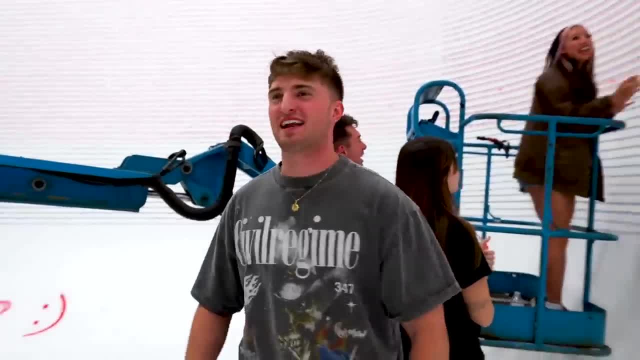 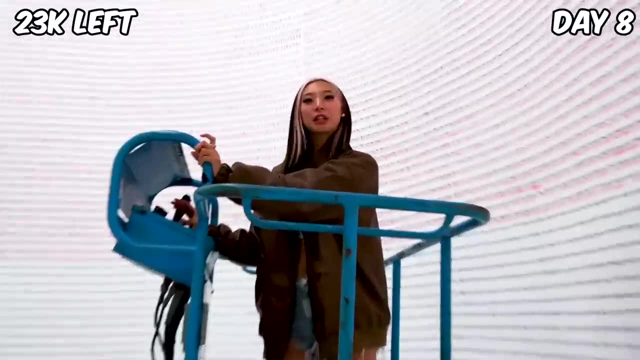 Yeah, Woo, Oh, my god, she's not allowed to watch the movie with us anymore. I'm so excited, Woo, I'm so excited, Woo, Woo, Woo. We're watching Shrek. Oh, I thought I'd never watched Shrek before. 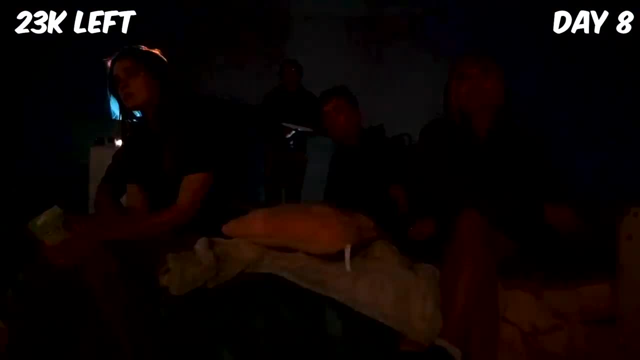 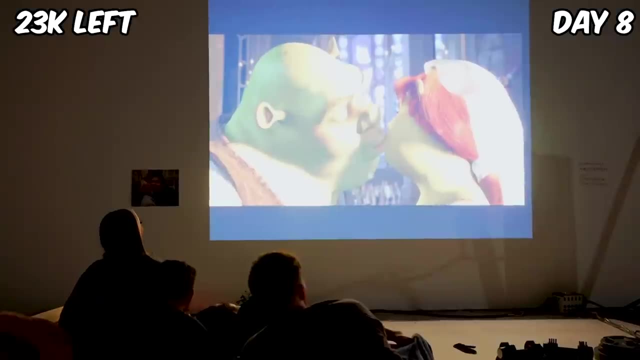 My friends are so kind and amazing for doing this for me. This moment right here is definitely what I needed, and I'm so grateful for them. Today I started off pretty bad. I was really tired, But today I ended on a really really good note. 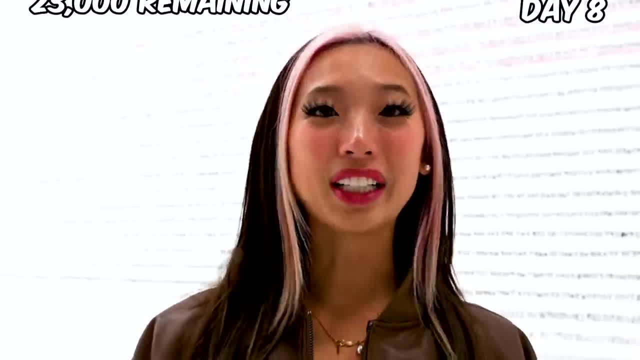 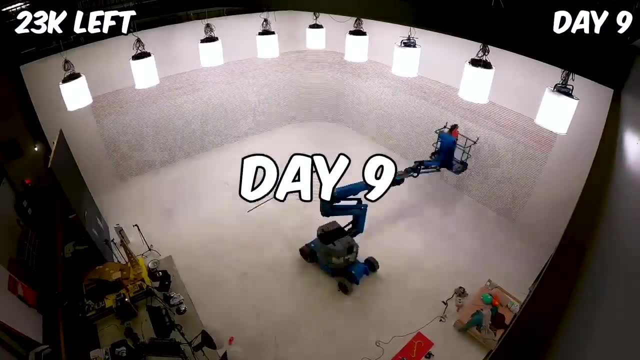 And I completed 77,000 digits. Two more days. 20,000.. 23,000 more digits. I'm so excited for the last few days And it's day nine. I only have two more days left. I'm really excited because I'm almost finished. 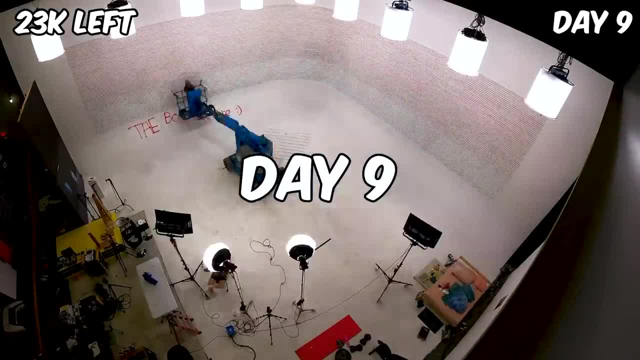 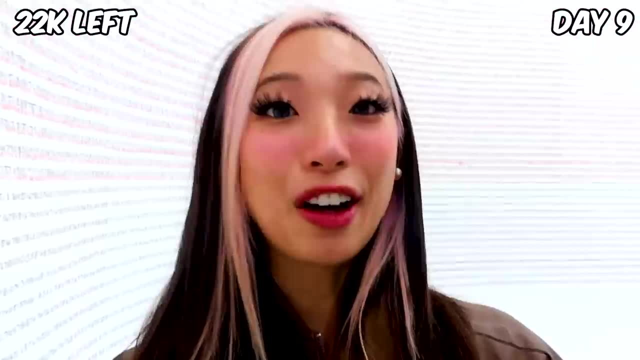 But I'm also really nervous because I still have 23,000 more digits to go. All right, I made mistake number 40.. Not off to a good start on day. nine, Six, eight. I only have nine more mistakes left. 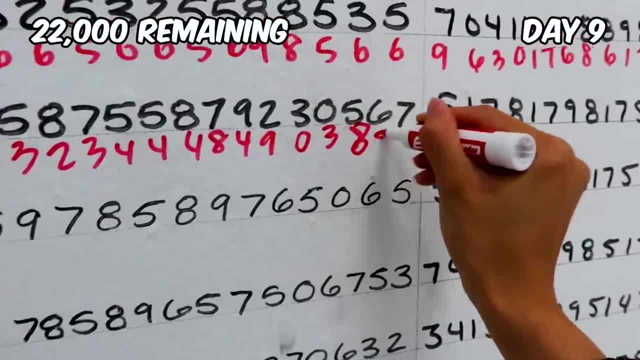 I have to be very, very careful from now on. I realized that after writing for nine whole days, my hands started to hurt a little bit. It's actually not that bad, It's actually starting to hurt a lot. So I'm going to look around to see if I can find anything. 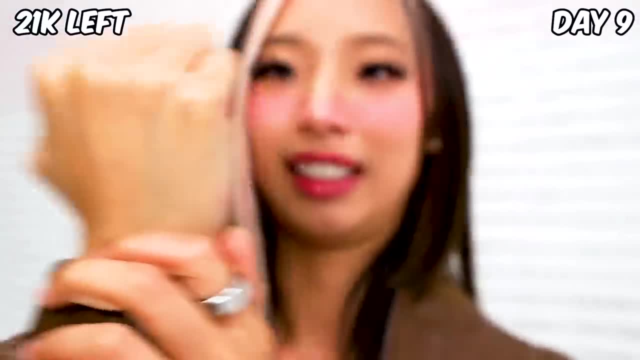 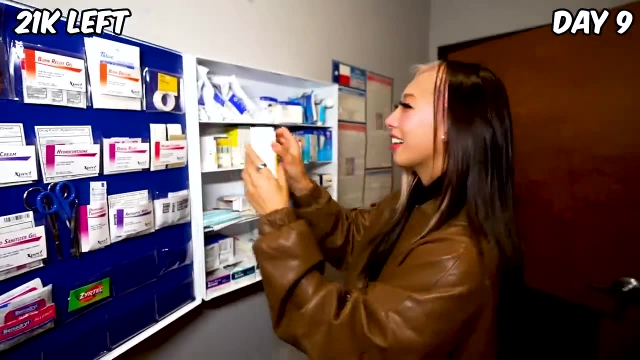 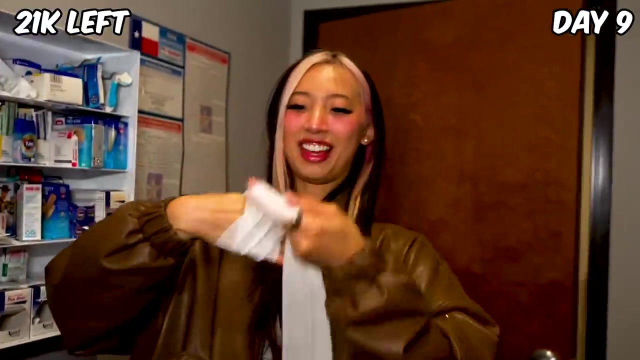 to wrap my hand with. It's so red. Can you see it? Did you get a boo-boo? Oh my god, I need to find something. Don't mind me. Oh, This might be it, Jake. Oh, perfect. 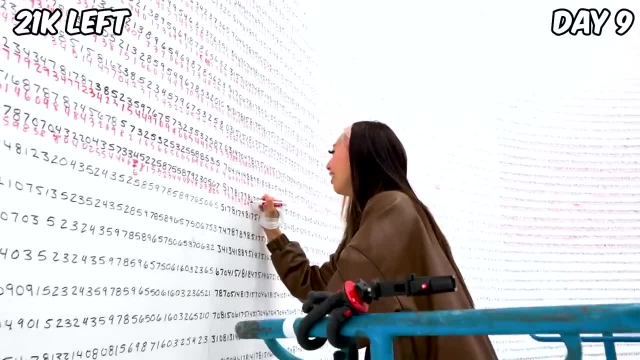 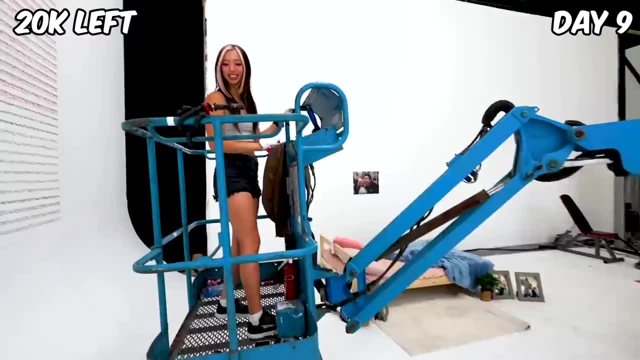 It's like a nice little cushion. Let's see if it works. It works perfectly. This is so exciting. I think I can finally work on the girls. I'm so close to the ground. I'm so close to the end. Let's get down. 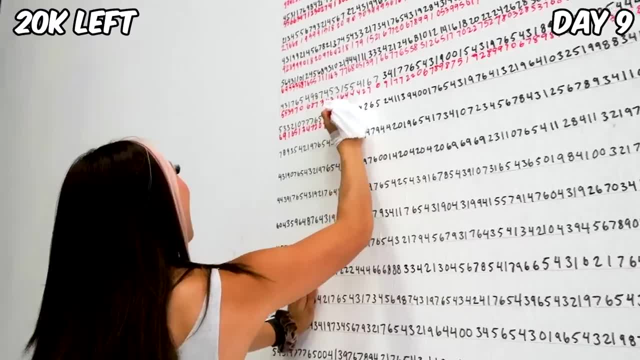 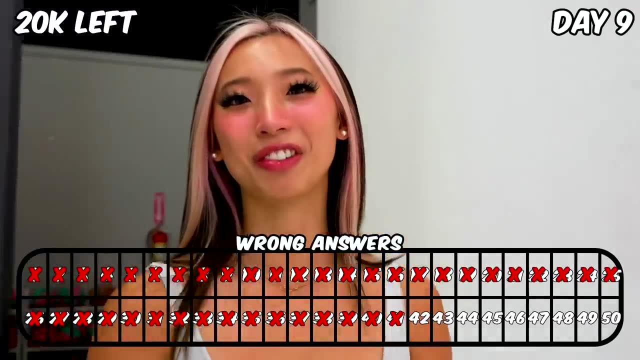 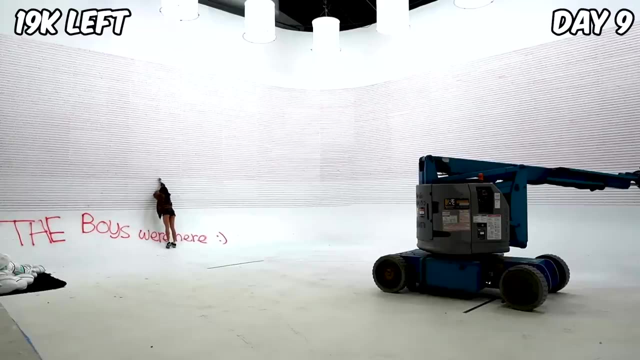 I can finally work faster. I don't have to use the lift anymore. Yay, Oh, uh-oh, I made a mistake. Mistake number 41.. Maybe working faster isn't a good thing. There you go. I thought working on the floor would be so much easier. 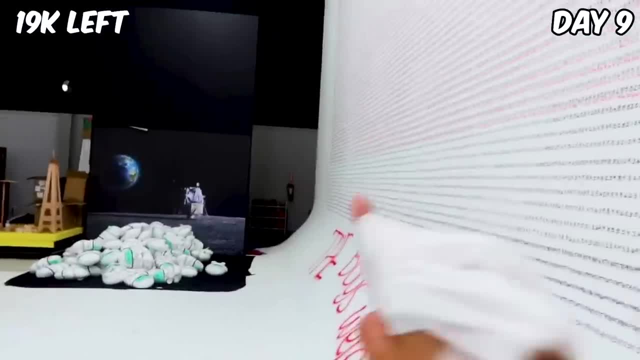 But actually working on the floor is so much harder. You can kind of see over there that it curves a little bit, So it makes it really hard for me to step on the floor. I think I'm going to get back on the lift. 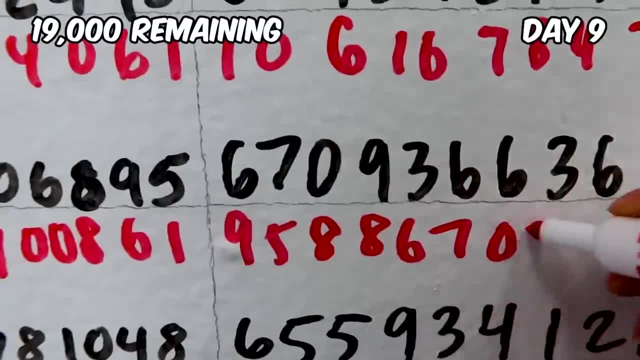 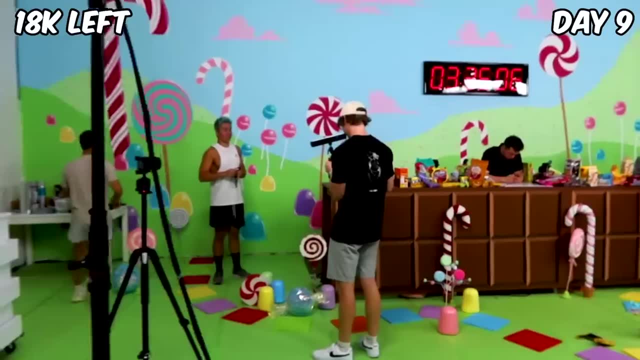 I've missed you. The next set: my friends are working on a craft video. I'm kind of getting FOMO. All right, Jake, Get over here, Wait, but that's not possible. Judy, Judy, Judy, This looks so much fun. 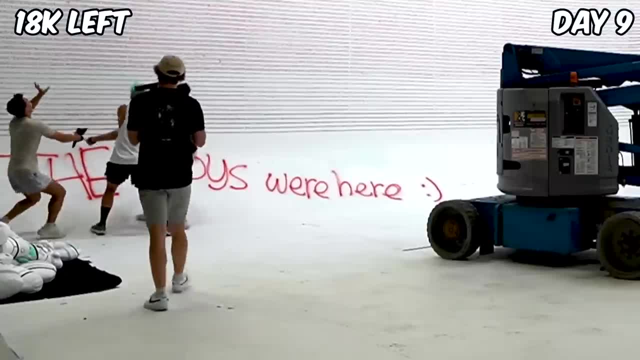 We are having a lot of fun. Dad, get in the car. Get in the car Before we can get back to work. they have to put on the dino costume. Oh, While they make candy art, I'm going to do more math. 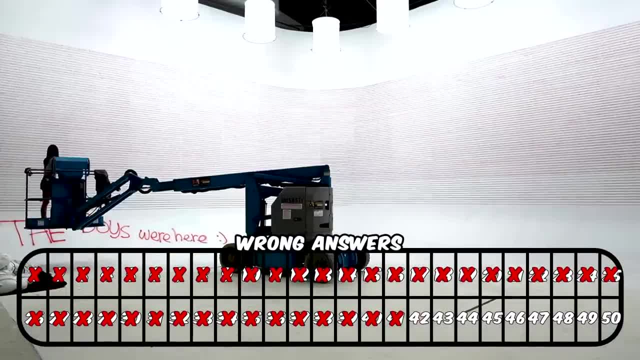 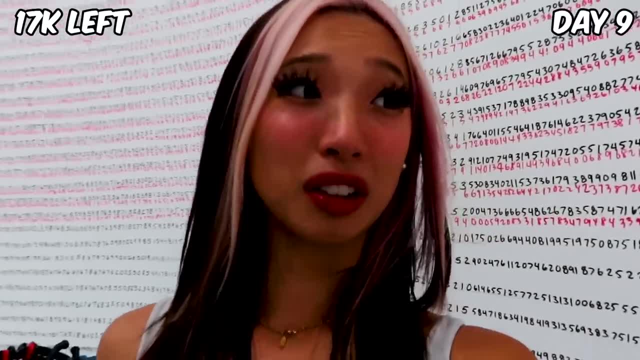 Say it. Mistake number 42.. I accidentally wrote a six instead of a seven. Go, Michelle. 13 more rows. I can only get seven wrong. That means I can have one mistake for every two rows, which is not a lot. 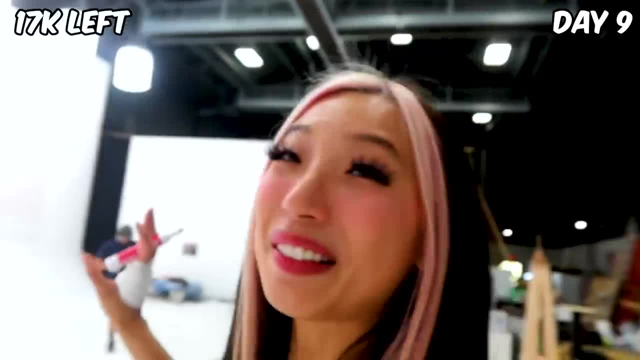 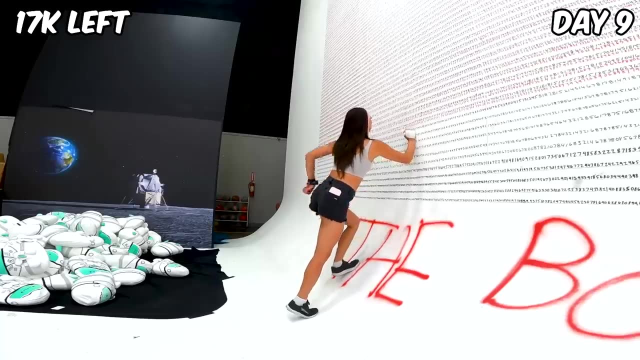 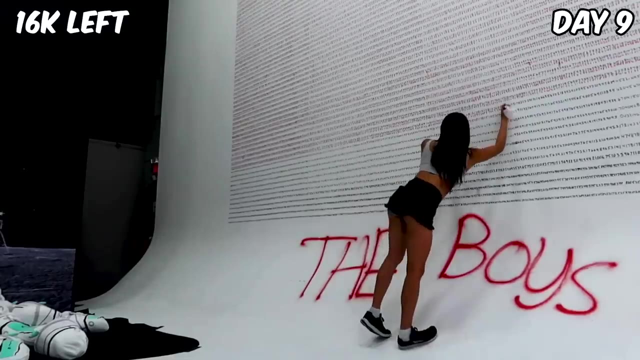 Finally reached the point where it's comfortable to work on the ground And I'm going so fast now. If I finish this, I'd be so proud of myself. Power stance. The last few days have been really really rough mentally, But at this point it's more of a physical challenge. 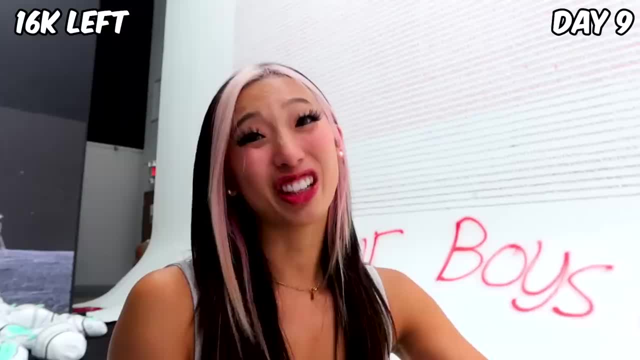 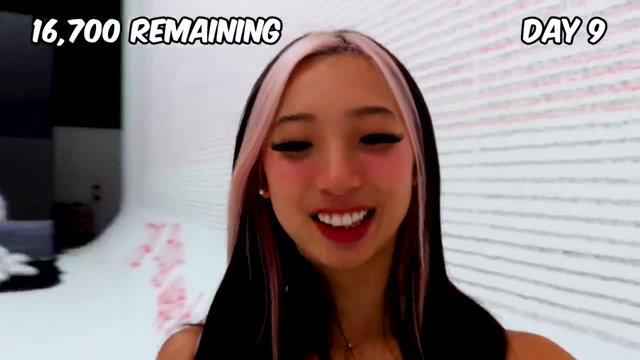 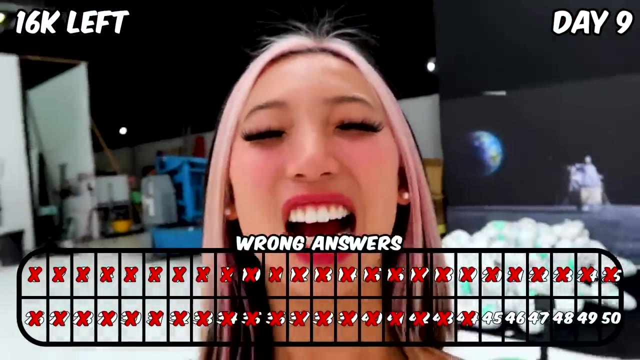 It's more of a mental challenge than a mental challenge. My legs hurt, My feet hurt, My hand hurts. This is definitely not what I was expecting. All right, Mistake number 43.. It has to be a one. Mistake number 44.. 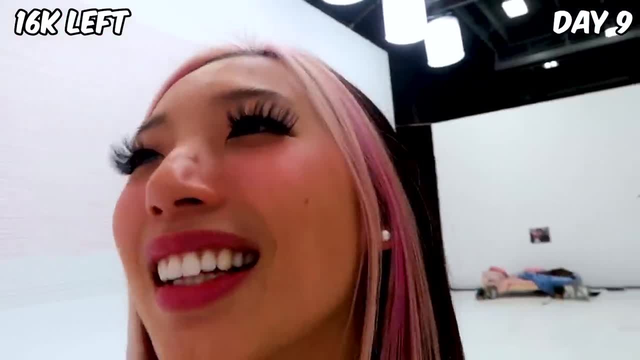 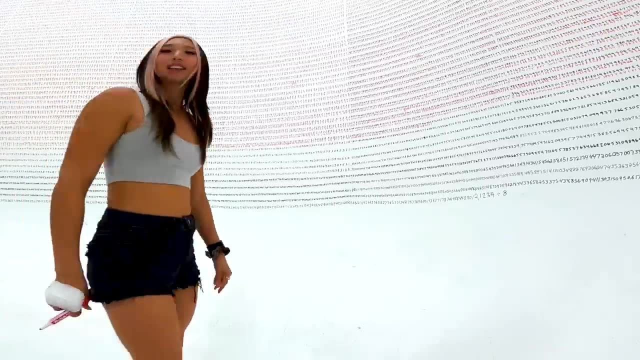 It's actually a three. I don't want to do this anymore. I'm so close to the end, though. No more math, I'm alive. Everyone say hi, Let's do some math. Doing these slides are so fun, And you guys really gave me good company. 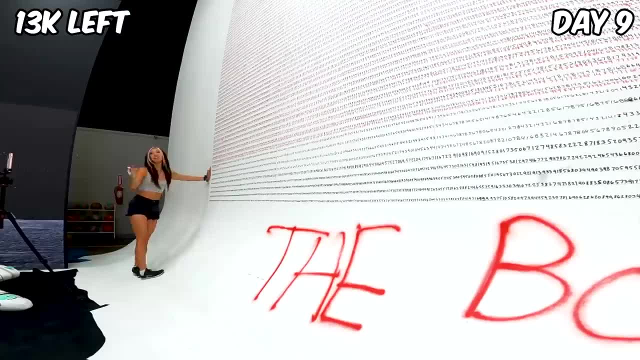 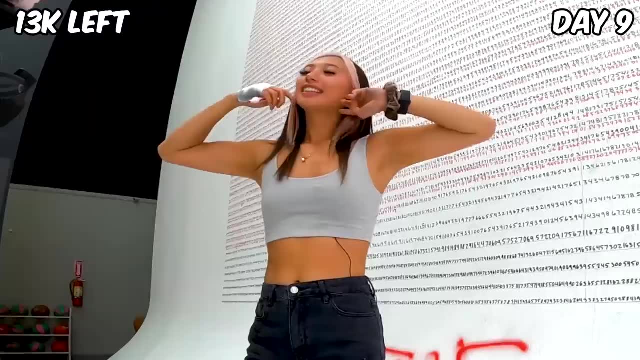 I hope you guys were entertained with these as well, And thank you to those who joined. Oh man, I made a mistake. Mistake number 45. It is supposed to be a nine- Those of you that are watching. thank you so much. 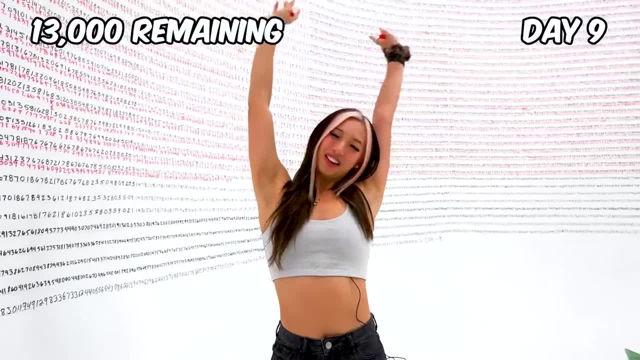 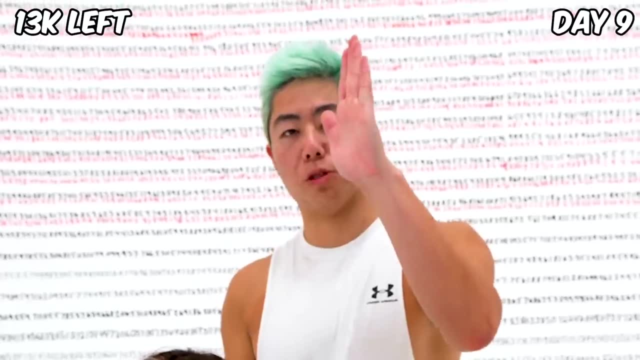 I love you. I am at 87,000 digits. My arm is getting so, so sore. Zach, you want to give me a massage. Massaging Michelle's neck is very interesting. Most people's are like this. Michelle's is like that. 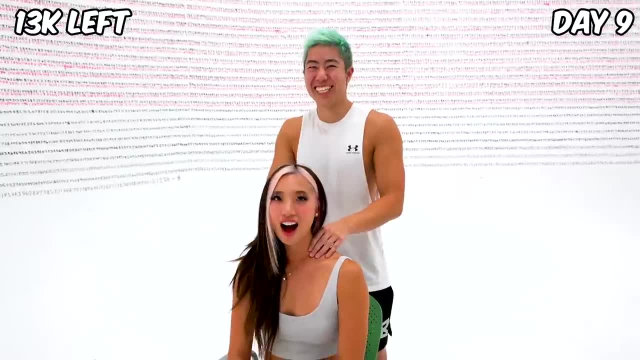 Are you calling me a hunchback? No, I'm calling you a hunch neck. I kind of see what you're talking about. I do not have a hunch neck. See, Michelle has a hunch. Oh my god. 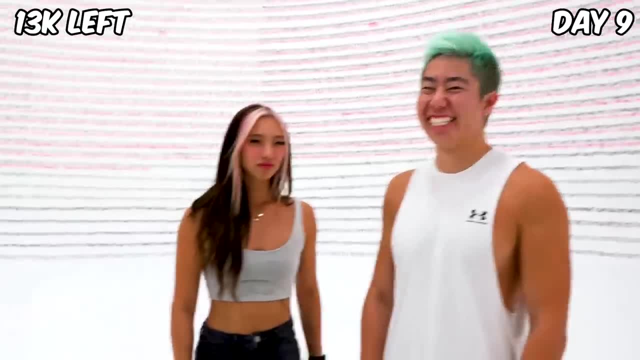 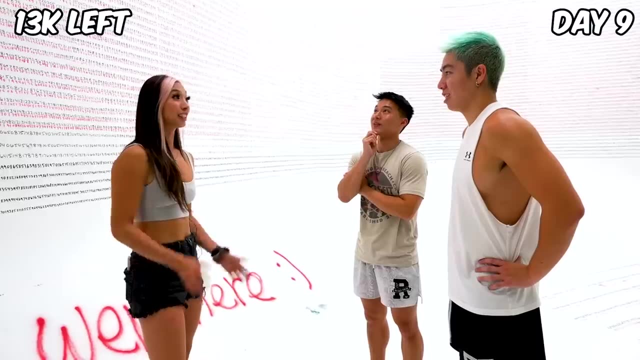 Okay, that's enough. Your posture is like this: Wait, she's doing it right now. Zachary, Look at how much I've done so far. Holy cow, That is ridiculous. Do you guys want to guess how much I've done so far? 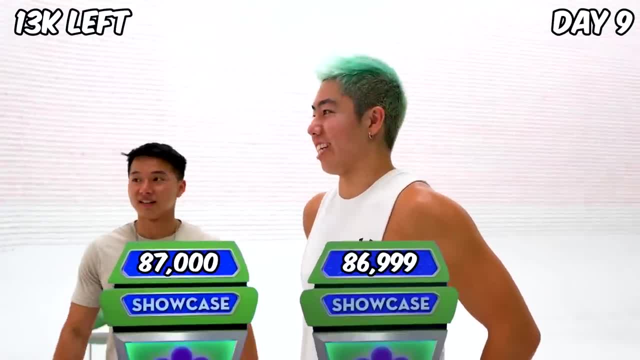 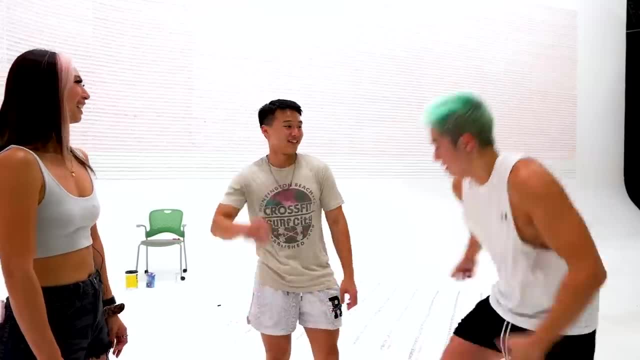 87,000.. That seems too high- 86,999.. I hit 87,000.. Really Why? Yes, You're telling me, Ben got it exactly and I was off by one digit. Yeah, I hate you, Ben. 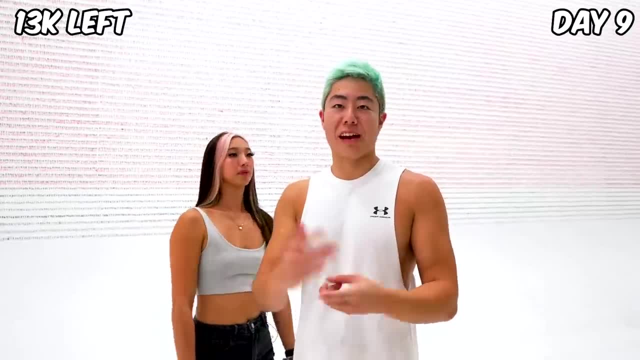 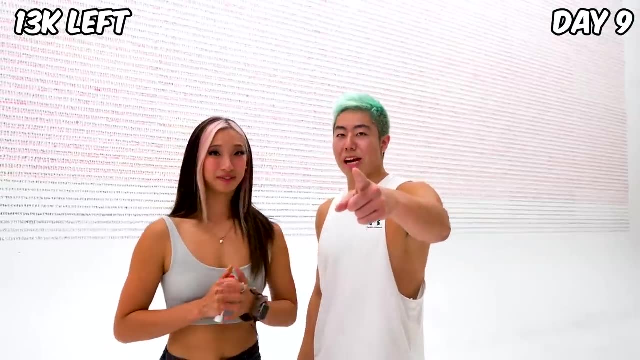 Okay, I love you. I've been doing YouTube a while. I do some crazy challenges. I've seen MrBeast do crazy challenges. I don't think I've ever seen anything this mentally taxing in my life. You guys in the comments right now call Michelle a strong woman. 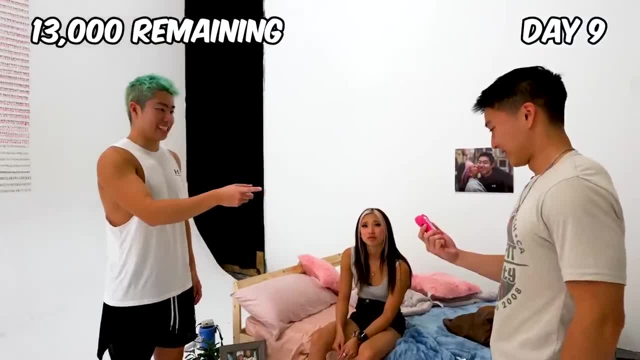 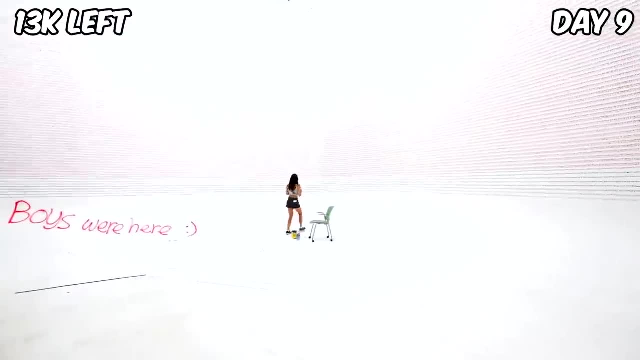 It's pretty impressive. I'm honestly very proud of Michelle. Don't forget, if you don't finish in 10 days, Oh my gosh, okay, I'm going to say that again. I love that. Call Michelle faster, faster. 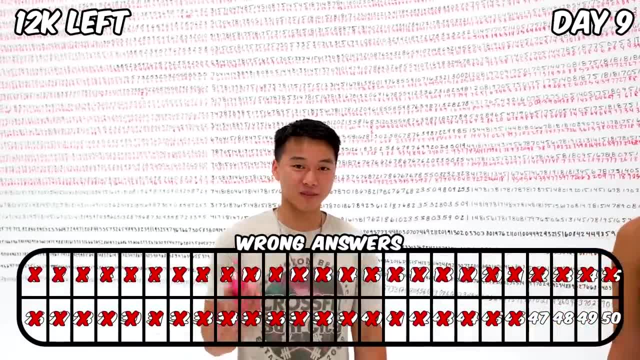 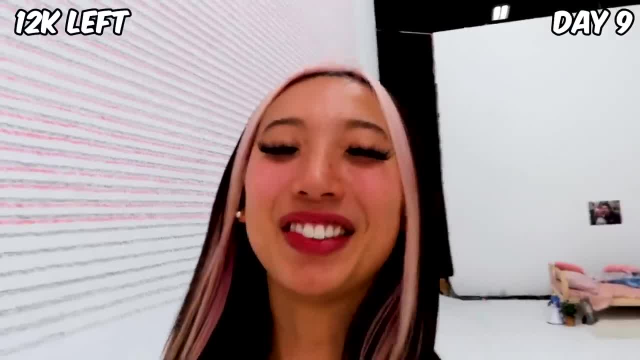 Bad. You made me make a mistake. I kind of feel bad, But then also I'm the gambitager. I just made a giant mistake. The correct answer is 7.. Mistake number 47.. This is not looking good. 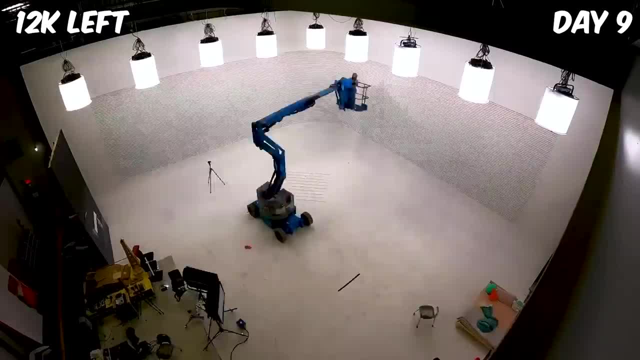 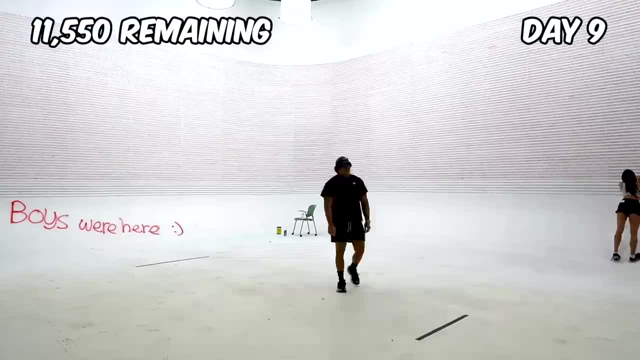 I'm only a couple mistakes away from having to restart the entire problem And, to make it worse, there's only one day left, So there's not enough time for me to finish if I have to restart, Alright, I think I'm going to finish the route and then end it today. 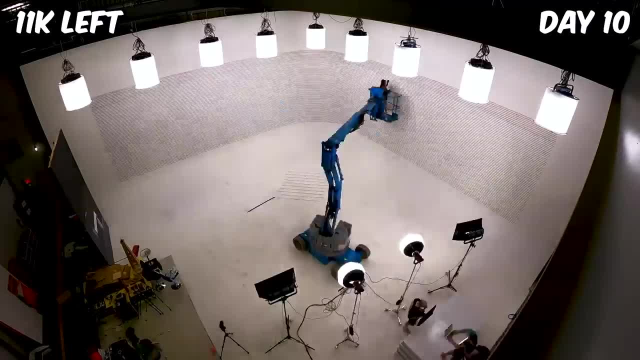 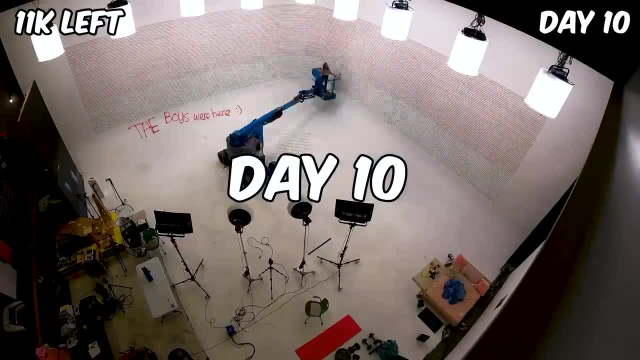 11,000 more digits for tomorrow. Yay, It's day 10 and I'm so tired. Everything hurts, but I'm so excited. It's the last day. This has been the longest 10 days of my life. I have 11,000 digits left. 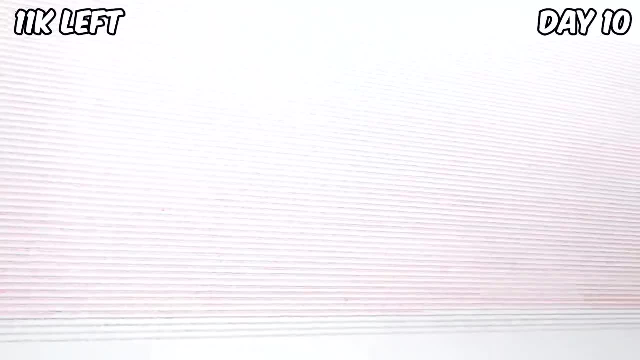 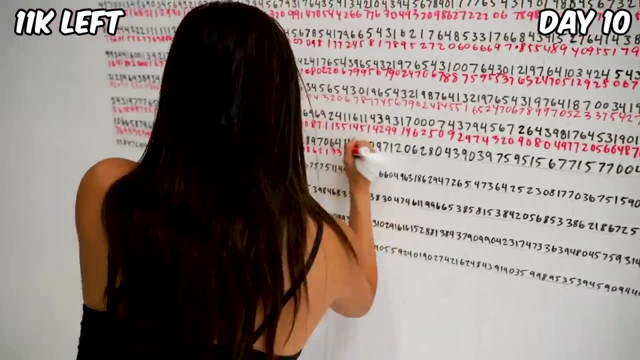 I'm at 47 mistakes. I'm worried, but also really excited. I'm so proud of what I've done so far. I'm finally so close to the end. I still have 11,000 digits left, but I'm only allowed to make three more mistakes. 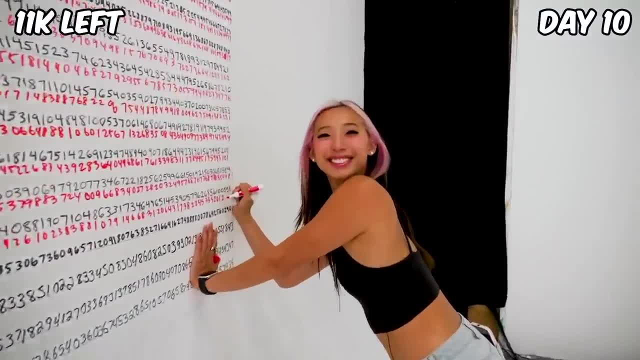 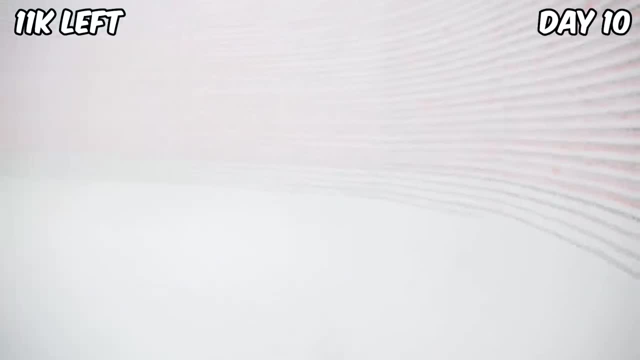 If I get to 50 mistakes and have to restart, all my hard work would have been for nothing. But this nervous energy is making me more determined to finish strong. All the encouragement from my friends is making me feel better. All the encouragement from my friends has given me unlimited motivation and their unwavering 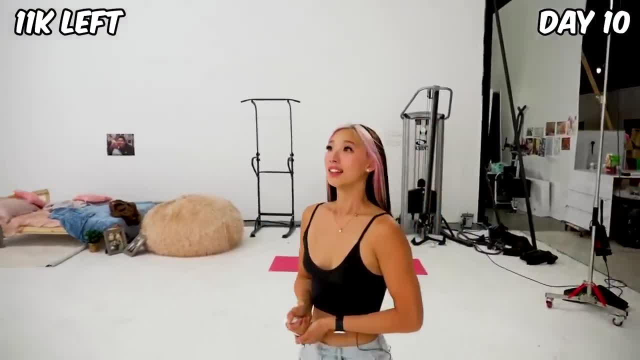 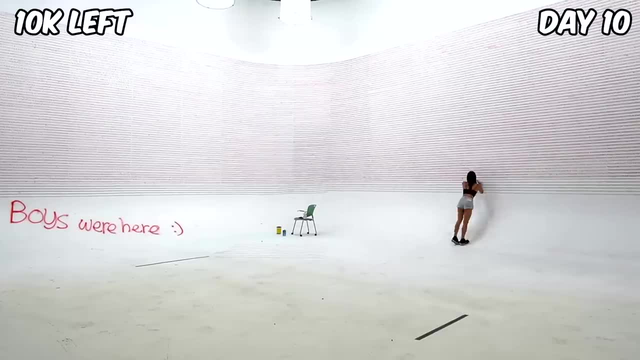 support is the energy I need to help me finish this crazy journey. Looking back on the 100,000 digit math problem, I am so proud of what I've accomplished so far. This is not a good start to day 10.. I made the 48th mistake. 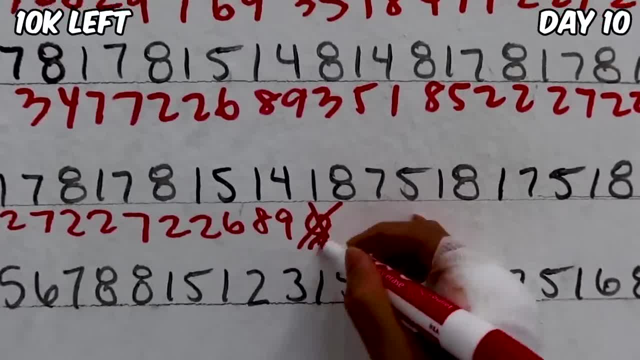 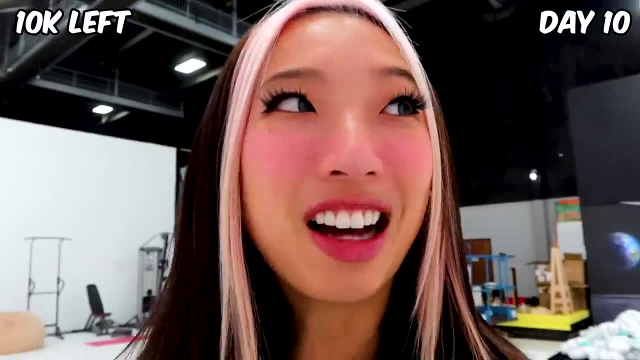 I can only make one more mistake. It's supposed to be a two. I'm literally freaking out. I still have a little over 10,000 to do. I only have eight more hours left. I cannot start over on day 10.. 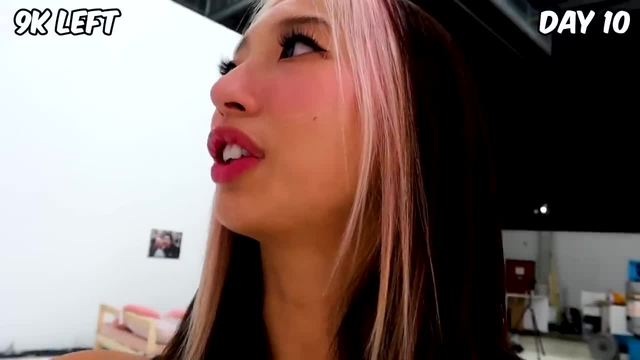 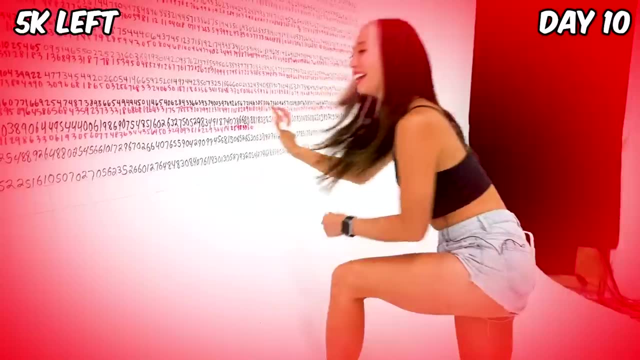 There's no way. There's no way. I'll finish. Come on, Michelle, You can do this. Just a few more digits: Four, nine, five. No, I made another mistake. I'm on the 49th mistake. 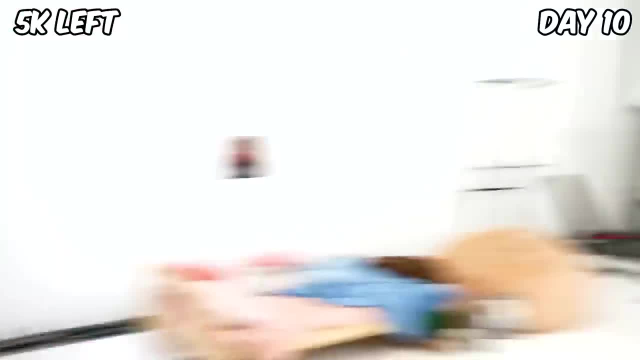 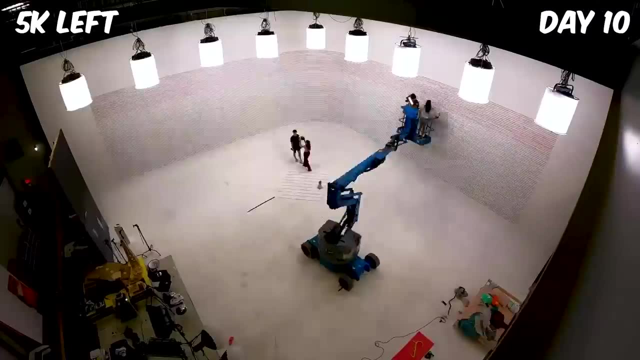 After that mistake I can't make any more. If I make one more mistake, I have to restart the entire problem over, and if that happens I'm not going to finish in 10 days. I just have to make sure that every number I write down from here on out is correct. 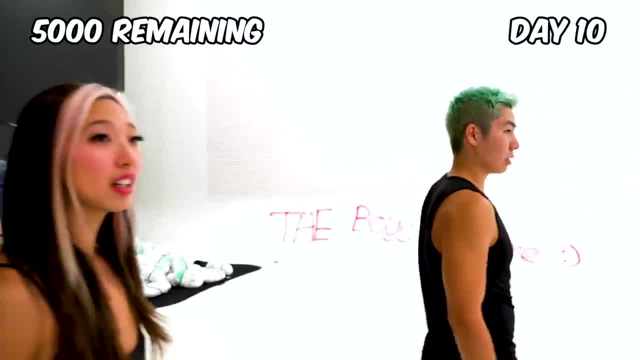 I'm going to have to be extra careful. I still have another 10,000 to do. I still have another 5,000 to go. No way, this is happening. Oh, it looks like it happened. So you've been averaging one mistake every 2,000?. 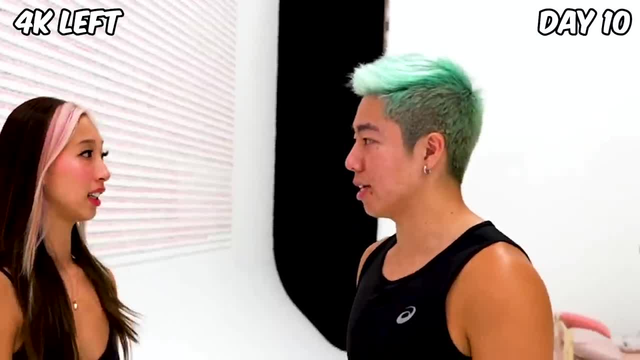 Oh my God, I just can't do math. Hey, I got it correct. Did I just read the human calculator You did. I didn't know what 100,000 divided by 50 was. I knew what it was. 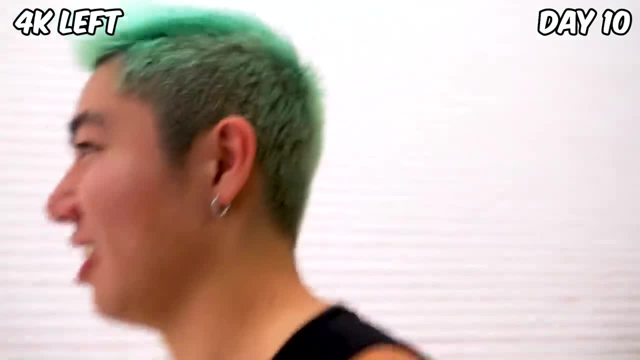 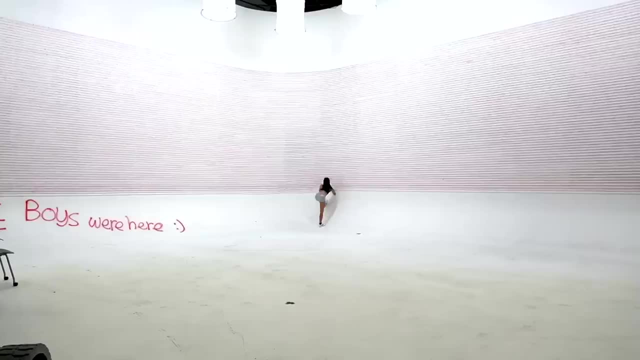 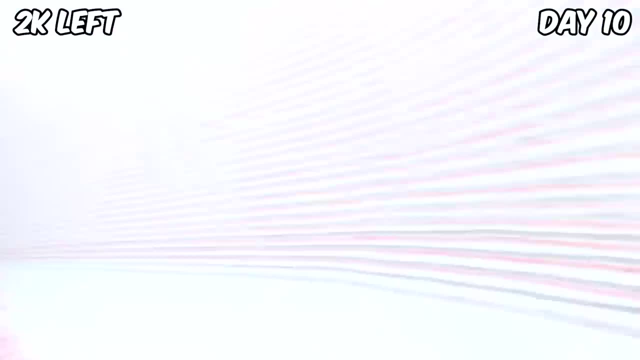 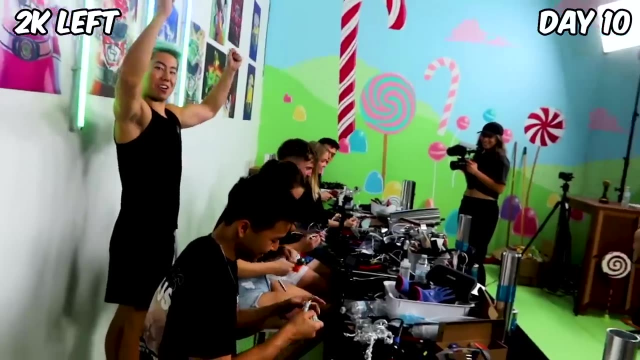 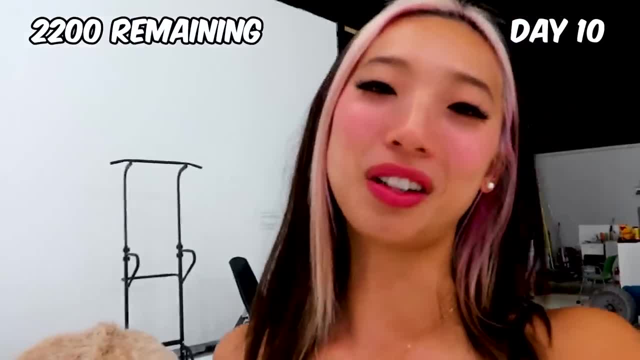 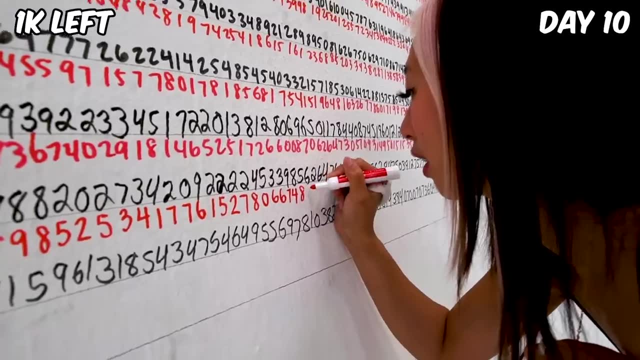 Oh my God, I'm almost there. I also don't want to do this anymore. I've been going super, super slow, so I do not mess up. My hand hurts so bad right now. I can't wait for this to be over. 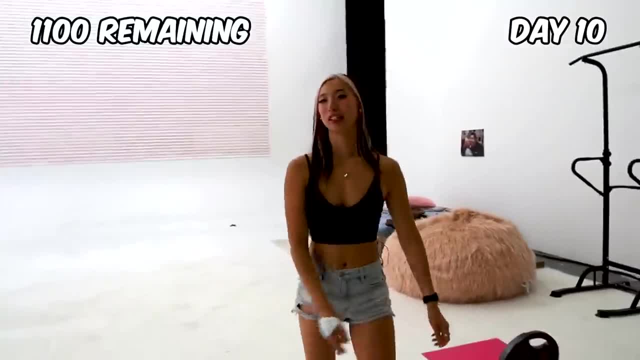 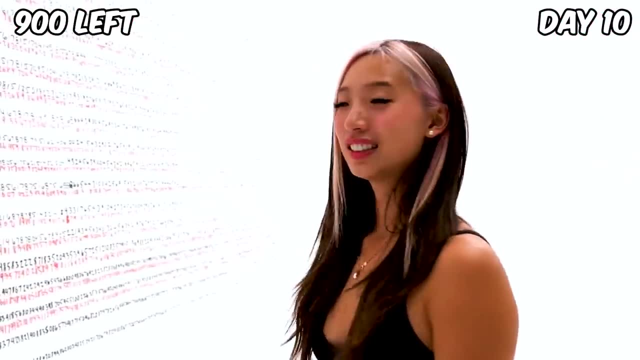 I need a new marker. I think I've gone through about 30 markers. now The last two rows. the numbers are getting better. It's getting really small, Big, small. It's actually a lot harder. These are the longest rows. 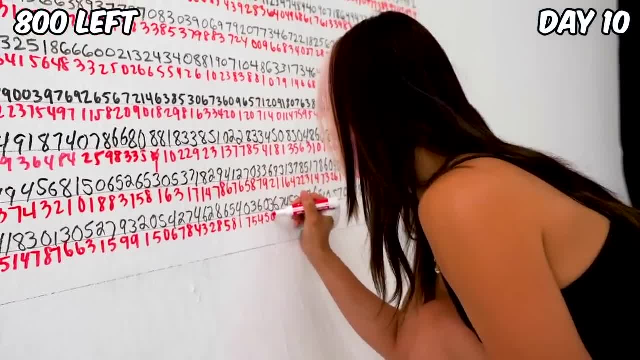 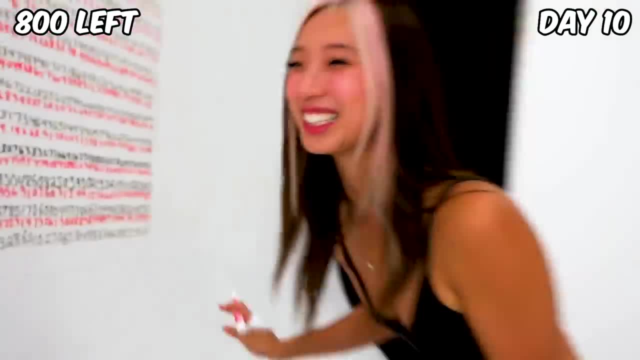 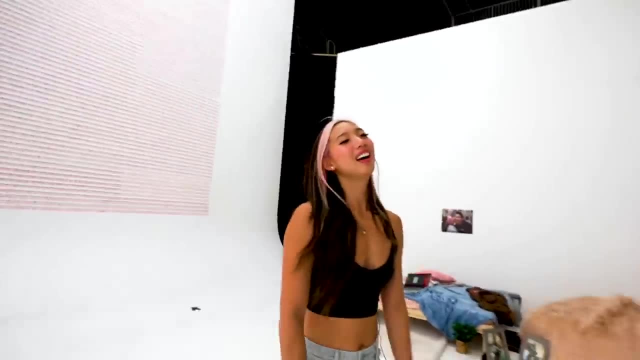 I didn't finish writing it. I didn't make it look big. I didn't make it look big. I'm so worried. Ah, One more row, No more math. The fatigue was really starting to hit, so I really needed to take a break. 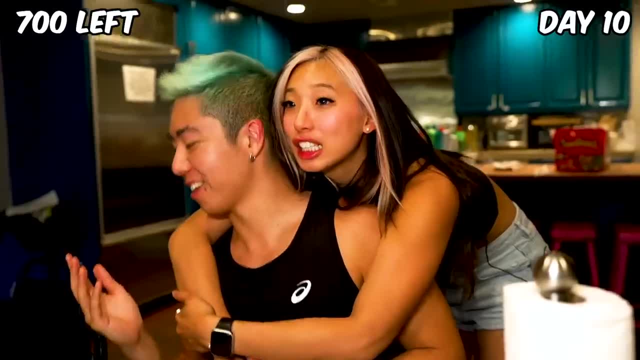 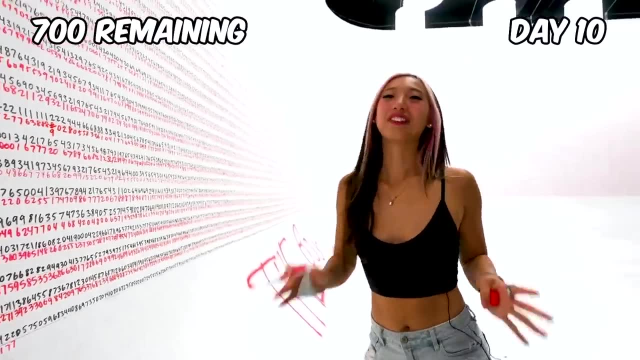 I don't want to keep going. Let it meet me. I need a kiss on it for motivation. I'm ready to go. I can't believe I'm on the last line. I've been waiting for this moment for 10 days now. 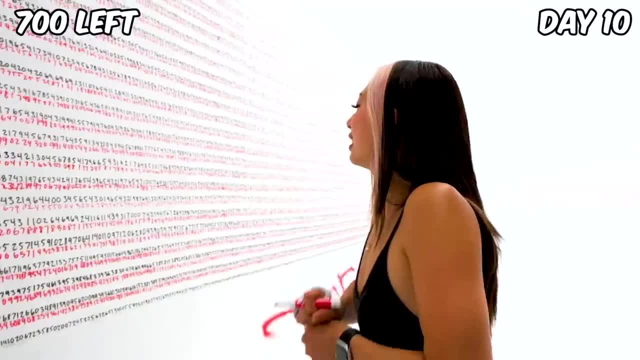 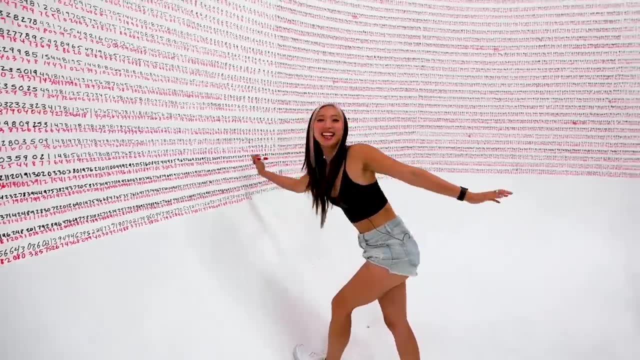 I can't wait to go home. I can't wait to eat. good, I'm just so excited. I just have to be very, very careful not to make any mistakes. All right, guys, I have 100,000!. Guys, can we just take a moment to take this in? 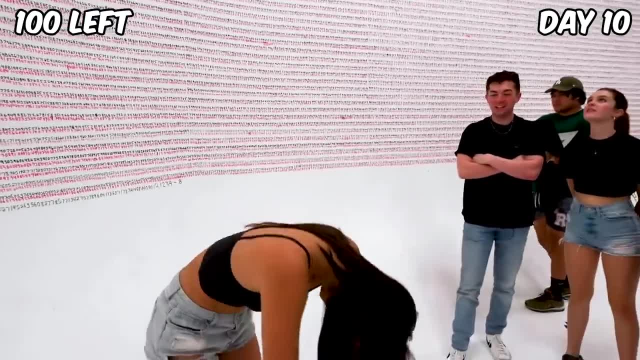 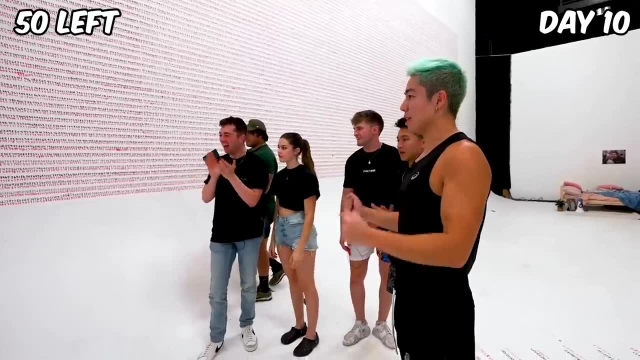 Like how insane. 100,000 is So crazy, Michelle. How else is this even possible? All right, guys, cheer me on. We got to go Munchy. Michelle, Michelle, Michelle, Michelle. Subscribe before Michelle finishes.